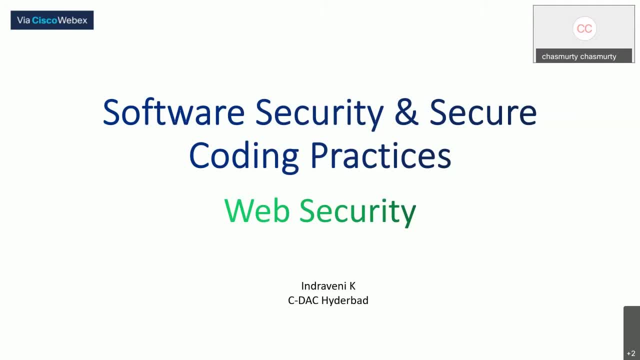 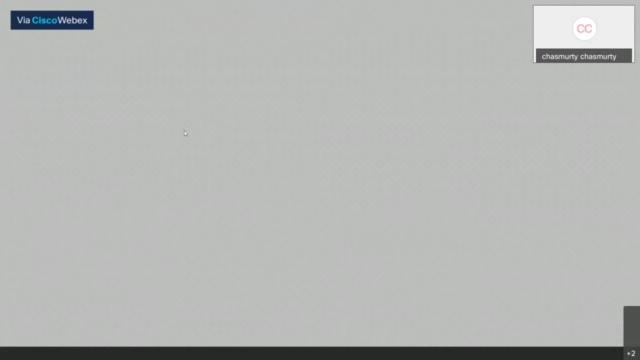 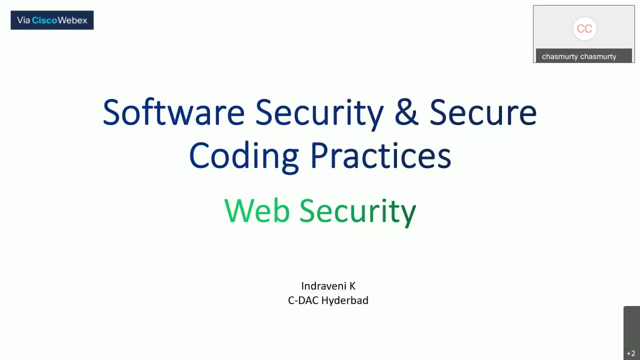 you, you, you, you, you, you you. very good morning to everyone. welcome to the session on web security. the speaker of today's session is miss indraveni. she is currently working as a joint director at cdac hyderabad. she has 15 years of experience and has achieved expertise in web technologies. 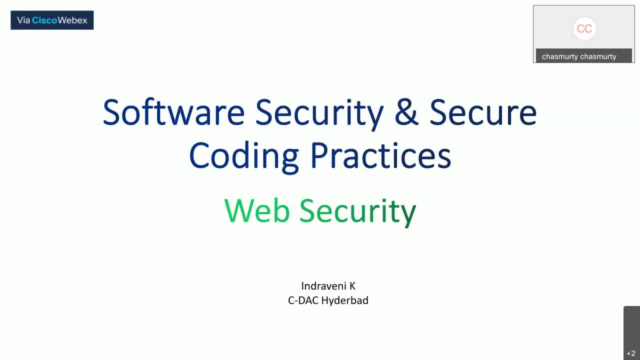 web designing and development, web administration, web security, vulnerability assessment and penetration testing, information security, open source software and cloud computing. she's a skilled security auditor and tester. she has published research papers in various conferences and delivered talks. she has been a keynote speaker in various cyber security conferences. she is actively involved in 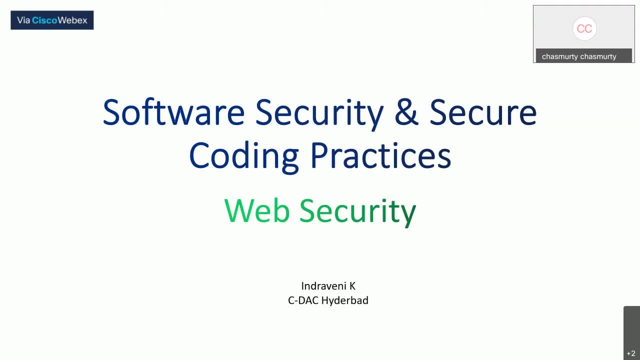 development of boss, gnu, linux and online and indian version of linux operating system. she has conducted more than 300 security awareness workshops across the country. she has many certifications- certified isms, iscis, computer forensics in orlando, florida. she is a sans trained in. 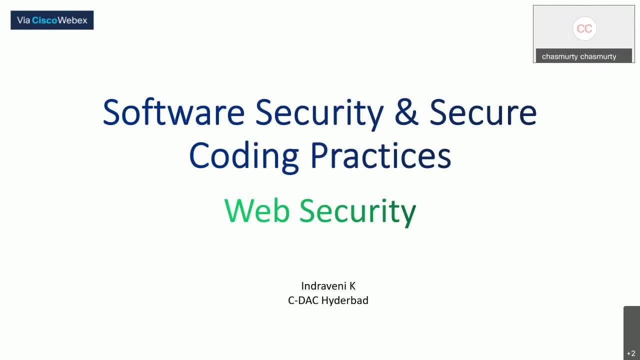 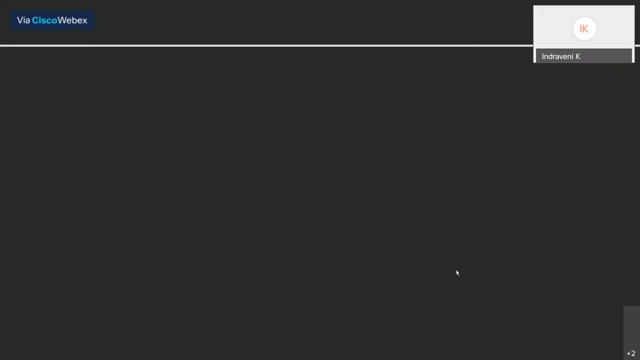 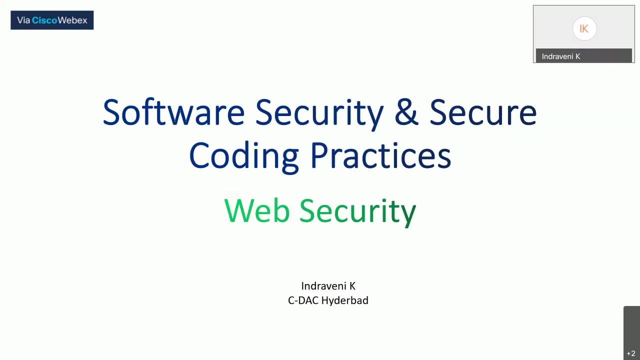 integration testing and it's still gi. web application penetration tests, gwapt, samson being certified in website quality, sdqc, effective faculty development by iu, cee and info. thank you, cheers, hello, see me, Hello, Hello, Hello, Hello. Actually your voice broke in the middle. 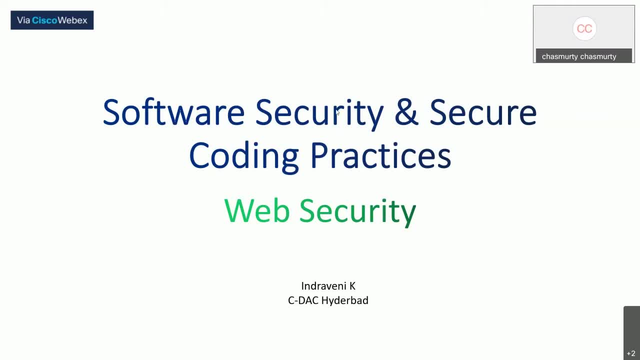 Okay, okay, We still have time, so can you please repeat the introduction? Yes, sure You want me to repeat now. Yeah, yeah, please, Can you do that? Yeah, Good morning everyone. Welcome to the session on web security. 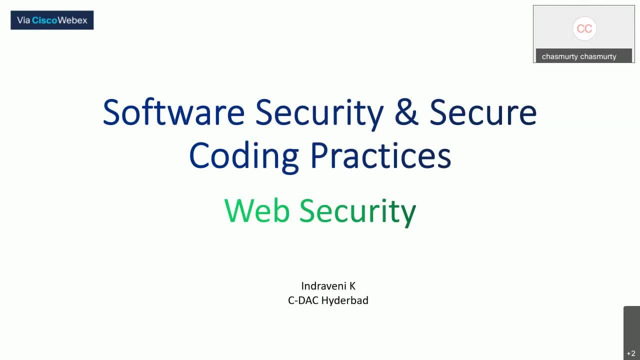 Ms Indraveni is the speaker for today. She is the Joint Director at SIDAC Hyderabad and she has 15 years of experience and achieved expertise in web technologies, web designing and development, web administration, web security, vulnerability assessment and penetration testing. 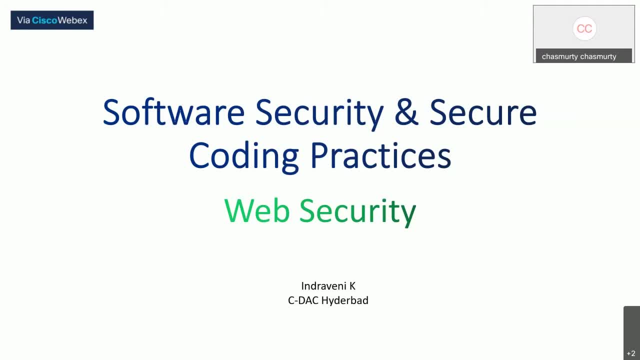 She has been a keynote speaker in various cybersecurity conferences and she is actively involved in development of BOSS GNU Linux, an Indian version of Linux operating system. She has conducted more than 300 conferences and she has been a keynote speaker in various security awareness workshops across the country. 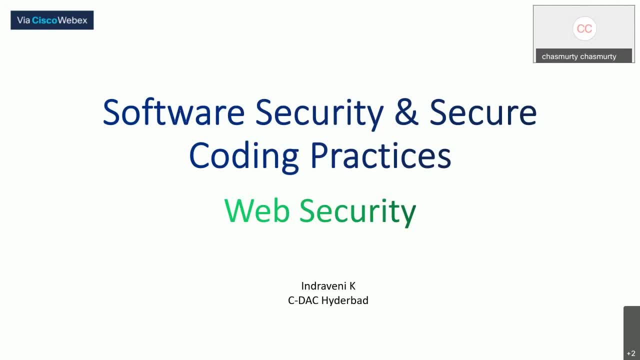 She has many certifications to her credit, which include Certified ISMS Lead Auditor, IACIS trained in Internet Forensic Investigations and Applied Computer Forensics in Orlando, Florida, during April 2016.. She is SANS trained in Advanced Web Application Penetration Testing and Ethical Hacking. 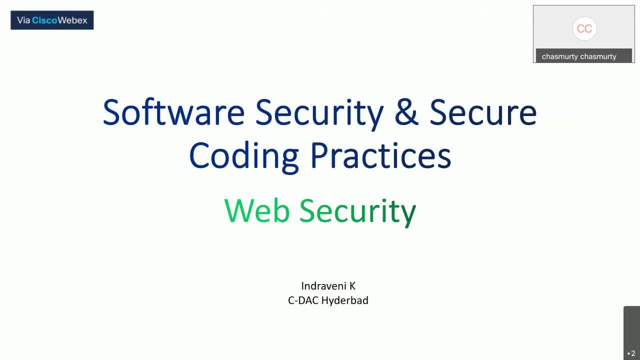 She has GIAS SANS certified 07. Web Application Penetration Testing and Ethical Hacking. GWAPT SANS Certification. She is certified in WEBS website quality assurance and certification by STQC. She is Certified on Effective Teaching, Cooperative Learning, Effective Faculty Development. 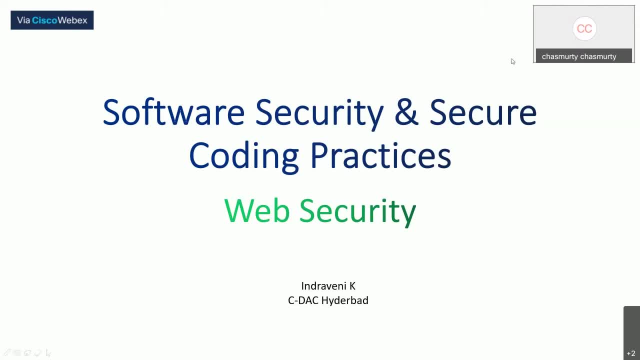 Outcomes-based Education by IUCEE at Infosys Mysore. She is Certified on Ruby on Rails programming language by CICC and Confusio Japan in Tokyo. Thank you, ma'am, for being here. May I now request you to take over the session? 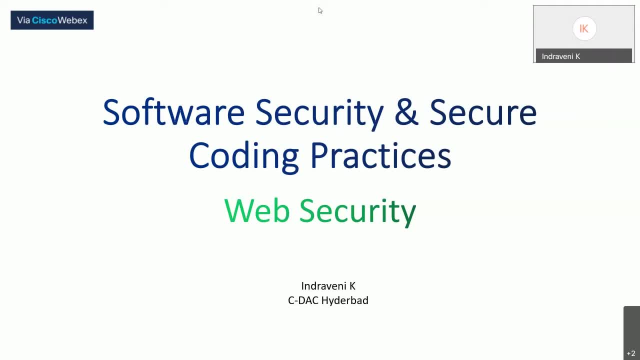 Yeah, thank you, ma'am. Very good morning to everybody. So today in the series of sessions on software security and secure code practices, we are discussing today about web security. I hope I am audible. Yes, sir, can you please acknowledge? Yes, yes, yes, sorry. 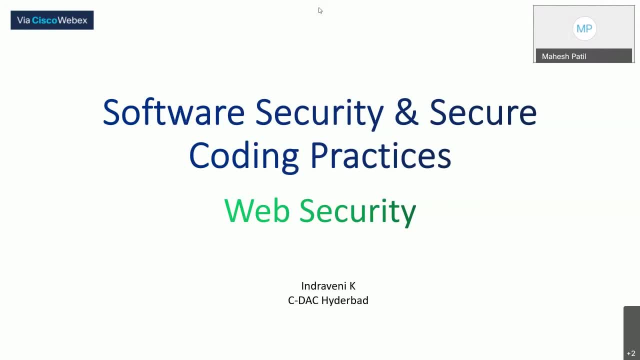 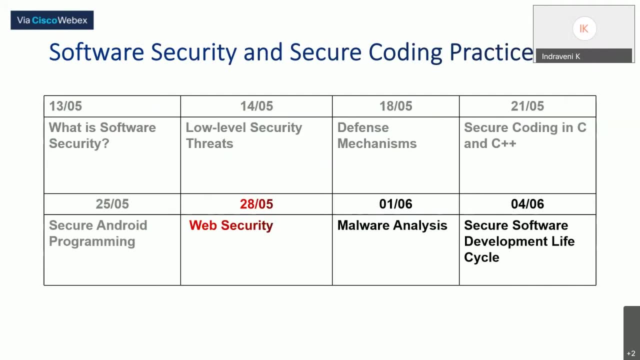 Okay, thank you, sir. Yeah, so we'll start with today's session on web security. So we have already covered with five sessions under this topic, and today we are on the sixth session of security, followed by you have two more sessions in the same concept, basically. 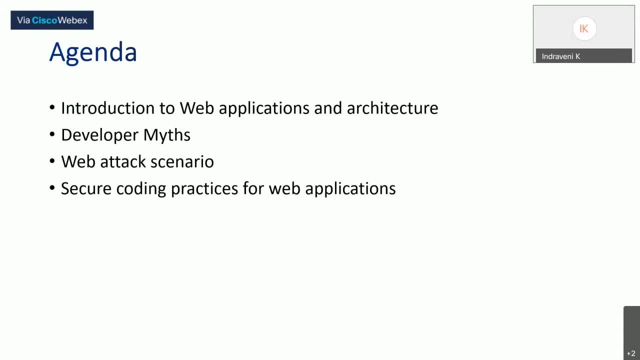 So in web security today, our main objective to be covered in this session is something like this: I will try to introduce you to web applications and some web-based architectures and then we'll discuss upon the developer mics how the developer usually does the programming and what could be the impact of those activities. 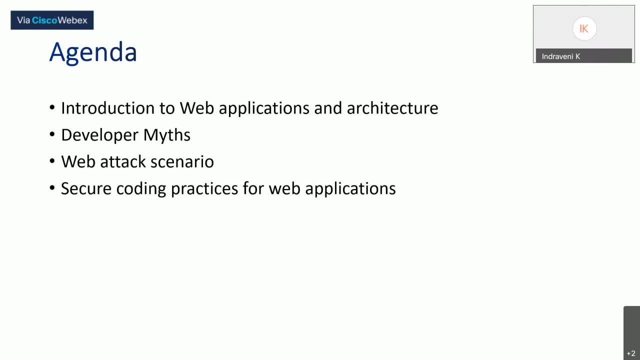 Then we'll see certain web attack scenarios and we'll then relate to the secure coding practices with these web attacks- Certain web attacks. we can't cover all the web attacks. However, we'll try to look into certain key web attacks and what secure coding practices we should follow. 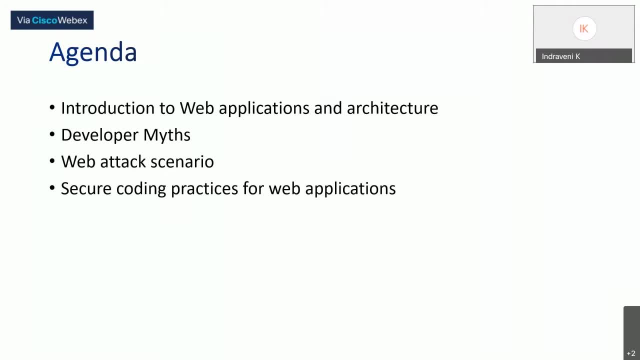 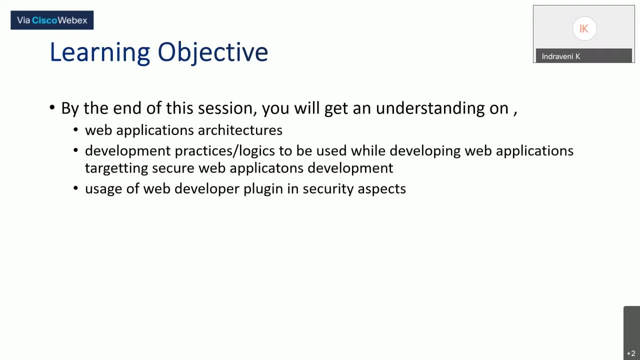 to protect our application from the web-based attacks. So this would be our agenda for today's session, And so by the end of this particular session, you will be able to understand and get a good picture on web application and architectures. You will be able to get development practices, some guidance. 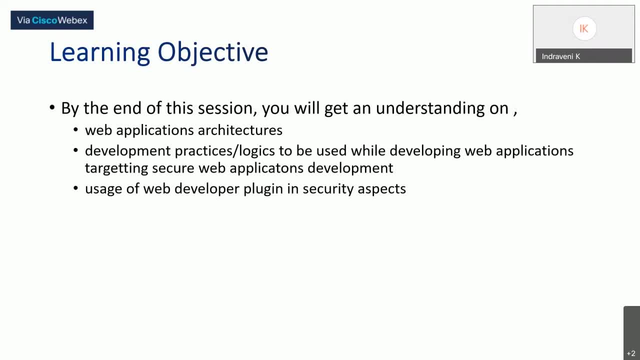 you'll get in development practices or logics- how you have to put your practice implement, what kind of logic you should implement While developing your applications so that your application would be secure enough, And you'll also have tried to understand certain plugins, basically how to use those. 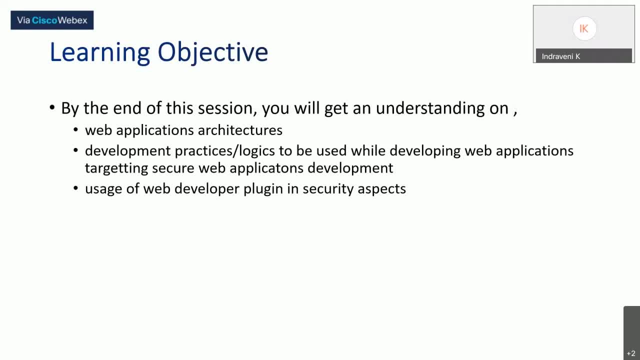 plugins in terms of security aspects. So this will be our learning objective By the end of the session. you will understand this. So, since our previous, all our previous topics are related to more on to the Android, Siri and all and this in between, the session is talking about this. 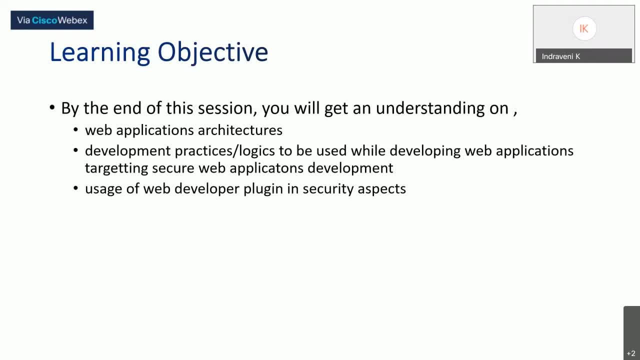 and i believe that most of you are students who are already doing some kind of programming in your colleges. you must be having programming web-based programming languages like java, php, python kind of things, and so this concept you'll have to consider related to those web-based programming languages. 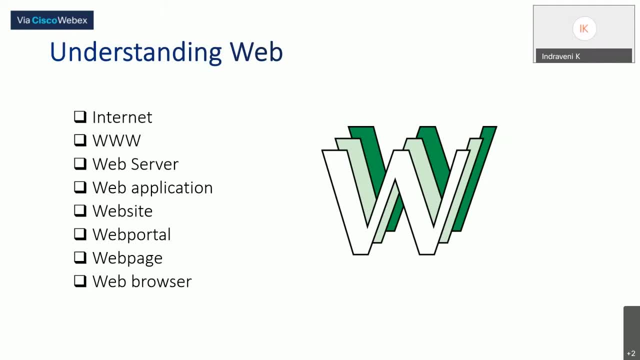 whenever you're developing a web-based solution or applications. so yeah, before we go into technically in depth, we'll just try to have some understanding on these words, understanding the web. basically, in web we have so many words that come across towards internet, www, that is nothing but the worldwide web. we do hear a lot of times website, web application, web portal, web page, so all. 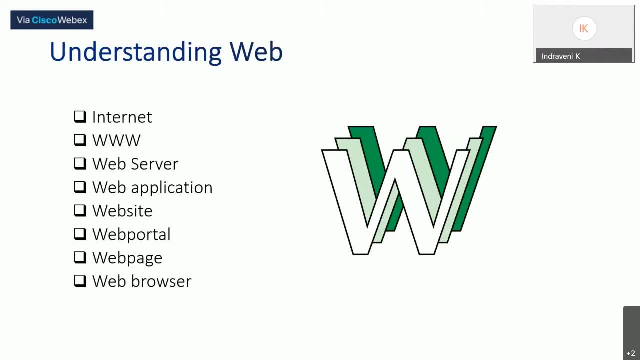 of these seems to be more or less they are same. the way they are bit called it depends on each individual and certainly when it is very dynamic in nature, it's usually called as the web applications. otherwise, a website, a web application, can also be called as a site. it can also have so many web pages into it, and so on. 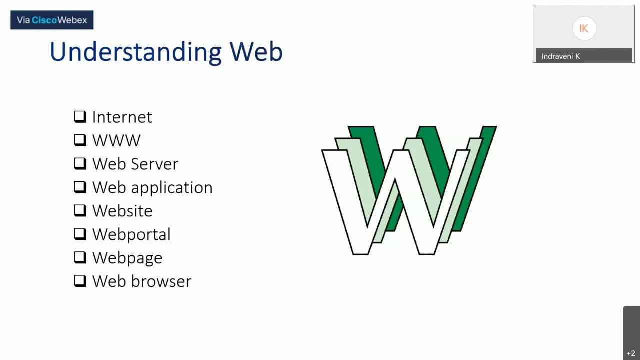 and in relation to all of these web-based applications, we would have a web server, which is required usually for hosting all of the applications. and, yeah, to access all these applications we need a web browser. so these are some key wordings that usually come across whenever we talk about the. 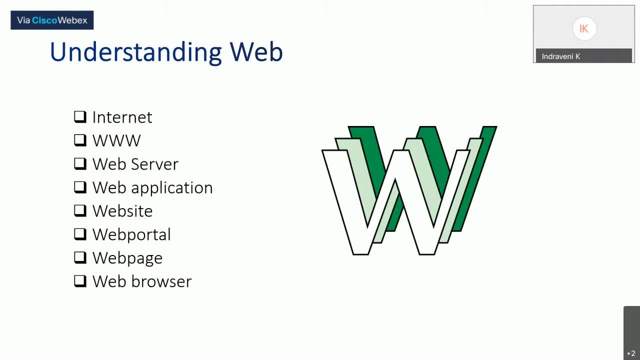 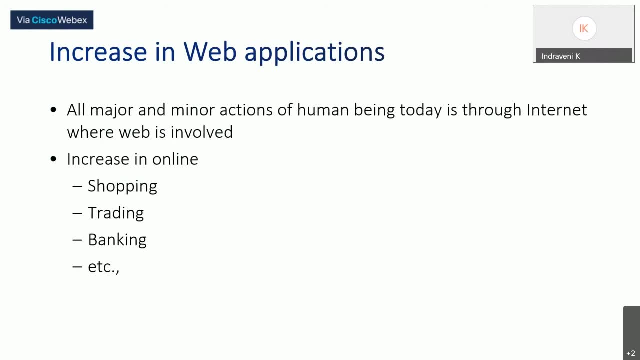 internet or a worldwide, so we'll see and understand, uh, the concept. so why are we so much concerned? because there is a huge increase in the web applications. all major and minor actions today we are doing on the web, and that, too, over mobile as well as on the same laptops or systems. 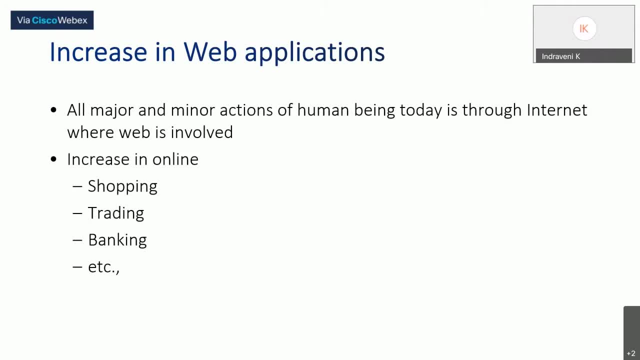 so increase. there is a lot of increase. since there is a usage has increased, the need for developing different applications also increased and today we are in a state that any website that we come across, the equivalent mobile application is also expected by the public because of its easiness. so there is a lot of growth in the web applications. equally, there 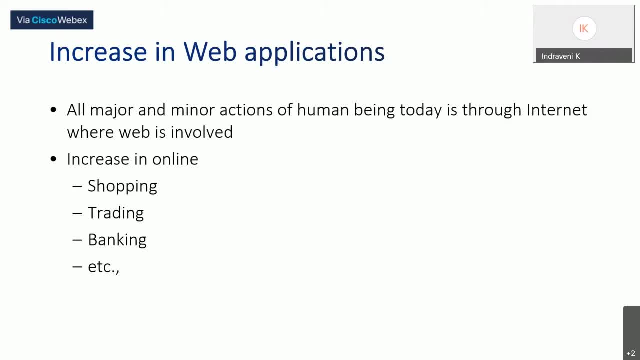 is huge growth in the mobile applications to equally compete the requirement of the web applications. so because of this increase there is increase, since the increase of development is increased, usage increased and so the development requirement also increased and so the attack on the web applications changed and hopefully we are not just beginning to target applications. 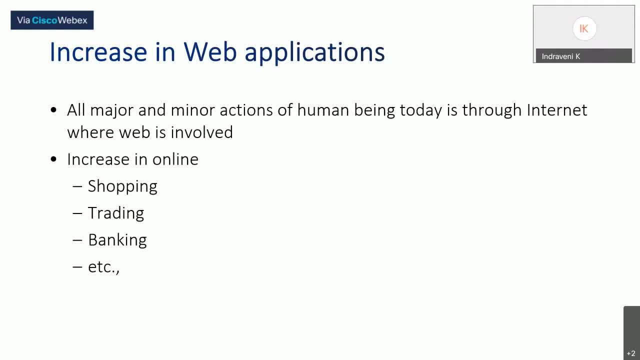 of anything on the internet. so those are just like the wholeiş. you also have a responsibility to the start cause. you are the ones who're tackling the development of the operations. to plan your challenges, uh, even if you think about, uh, you could take a web browser andablo. 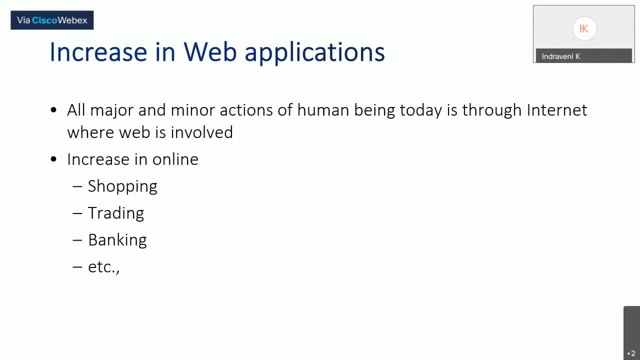 and also target um, industrial administrators with digo, the public, the common man, to perform various attacks through these applications. and, yeah, the same web applications are also helpful for the attackers to attack the organizations, the one which where the applications are deployed. and to you all, being engineering students or programmers, upcoming programmers or experienced programmers, you all have a responsibility of developing. 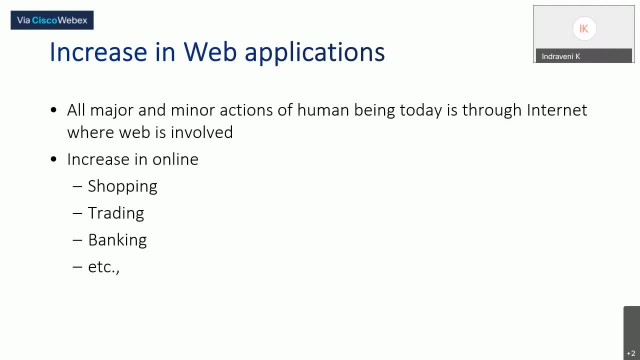 may be doing a big, big government projects. you may be doing international projects which involve a lot of web-based solutions or applications. so if we do not introduce security practices into those applications, it can lead into various attacks and which can actually result into loss of a lot of data and all of these things. 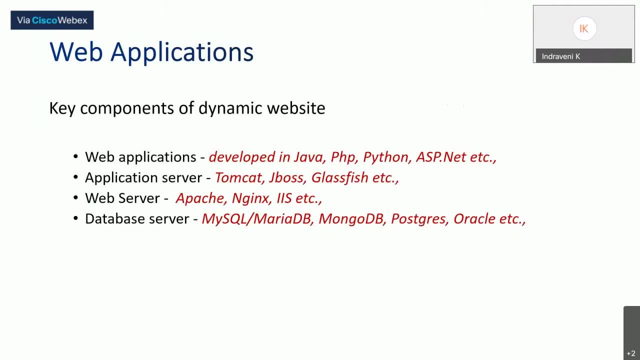 right. so that's the reason we are trying to today understand security practices into web applications. so certain key components in any dynamic website. if you pick up any kind of a website, usually you see that there would be a web application which is usually developed. this is the one which we develop using programming languages like java, php, python. 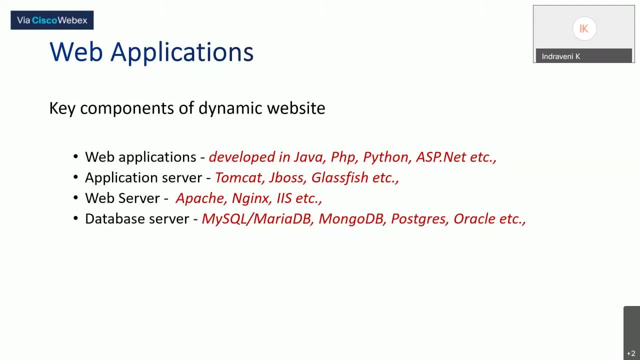 there are so many programming languages, so any of the programming we use, either we use programmings or we directly use the frameworks. through these programmings are used or developed. the frameworks also can be used by many people. many people use content management systems, and all to develop the applications or to host a particular website. 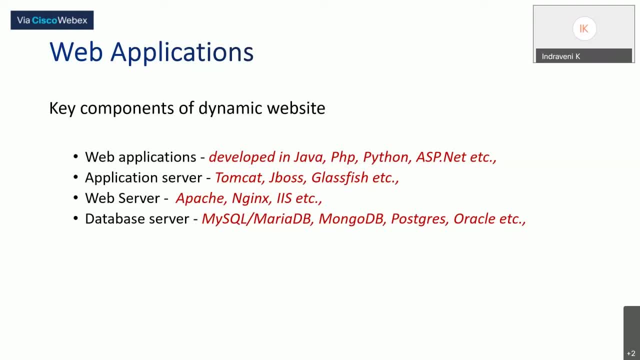 another key component that is usually used for hosting any dynamic website is there would be an application server. application server is a server which is usually used for executing the programming, the application which you are developing, usually the tomcat jboss. all of these are known to be the 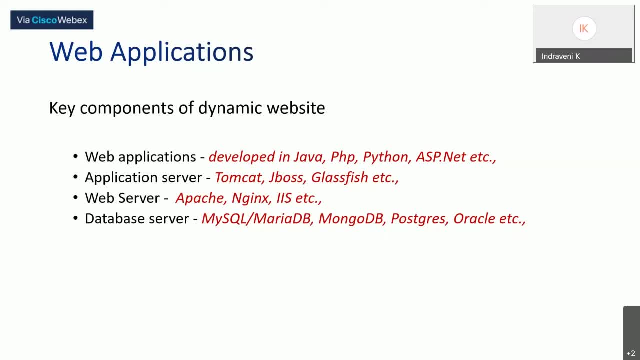 application servers. now, apart from application server, there is also called as a website. actually, application server also supports hosting the websites, but considering the security point of view as well as the performance wise, it's not recommended for the public to host one of services. so a web server is being placed in between, through which web server itself communicates with application. 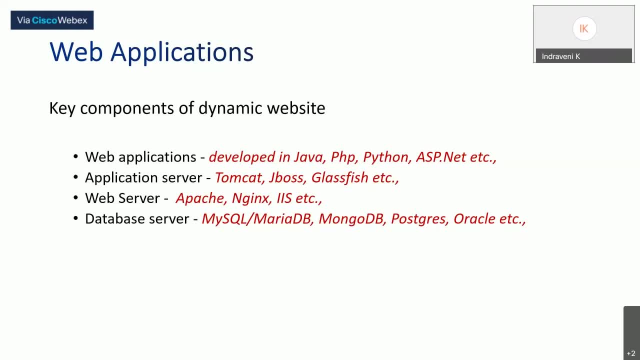 server to launch the application and there would be a database server. so these are some key components that you usually see in the dynamic websites. so these are the key components that you usually see in the dynamic websites and their examples are given us over there. so this is the same architecture of the 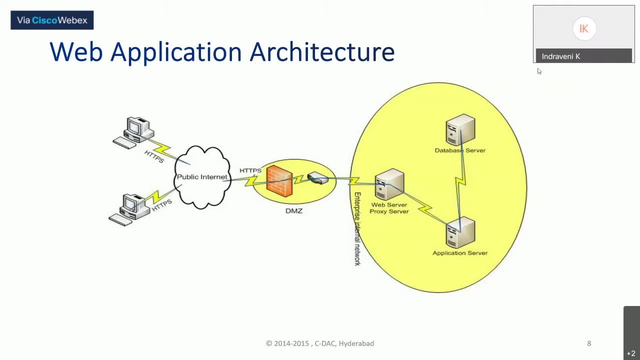 applications, web applications. so usually what happens is from the public. there would be a https or it can be http based interest coming from a public network to your dmz. dmz is generally a demerit zone, nothing but those data center or an environment where the actual websites 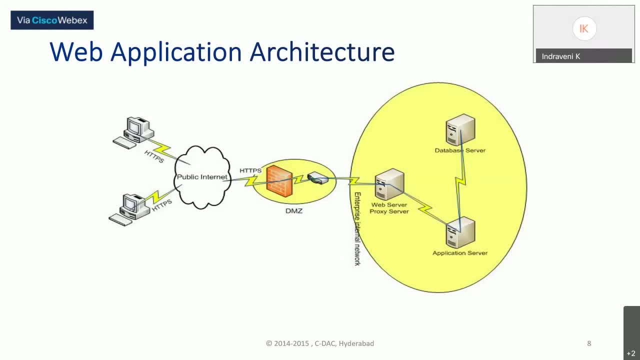 are, servers are posted, are running. so in the dmz there would be a lot of perimeter security devices like firewalls, routers and all these things. so, crossing all of these things, the https request from the public reaches to your server, the server, nothing but the web server, which is 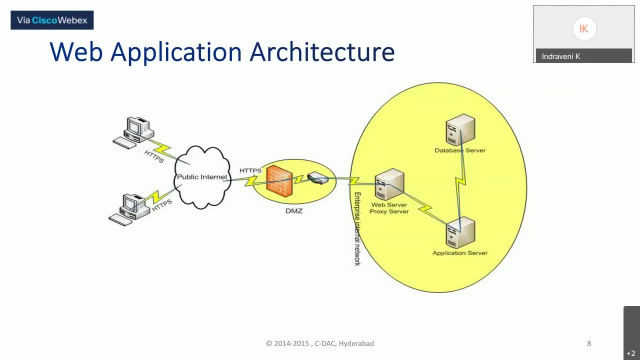 actually the front end for your actual application. so now from the web server, the content can go and hit the application servers and application server processes. your request gives the response. if there is any requirement of fetching something from the database, it does. the communication with the database server also. so this is a typical architecture of any web-based application. 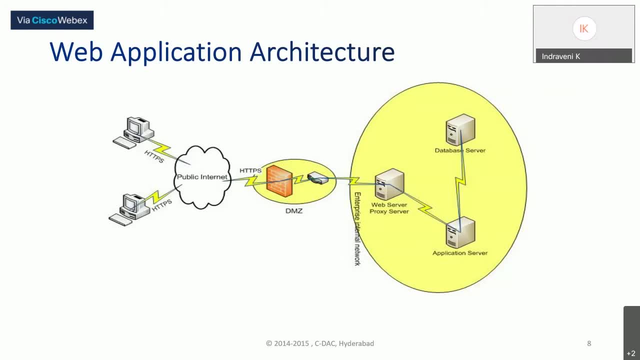 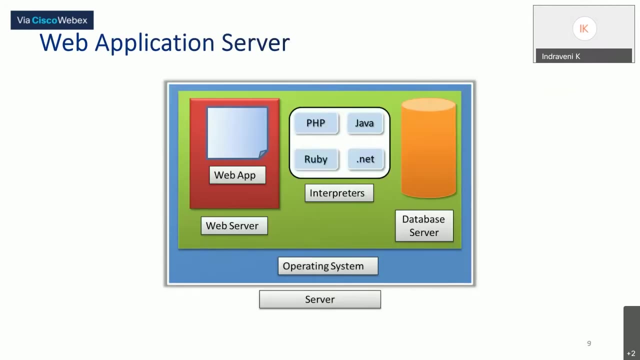 so you will have components like the web server and application server and the database service. so what? the key logic for all the security practices that we will be discussing would lie for the application server solution. so, and when you say web, application server, you will have all of these components into it. generally, you will have a web server, so these: 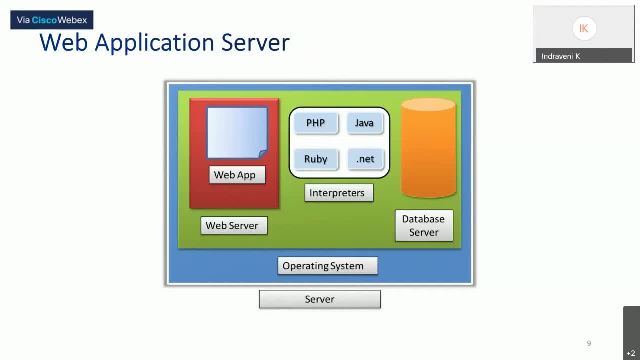 words application server and web servers are mostly those interchangeable, but technically, when you go at the implementation level, there's a slight difference among them. so there's always a server, web server and application server underneath which you will have your actual application which has been developed. so there's an interpreter view of your programming language. 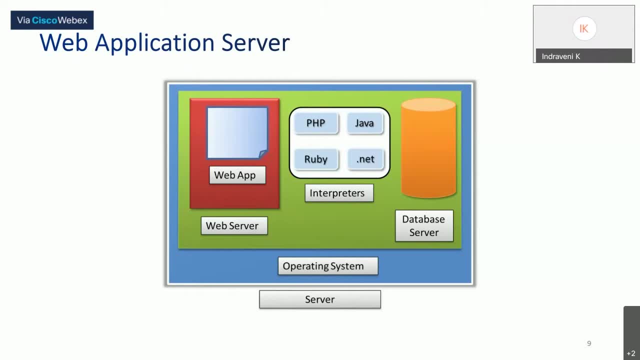 which actually tries to process your uh, your compile your program, run your program, and then gives the response to the end users. and here there's a database server on. all of them are been installed on an operating system which is actually lying on a server. so this is the. 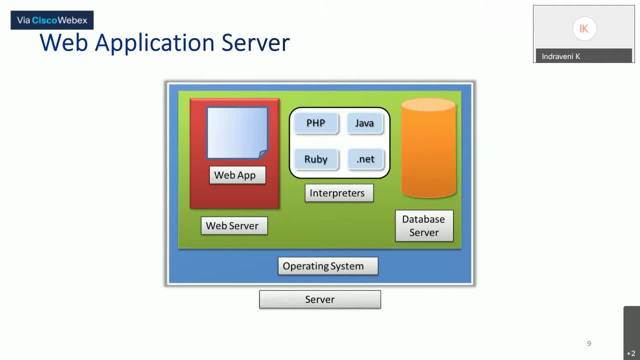 typical components of what all are part of your web application servers. now coming to your client: now, when we are saying that there is a request coming from the public, so request is coming from public is from where it's coming from a client, so the client is nothing but the web browser, generally a web browser. 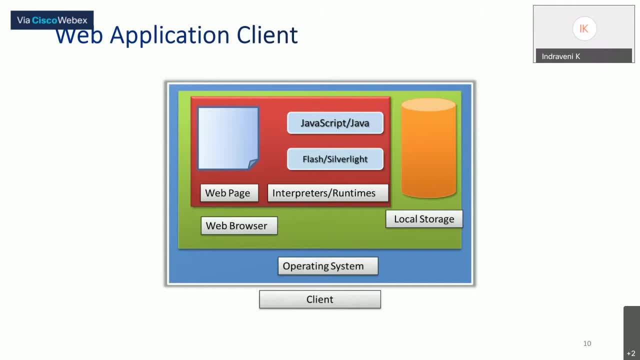 is being considered to be a web application client which actually interacts with your web application server. so the client: yes, there would be an operating system on top of which you'll have your so many applications running in your systems. one of them are is the web browser. so through this, 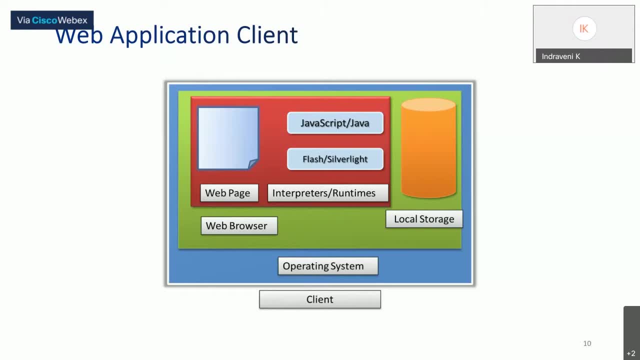 web browser only. we try to interact or access any kind of a website which is there in the worldwide: the web page. the browser has some more responsibilities of running certain browser-based modes, whichever is available. Whenever there is a response coming from the servers, usually the browser. 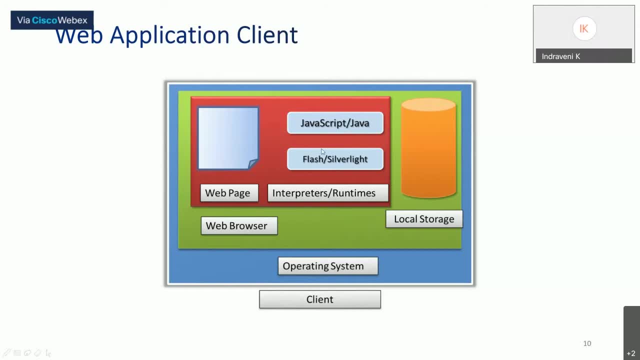 has a responsibility of executing those codes and showing them. something like JavaScript is visible, the browser executes the JavaScript and shows you the results, similarly a flashlight or server-like kind of programming it executes And within the browser also there is a storage, Like we have seen in a server, in an application server. you have a database server over here. 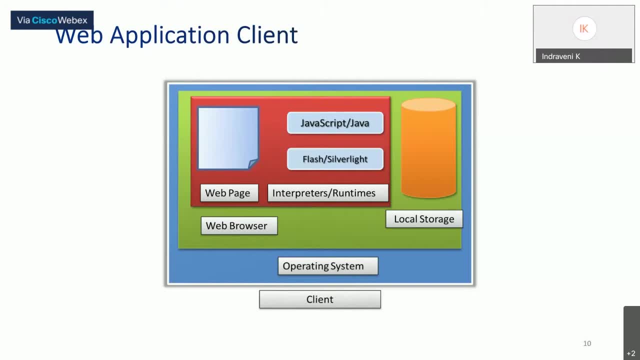 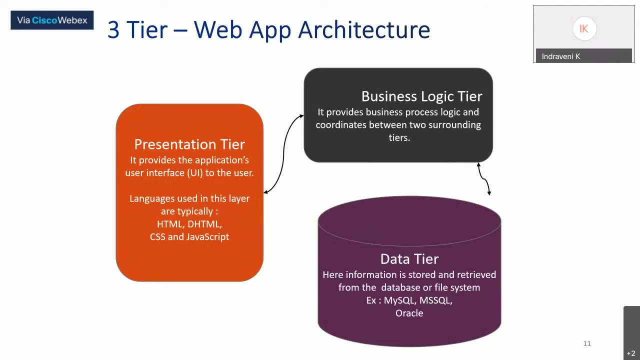 Similarly, in your browsers also, there is a local storage available And many of the developers tend to use this local storage also for storing certain information, some temporary information, in browsers. So generally this kind of a communication between these database servers, application servers and all is usually known to be as a three-type. 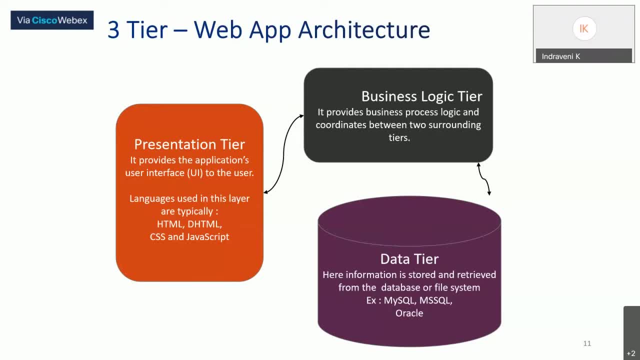 web-based architecture. Three tier is one tier. first tier is the presentation tier, which is usually the user interface which is provided for the users. Typically, you develop this using whatever you are developing on HTML, DHTML, CSS, JavaScript, all of them. 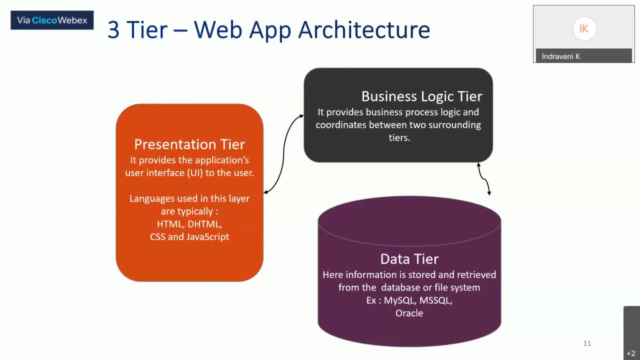 belongs to the presentation layer. Then comes the business logic tier, where actually your business logic is being processed. That is, the application is trying to take the request from the browser. that is nothing but the common client. Like, let's say, you have a 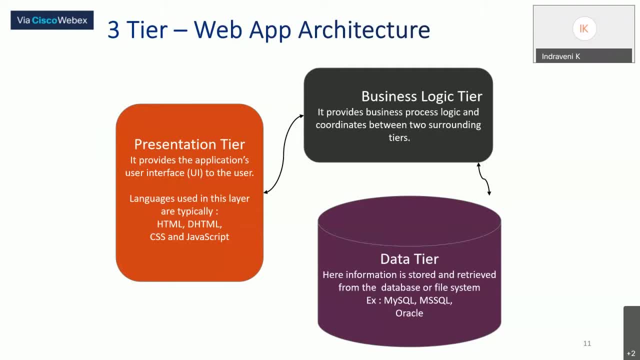 user. if somebody is typing a username and password, there's a front-end which is actually giving a. that is a presentation layer where you can see a form with a username password to be put in the form. That request is being sent to your server, where the business logic. 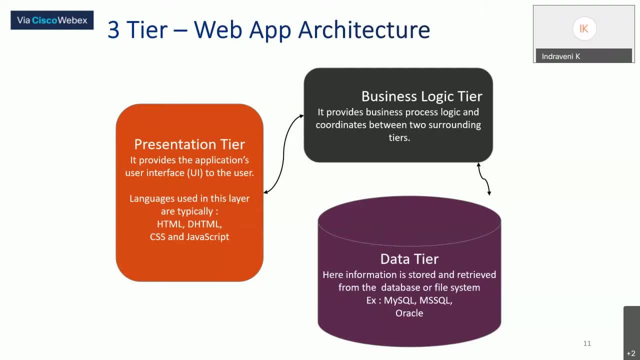 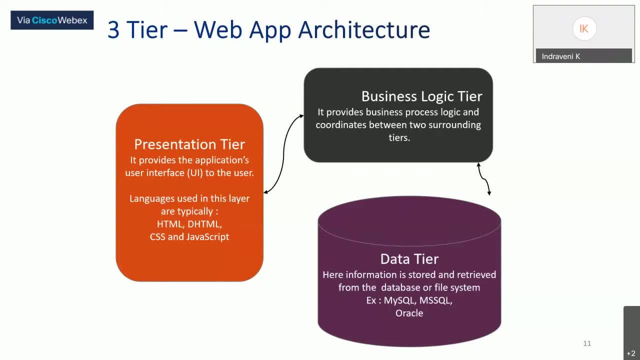 let us see So generally. this is a three-tiered web app architectures, So many people host either all of them in the same server. many hosted them in different different servers, Database servers. people host different servers also, So these are certain terminologies. 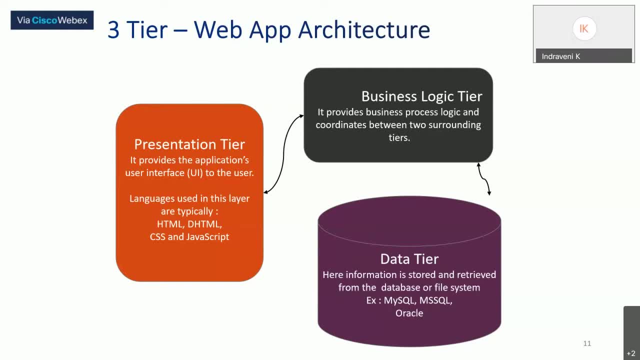 that, before we go ahead with actual security concepts, I would like to introduce you to how a web-based application usually works. So when we say a client, remember it to be a browser, And when there's a server, we are talking about. is that when you say a client, you're talking about a server, and when there's a server server, you're talking about a web app, and when there's a server, you're talking about a database server. So when we say a client, remember it to be a browser, And when there's 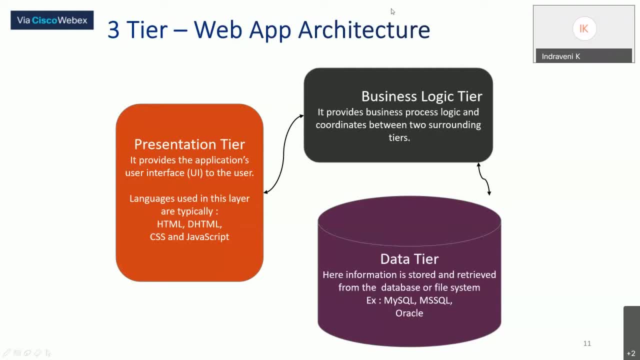 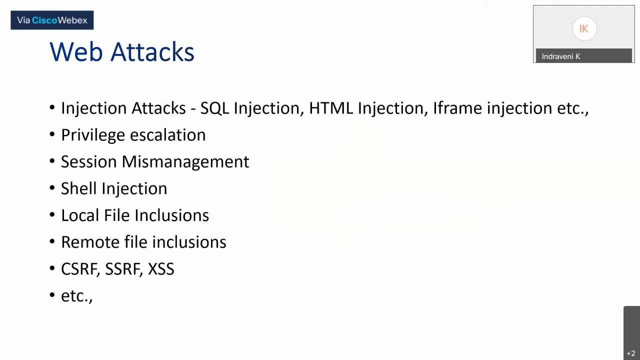 are talking about a application, whichever is running on the server specifically. so so, moving towards our web attacks, basically you must be heard about many of the attacks. there are so many web application attacks. few of them. i just listed out over here to just give a look to you that what kind of attacks are usually being targeted on the web applications first, 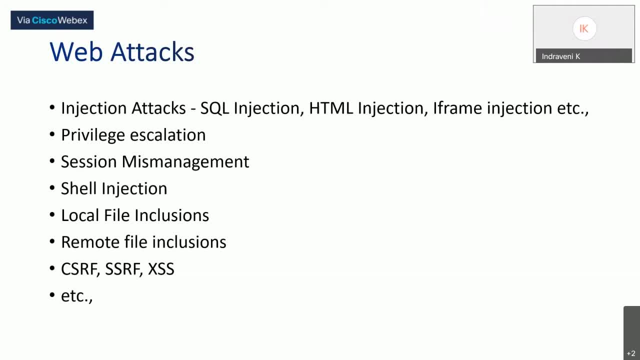 and foremost and most famous attacks are the injection attacks. injection attack is something which is like somebody- somebody tried to introduce some malicious or unnecessary content to your site, which can lead to different attacks like SQL injections. it can be an html injection and then iframe injections and so on. if there is no session management, proper session manager, 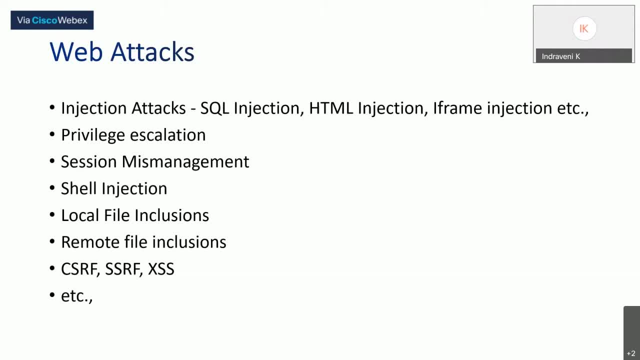 there is chance of performing the privilege escalation kind of attacks, sessions related attacks like session fixation, session hijacking, etc. then there could be local file inclusion, cell injections, cross-site request forgery, cross-site scripting attacks. there are so many web-based attacks, but since this particular topic we are discussing about the SQL coding practices. 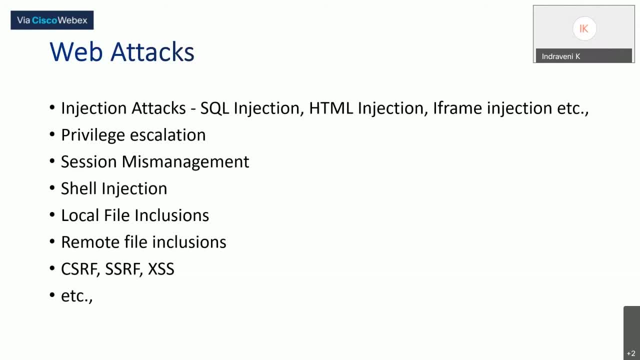 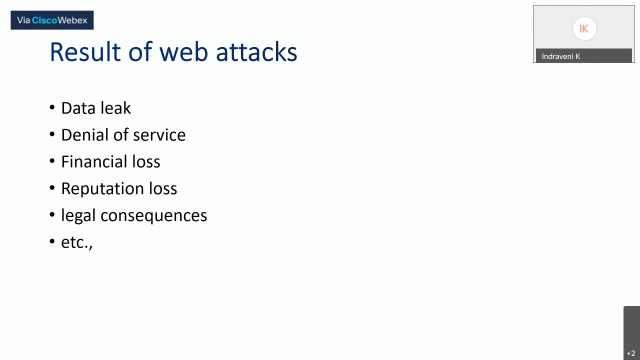 we are not highlighting anything on these web attacks, like how this attack happens. how this attack happens is a different context, but our point is: what do i do to protect my application from these designs? okay, so we would be discussing on the– how do I do to stop these? 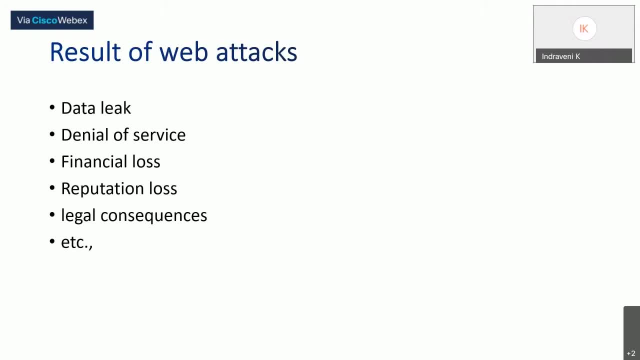 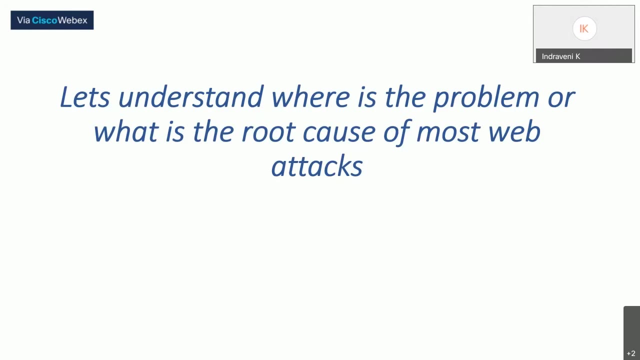 because it deals with lots of users- personal data also. many more can happen. so these are certain impacts of web-based attacks that can have that happens on the service. so, with this understanding on the architecture and attacks that are coming onto the system specifically, so why these attacks are coming into, what is the root cause of these web attacks? 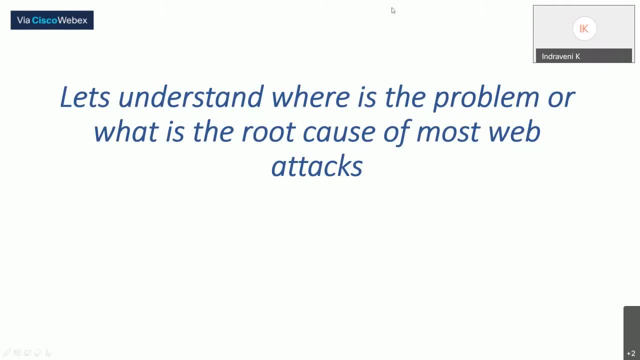 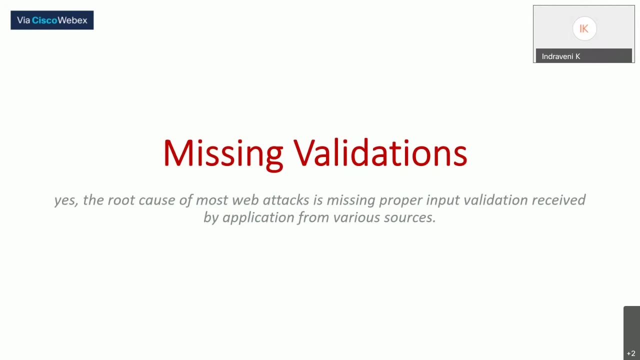 why these web attacks are actually happening. more majorly so, missing validations, the major reason for these web attacks being successful. the root cause behind the web attacks is validation, non-availability of validations and this very validations- i am not talking about only the input field validation- have plus. 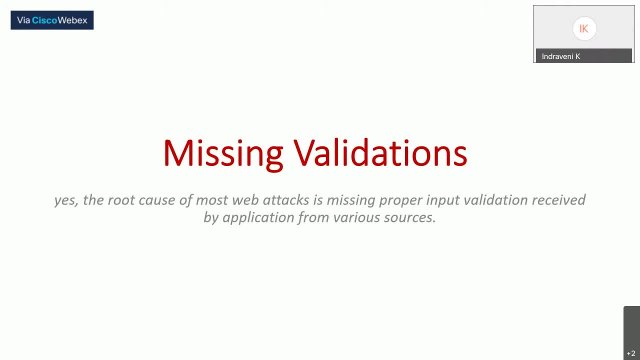 validation. you can save for anything that data that is coming from any source. it can be validation of session also. it can be validation of the file also. everything is finally. the result is there is no validation of something due to which some attack is happening, one of those attacks which we listed over in the previous slides. 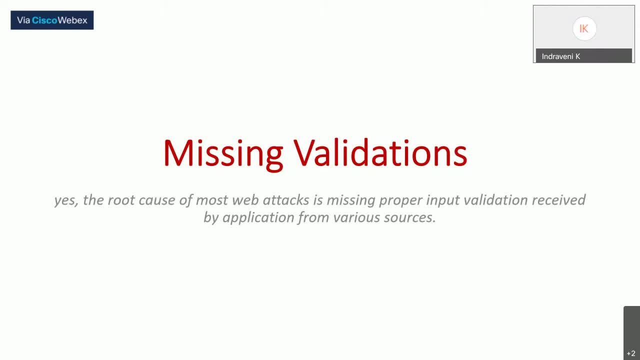 so why validations is missing? do you think that you are not doing validations? i'm sure all of you must be definitely writing a program and you are definitely writing your program in such a way that you do not accept a whole number in a name field or an email address with a value a. definitely not. you are all good programmers. learn good. 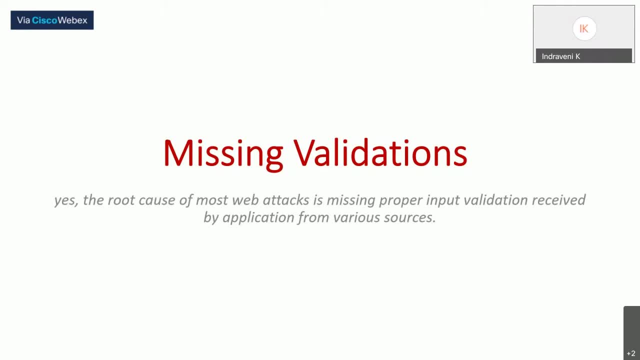 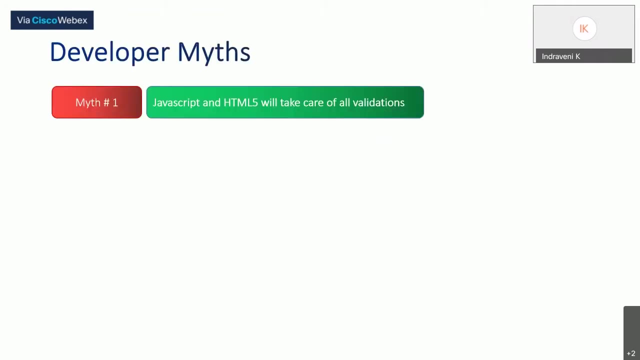 programming language. you have developed so many projects in your colleges and all so as per the things being taught in your college. definitely, you will implement validations, but there is something that is missing over here: what validations we are doing, where are we doing, is what that's mattering over here. so let us understand from developers point. 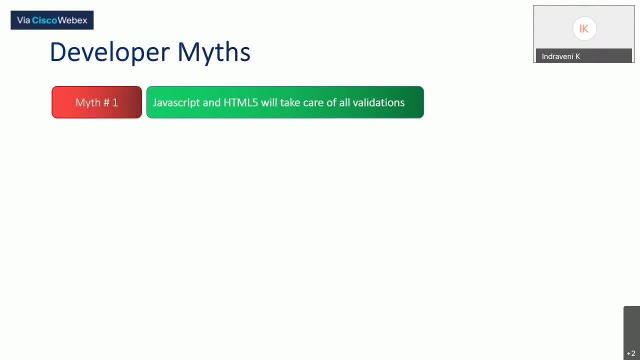 of view only this particular entire session. so, developer minds generally, what does the developer things? rule number one, rule number two, rule number three: developers have certain practices that are inside them while developing the application from the data. so the first and foremost practice, or the rule that every developer follows, is using javascript. 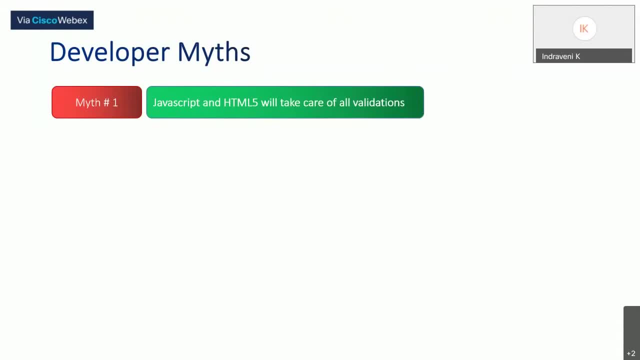 and html5 to take care of all the validations. yes, it is a good practice to use javascript and html hyper validation because when i'm filling the form, if i see some- uh, if i enter a wrong value and as soon as i see an alert message saying this value is incorrect, or as soon as i see a 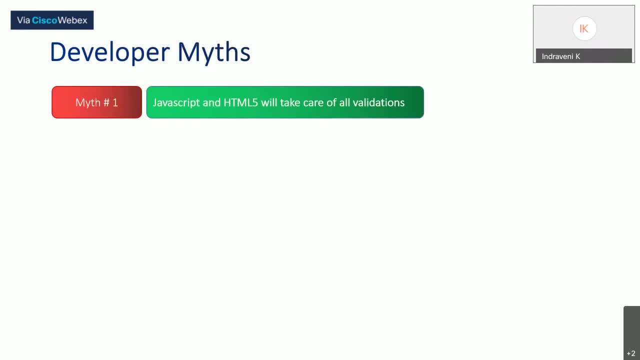 message on my next to my text field itself that this is not correct. your password is not strong. your email is incorrect. it's very user friendly for me. i can immediately go and correct my my form, instead of waiting for filling the entire big form and then finally result into. 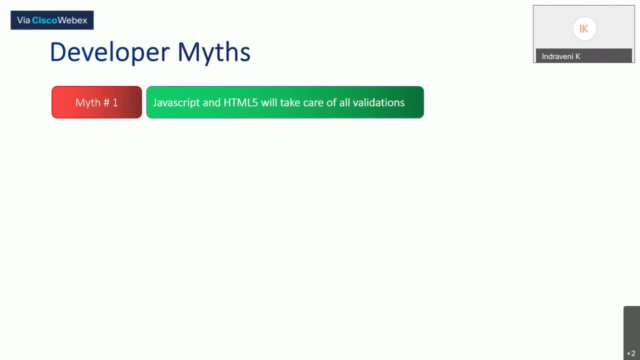 seeing so many apps. so that is the reason we do a javascript and html5 validations, so that it is very easy for a user to actually fill the form correctly. so it's a very good rule, good practice, but what is happening is my voice is not audible. 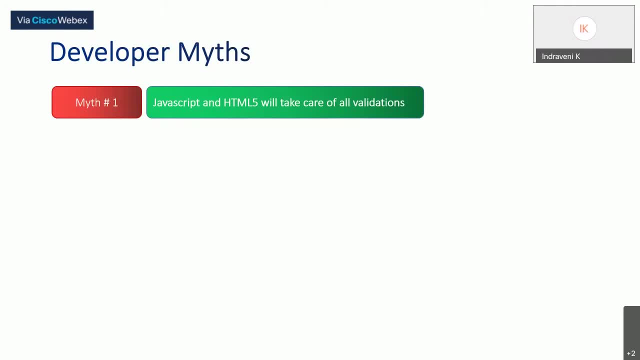 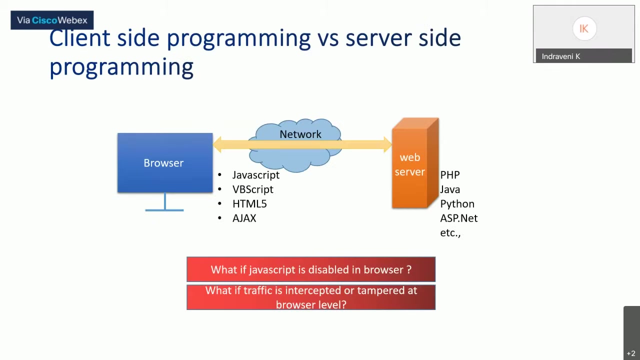 i just saw a message. am i audible? it's audible? okay, yeah, so the fifth is the first rule. but even though this validation is there using html5 and javascript tender button, still there are chances. why means, where are we doing? validation is what. that's important. there is something called as. 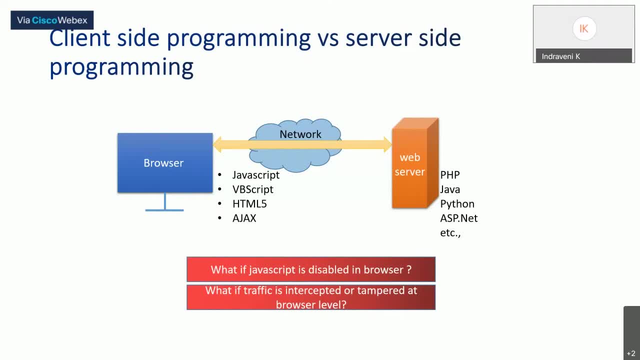 client-side programming and server-side programming. so what is client-side programming? client means, as i said in the beginning, client is nothing but a web browser. for us, a server is something. a web server is something where your actual core application is running. now, whatever validations we are doing using our javascript, html5 or ajax or 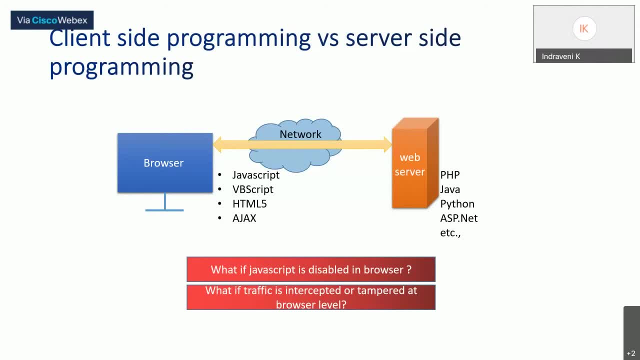 this kind of application programmings. they are all running on your browser. browser is client, so it is called as a client-side programming language. whatever code you write in programming languages like java, php, python, they are all server-side programming codes. so when you're adding your validations that your name should have only alphabets, your phone number should have only. 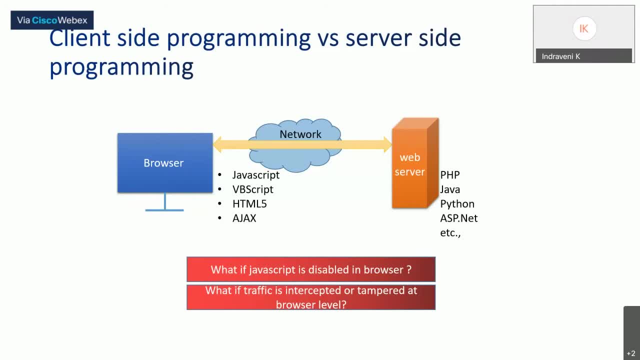 numbers this kind of validation you are adding using javascript and html5. it means that those are executed at the browser only. what will happen if the javascript is being disabled in browser? that option is there right in every browser. you can have an option that i can disable my javascript. 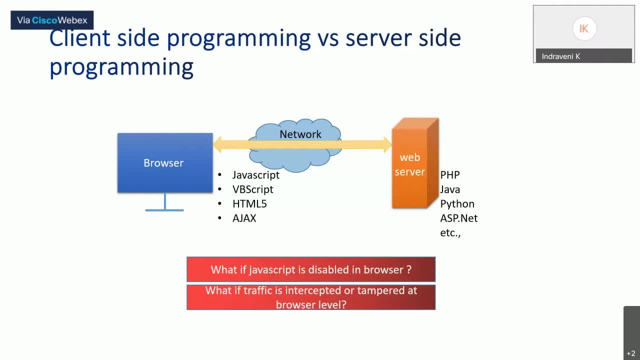 sometimes people even use text-based browsers also. so where, in none of the logics, what we implement for javascript, using javascript validations, will work? and what if somebody intercept our traffic or tamper our data? so there is a communication going from browser to server. in between there is 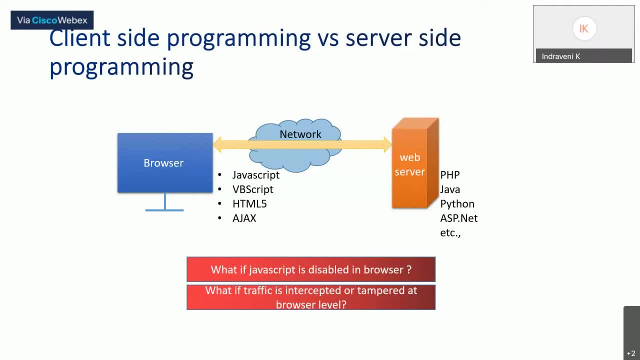 a network, right. so what would happen if somebody intercept and change their data after i put the correct value? there are, such possibilities are available in this kind of web-based communications. so these two points. if java down javascript is disabled, yes, they can do. malicious content can come in that systems. another thing: 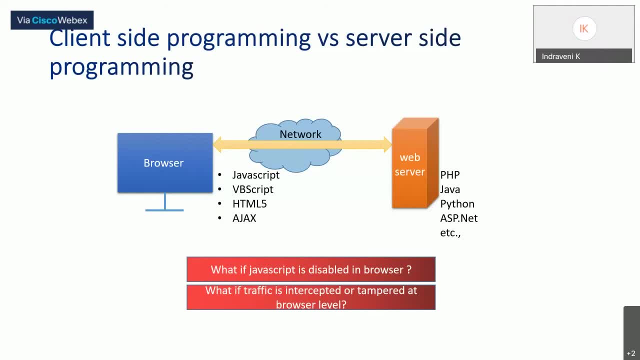 is how the interception of traffic happens. that too, at the browser level. you can see i've mentioned. what if the intercepted or tampered at the browser level? what does it mean? browser level means what browser level means? when you are adding a code using javascript or html5 validation, that validation is being called. i enter the right value. after entering. 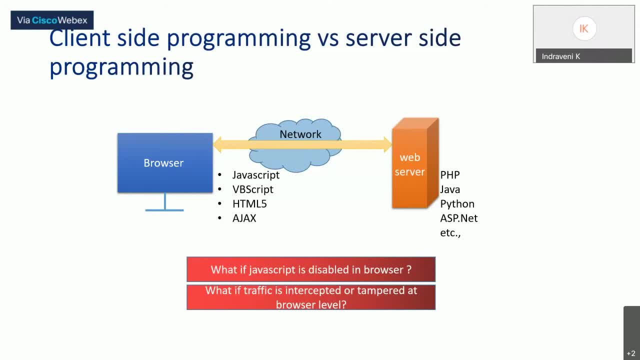 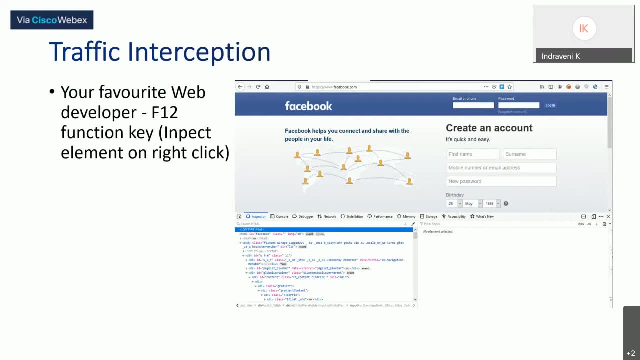 right value, then i do a tampering so that your javascript do not catch my wrong data. that is how the attackers usually work, right? so how we can do that. this is a simple examples. i'm just. i've just put some screenshots because during this session i feel that we can't show. 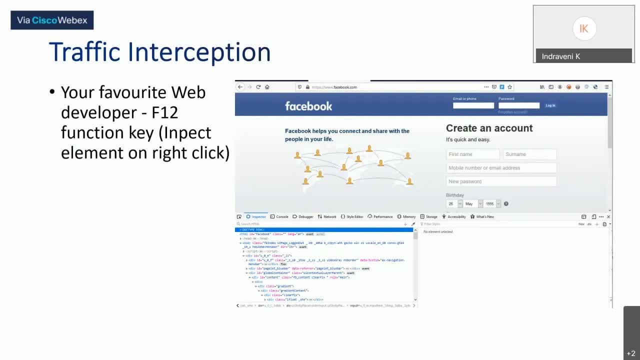 a demo, so we'll just see how traffic interception is possible at the browser level. so any website you take up, i have taken facebook because i know most of you use regularly facebook. so when you open up any website, press your favorite function, key f1- you're a developer. 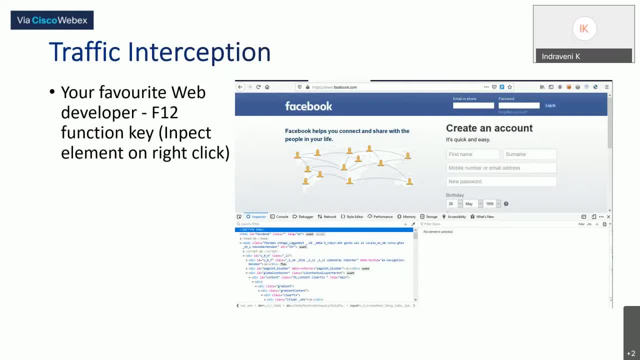 definitely. you're used to see this window by pressing an f12 command, or many of you try to right click on a given element and try to inspect it. so it's nothing but a web developer plugin that is there in the process. this is the one i'm showing is on the firefox. 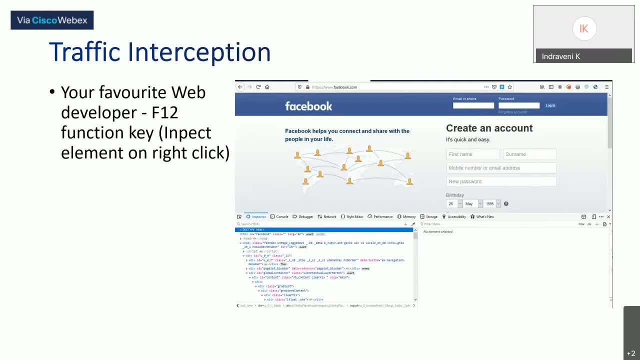 browser. so this particular web developer plugin is the one that shows you the page source and tries to help a developer to see what logic, what html code is being written under each of these fields, each of the web page content. so we'll try to understand this same web developer plugin how one can use for security point. 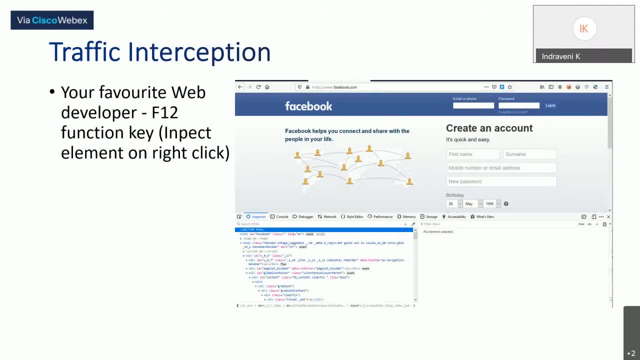 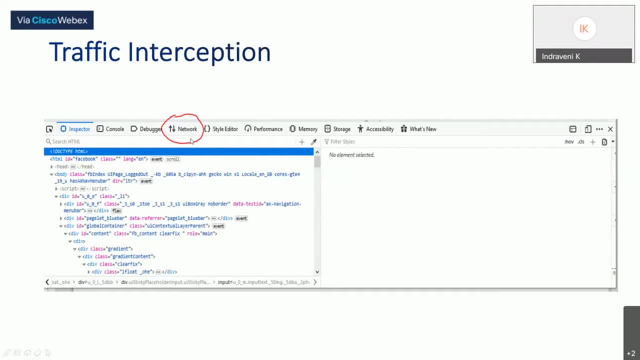 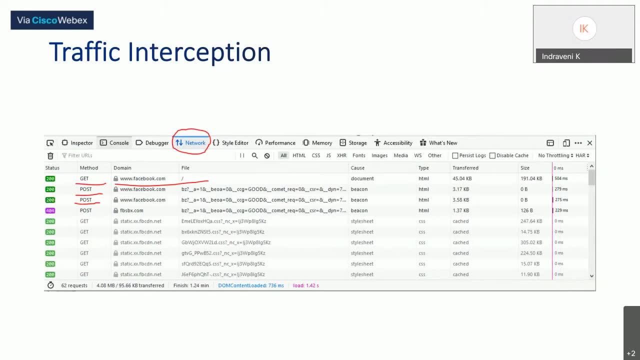 is inspected in the same tabs. you can see. the first block is inspected in the same tabs. you can see there's a network tab. so you click on the network tab and if you refresh your browser by pressing f5, you can see there will be a lot of requests that are running over here. 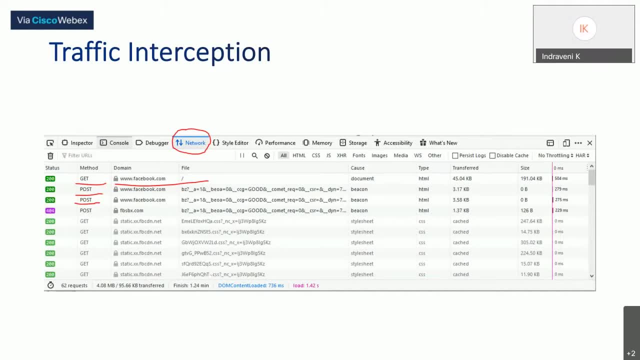 this is nothing. but when any page is being loaded on a browser, for each and every call that is going to the server- coming from an image to css file, a javascript file and index html file, every component of the web page- there is an individual request going to the server. 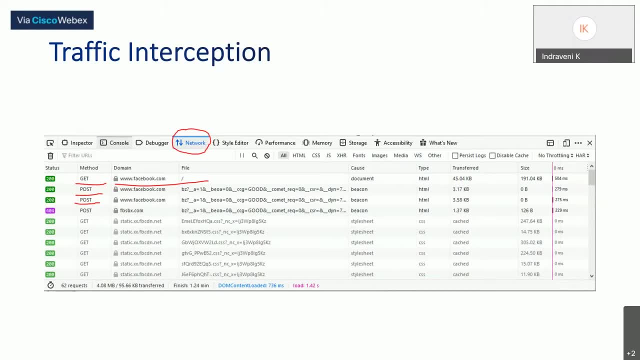 and then the web page will be going from your browser to the server. all of those requests you can see at this particular tab of your web developer plugin, under the network tab. so you can see i have just put up certain red marks under the column method: get post. 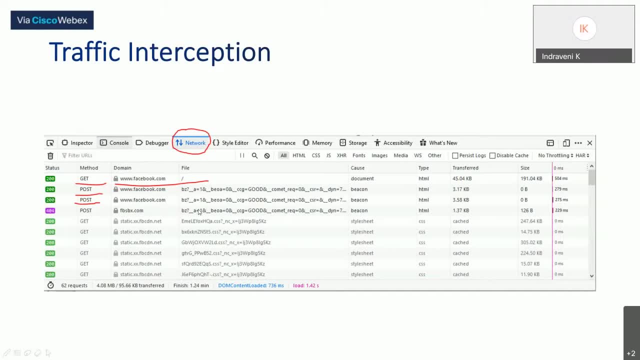 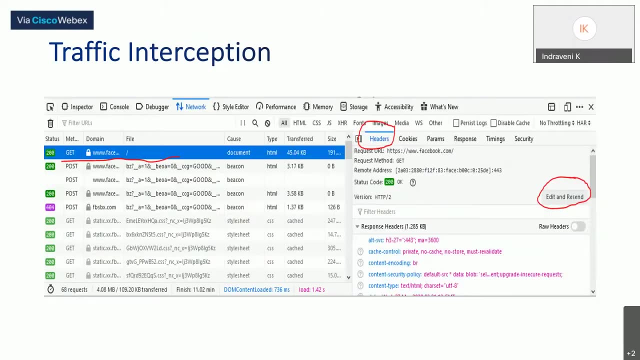 which method it is using, what is the domain and which page it is trying to fetch. when you click on any one of them- like i just click on this first one, forget. but when you click in the right side, you can see this kind of a information table. this is the information. 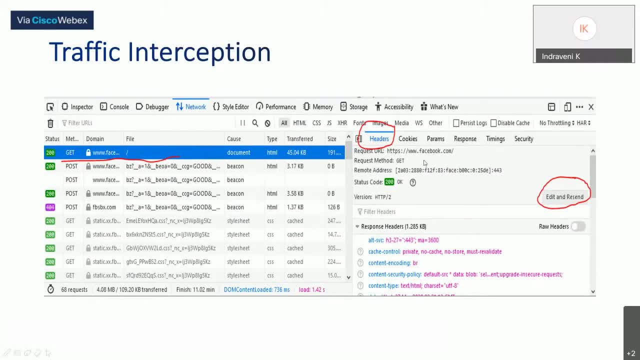 table which you can add to your web page. you can put up a few instructions depending on the opened up by the plugin. there you can see the first tab is headers. it means for this particular first request, get request. these are the request and response headers been sent from the browser. 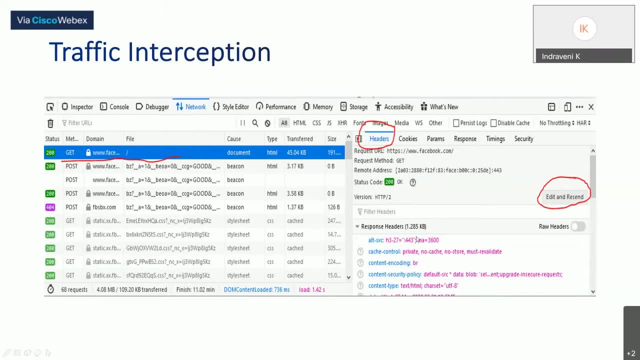 to server and you can see the request in the top. below is the response and there is an option of edit and send. this is how one can actually change or edit the request that has been sent to the server. so if you add a javascript validation for any application, then after the javascript, 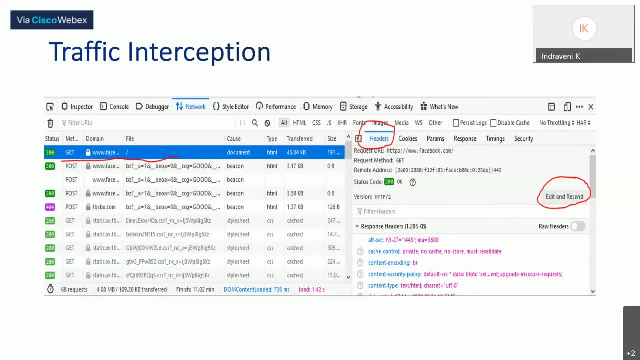 validation request is submitted, i can resubmit the same link by just clicking on this edit and send option and enter the data. when i say edit and send over here, it will try to open up the post contents which i can just edit the value and send to the servers. so this is how your 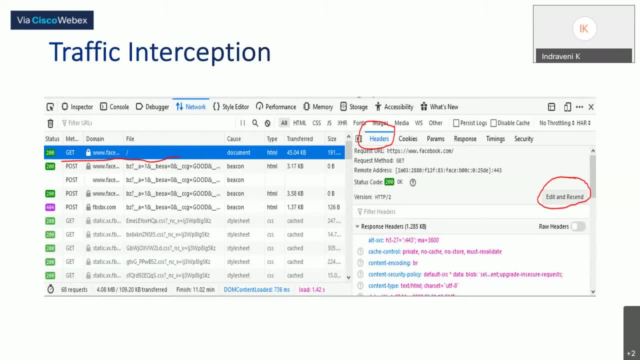 data that you are sending from your client to server can be edited and sent to server- nothing, but you're intercepting the traffic. in fact, we don't call this exactly as interception, because interception is something wherein, in a live communication, if i'm trying to stop a communication, 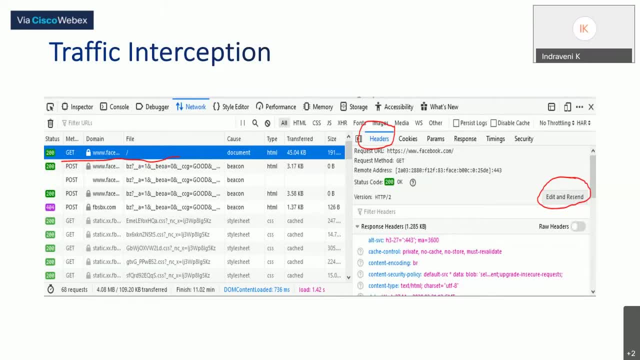 change and send that is. that is one way, but this is also the the way in which we are trying to capture the traffic, alter it and send it at a later point. so this is also possible. so your javascript variations would not work if i or if you are. 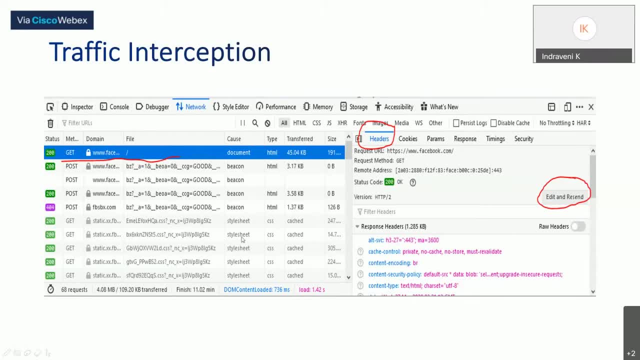 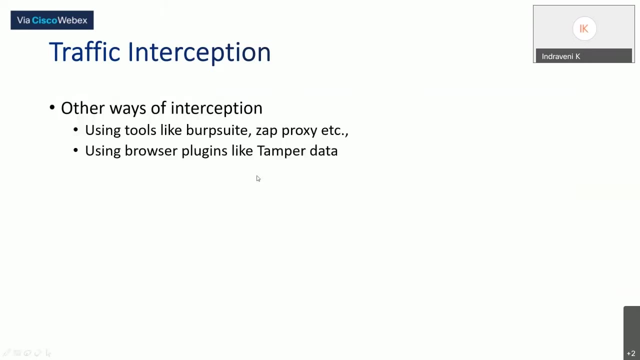 putting up in your applications. i can click on this. this way i can go to individual page and try to edit and send the particular requests to you. generally, this activity is done using the tools like burp, suit or tamper data kind of plugins, and all are also used. 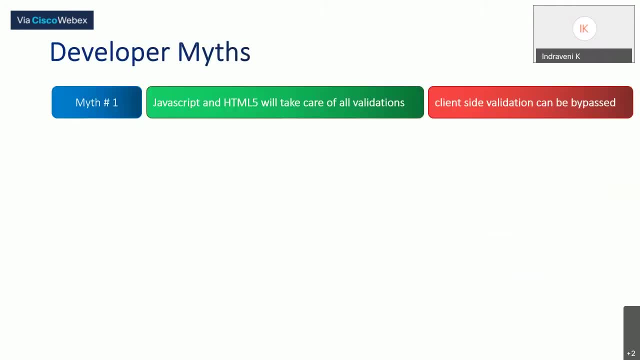 for changing such kind of data, usually so client-side validations can be bypassed. one way, consumption, is disabling javascript on your browser. other mechanism is using tools like this kind of plugins, wherein i can alter, click on any of the requests, change the content and send to the server. 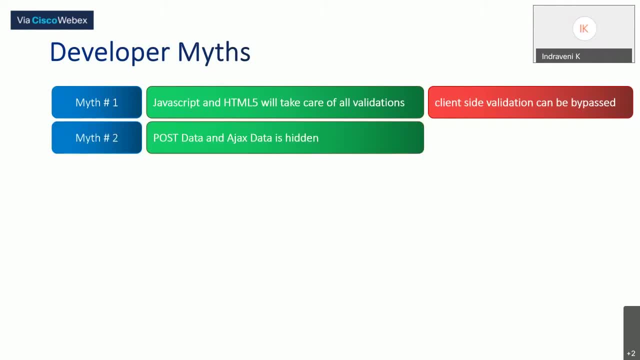 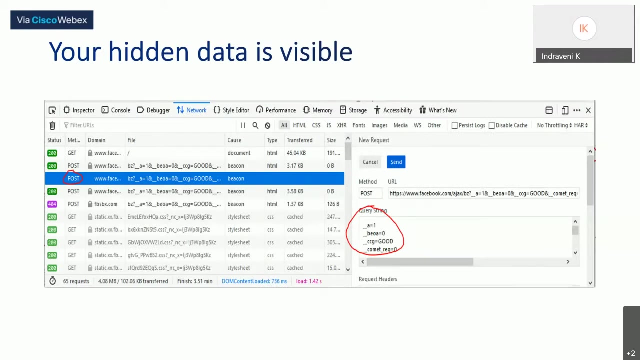 rule number two: most developers think that the post data and the ajax data is hidden. so many people put sensitive informations into that. many people could uh consider that since it is not visible, nobody can alter it. but that's not the thing. what i want to show you here is that the post data and the ajax data can also be seen. 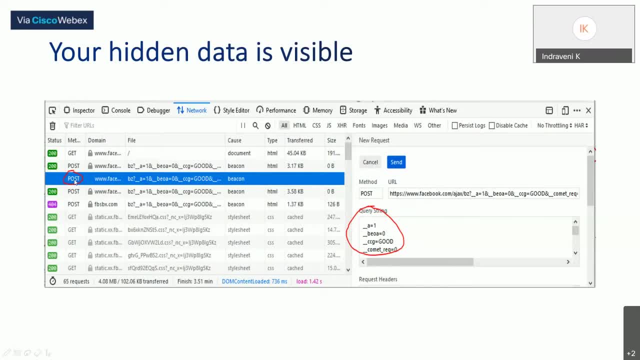 through the same plugin again. i've just gone to the the post method over here, the third one, which i have marked right over here. when i select that in the right side, you can see the similar one. when i click edit and send button- what we have seen earlier- you get this kind of a screen. so 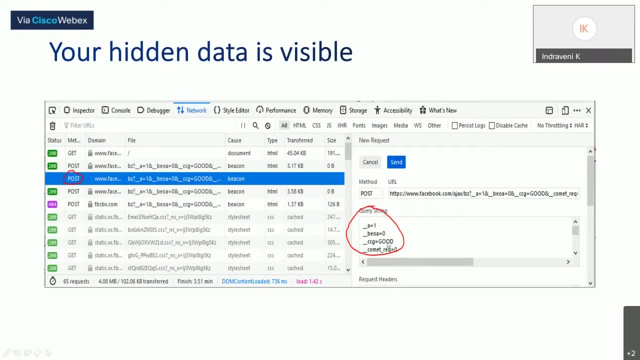 first block. you can see the post method, followed by the url, and then these are the query screen values that are going for the system over here- and click on send. then my changed content is being sent to server and at this moment low javascript validation will stop the request. no html5 validation will stop the request. 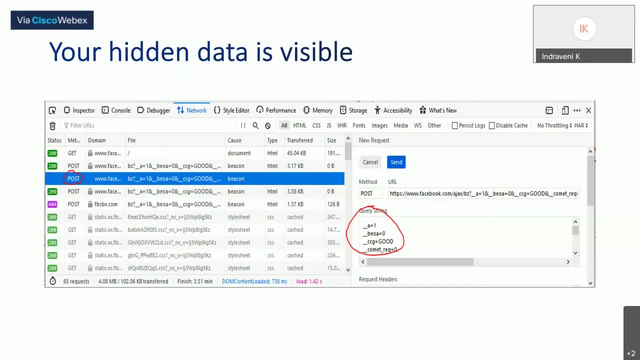 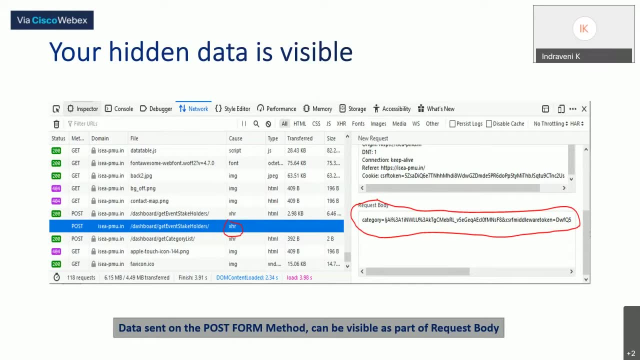 so that is how the information can be tampered and, as you can see, this query string is a post method. but this is one more example for another website where you can see this is a post method. the post data is actually going as a body over there request body separated by ampersand. so we can 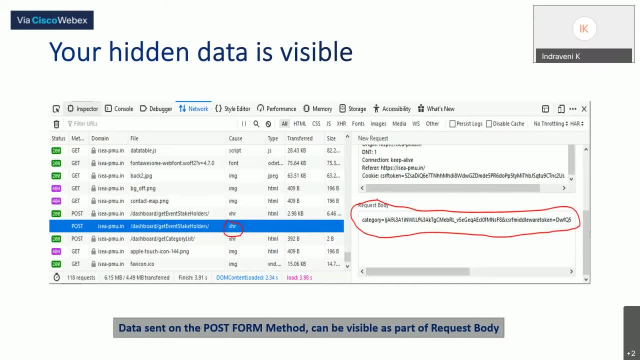 tamper this and send it to the server. so changing the post data is also is very easy, as easy as you are changing your get parameter data. so your post datas, your ajax data, ajax data also can be visible in the same way. so they are not hidden, they are just not visible. they are always visible. 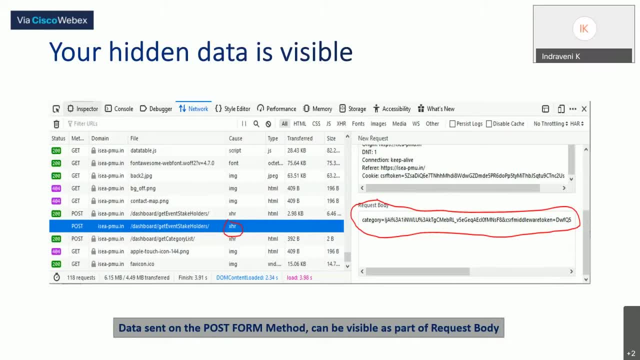 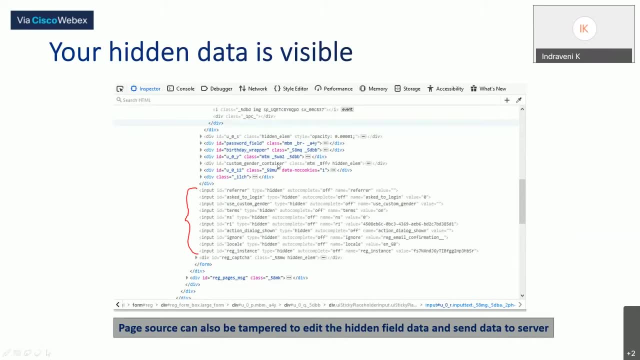 in the part of the request volume and in the page source. most of the times we put input fields in the type hidden and most of these are not visible in a normal browser. but attackers who really want to perform any attack, they try to look for something which is hidden. 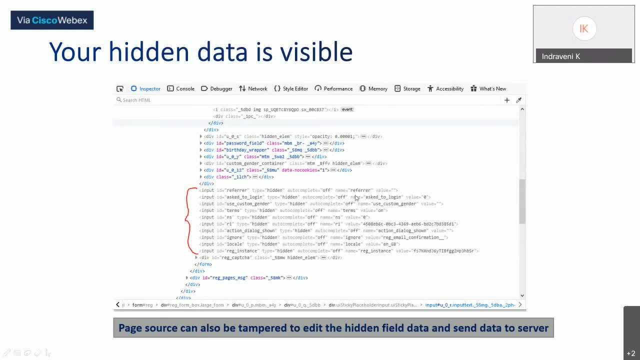 so you can go to page source. there are hidden options. if i just enter some values over here and try to submit, since it is hidden in front end, you may be thinking that nobody will send an request, but if you are sending a request, your server should, if it is accepting the request and 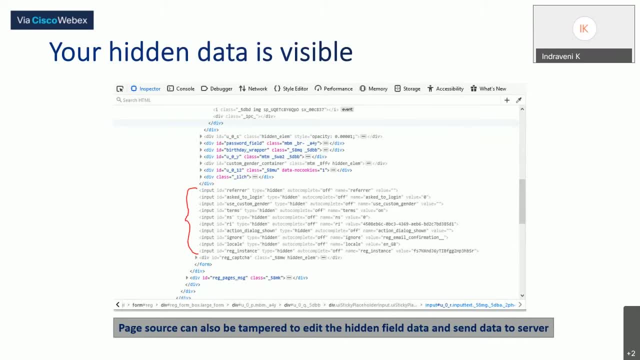 processing it. it's not a good practice if you are hiding something from the front end. your backend server logic also should take care that you should not accept a value from that hidden parameter. is it clear? so it's always recommended that your server side logic should be. 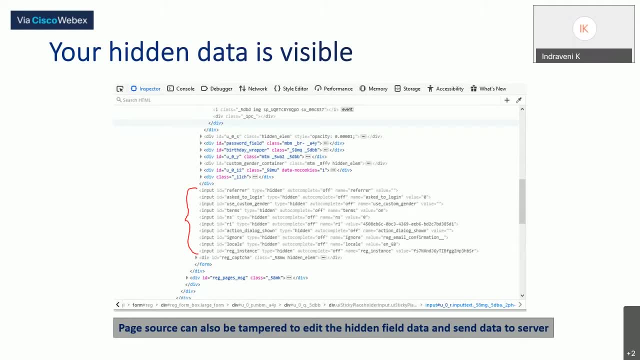 in line with your client behavior in client. if you are hiding something, if you do not want to accept anything, do not just comment the code from the front end. do not just change the types to be hidden or something like that, because those can still be made visible, those, those parameters also can be. 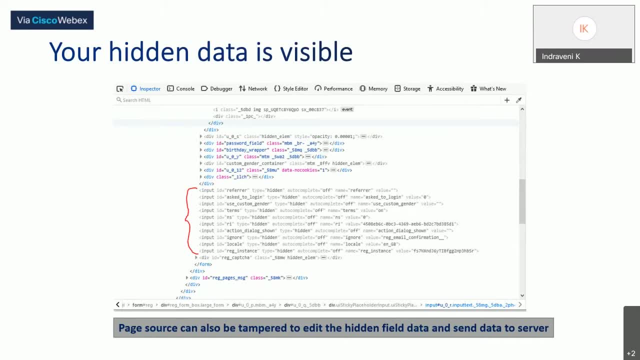 inserted with some data that your server, if it, is accepting and processing, can lead to unnecessary behavior on the systems. so whatever you feel is hidden is not always hidden. it is visible and it is temperable, also including the radio buttons, the buttons that are used to enter the server. 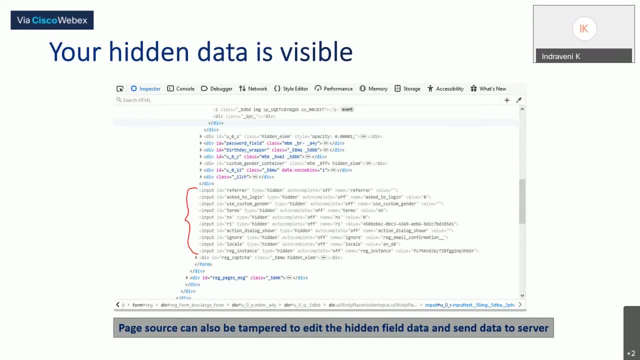 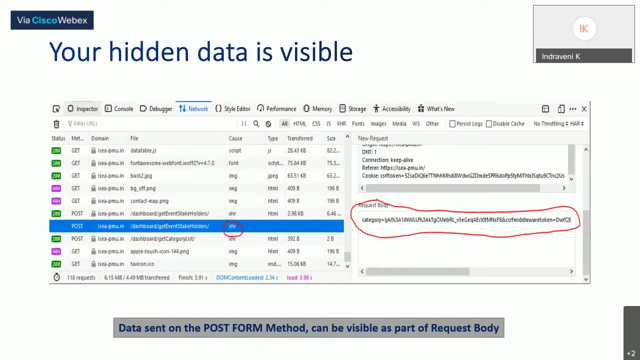 you see in your form, data, the check boxes, the drop downs, what you see, all of them are temperable. the same way, if you use a drop down box or a radio button, those values would also be visible to us in this same request. body like gender is equal to f if you are putting the radio. 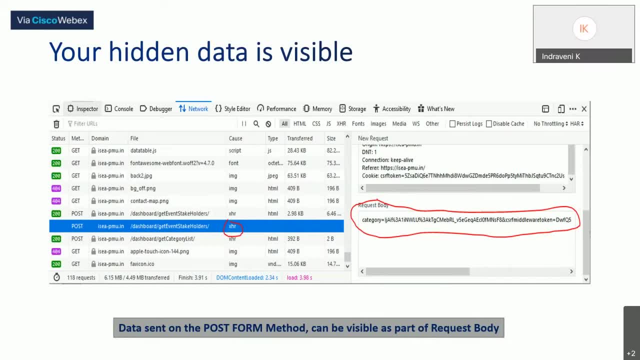 button, gender, female, male and for one box, the value of the radio button. the value is f and m. you can see those in this request body are equally and i can change that. instead of f i can put number also. so don't consider that your values- whichever is hidden or read only- are always like that. 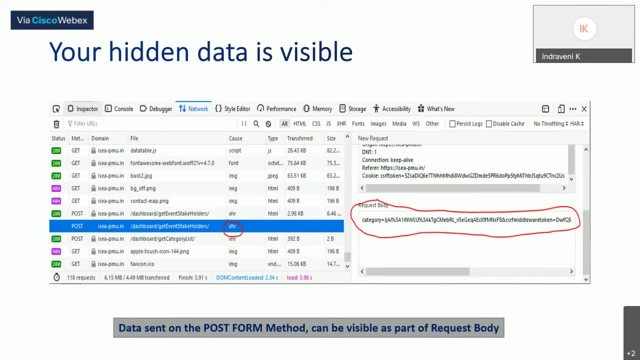 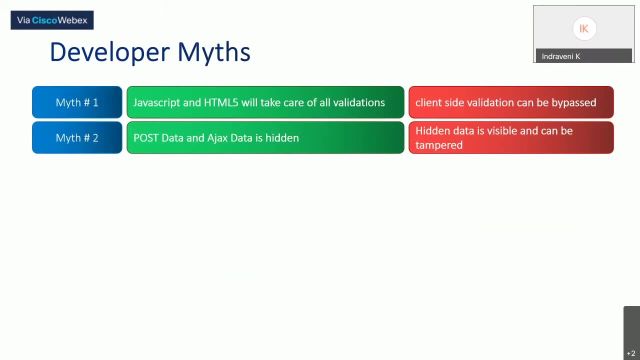 they can be temperable. there are so many mechanisms, so many tools, that which one can do that, in fact, this is not any tool. this is a simple browser plugin. the intention of this plugin is to help the developers. okay, so, with respect to our second mic, our hidden data is visible and can be tampered. 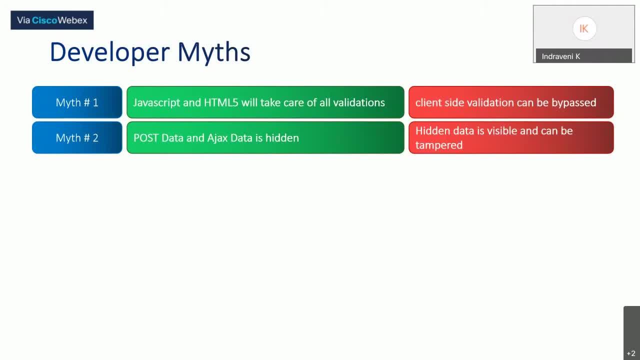 so be careful: what you are keeping in the hidden mode, what you are keeping in your post data, as well as what are you sending in the agile screen. the next myth of the developer is: cookies are always server generated and it can be used for business launches- correct cookies. 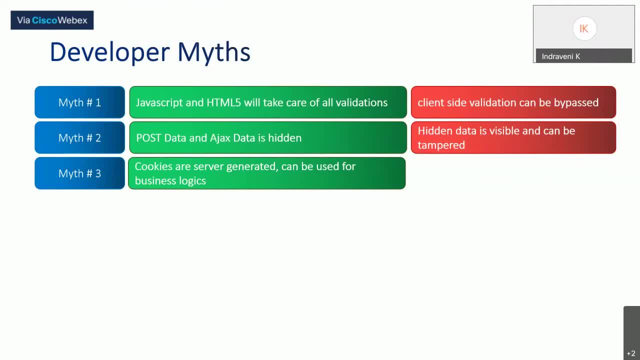 are generated by servers. that is true, and that's the reason. what are cookies? usually, these are something which, through which we try to store our session ids. we have our session. each of our session id can we can store on the cookies and most of the time we decide or perform certain business logic based on the sessions. 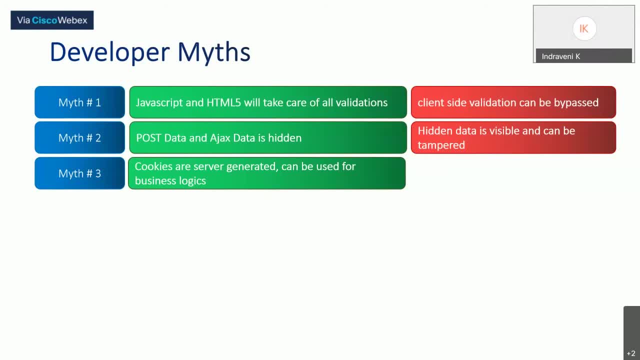 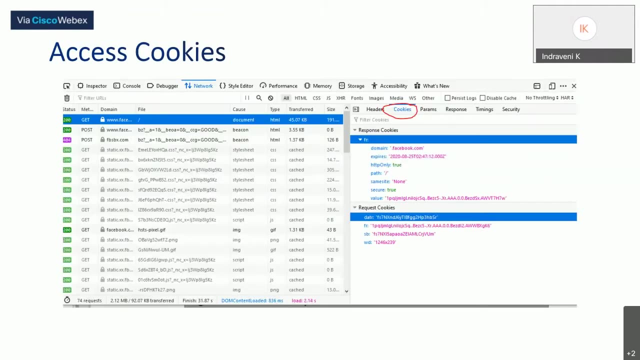 most famous business logic is whether a valid session is there or not. you see whether a user is logged in by checking his session id and then you allow him access of the particular given page. but even with cookies, what kind of problems can come? let us see. so we have a request for a plugin, if you see. 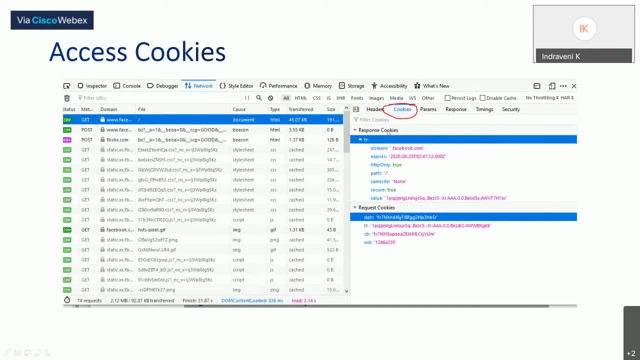 i'm just accessing again the same request and if in the right side you can see the next header tab which we saw earlier, there is a tab called cookies and this tab shows you information about response cookies and request cookies. so request cookies are something that is coming, that is. 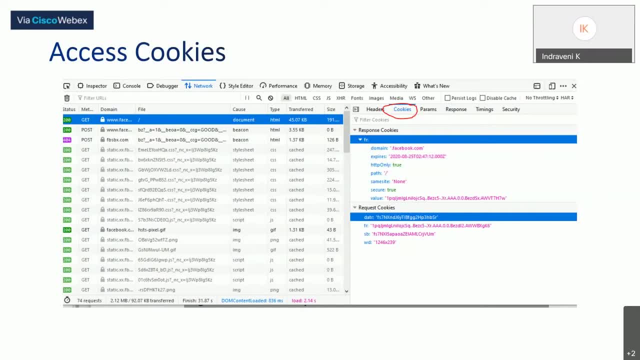 being sent from our browser to the server. response cookies are the cookies which are sent from server to client, so request is from client to server, response is server to client, and those are these cookies. now, these cookies are also, as we were discussing earlier about javascript: validations can be tampered. we're also discussing about hidden data can be edited. 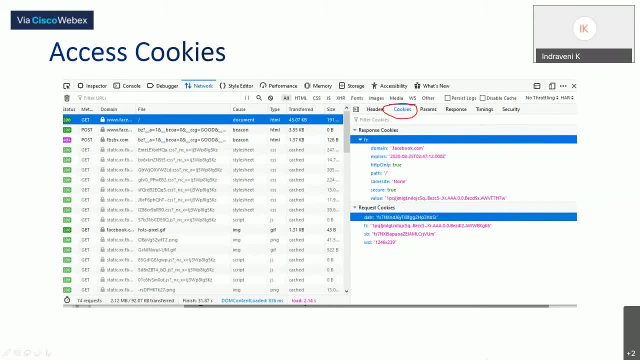 cookies also can be edited. now what you're seeing over here are cookies. if i just right click on this cookie and say edit, you can change this cookie value to something else and send to the server also. you can change this cookie value to something else and send to the server also. 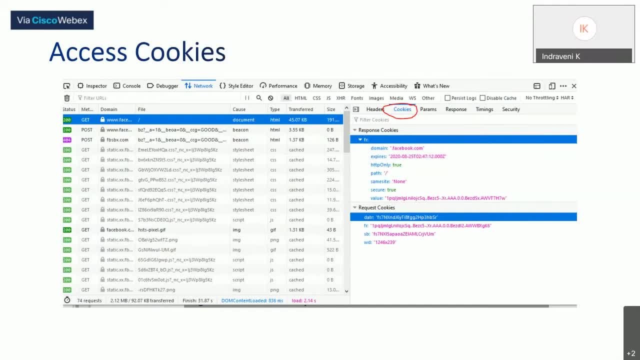 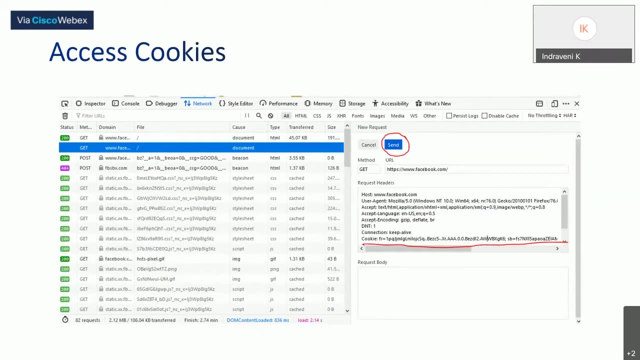 what if you put business logics into these cookies? what can affect? one simple business logic that most developers use is something like deciding on a specific role, kind of things. so how do we go? there is something like this: edit and send and then you can come. there's a content over here. the key is there, this value. if you edit over here, you can. 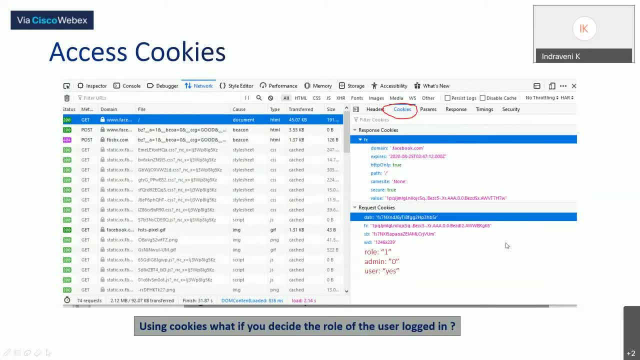 just tamper and send to the service. so in this screen you can see the bottom request cookies. have just added certain more cookie values. as an example: role one: admin, zero user. yes, so these are usually. most developers try to maintain the type of the user by setting this kind of cookies in the systems. 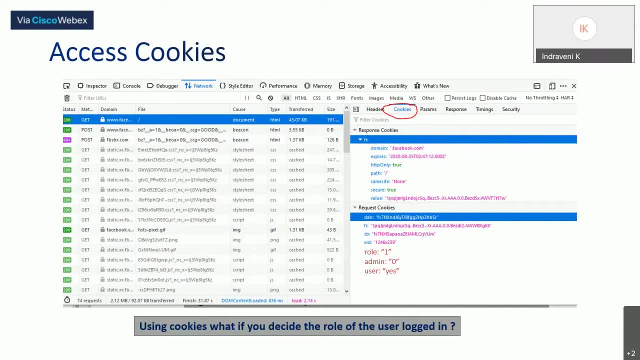 so whenever there is a request coming from a browser and if it is having role as one in the cookie value, he may consider that that particular user is an administrator, or he may consider that that user is normal user. so the user is normal user. admin may have zero, so it depends on the logic. however, 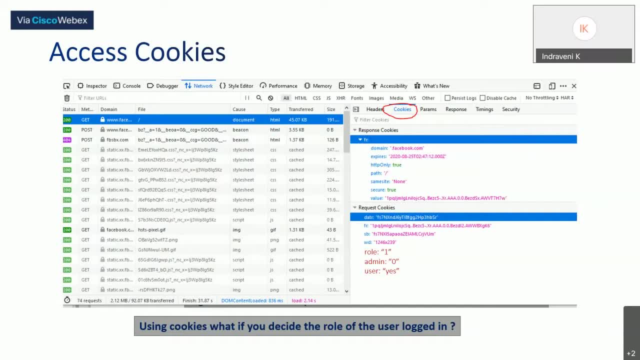 the developer is trying to decide upon what role the user is, based on the cookie that has been sent from the client to the server. so here, role one, admin, zero user. yes, these are certain examples we have here. so this way, many of the times in applications, this kind of decisions, business logic decisions, 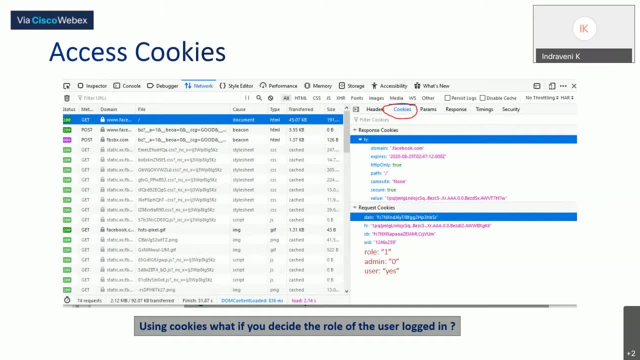 decision upon the user's role are being done based on this kind of cookie values. so if such thing is done, what can happen? yes, as an attacker, if i want to perform any attack, i'm using this particular function. i just come to this particular plugin and go to the headers edit option and i just change admin. 0. 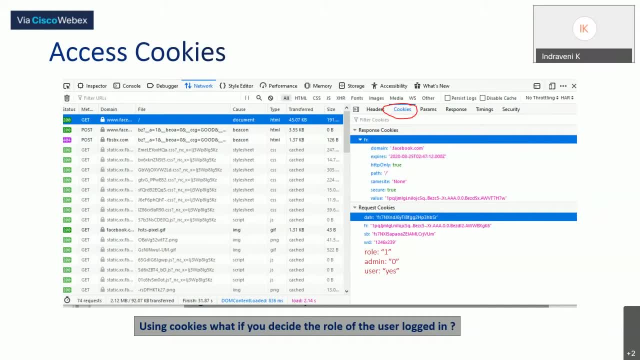 to admin 1 for saving, irrespective of my login credentials. i'm just i can log in and i may become an admin. and if i already have an admin and i say, can the admin Heart Drop While" です, all is a list of em, simple organizations like 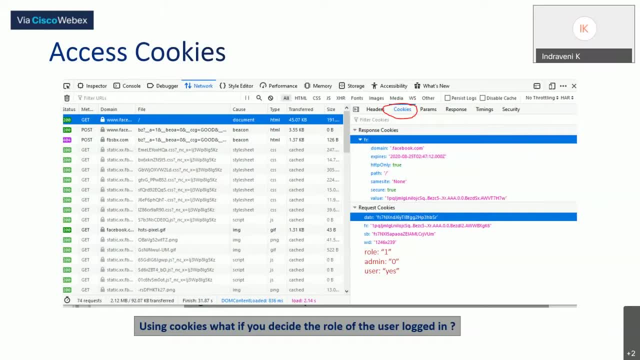 the submission data in user will never behave the way you want him to do, him or her to do. once a user logs in, he can do whatever he want on the systems. so we can tamper any data that you can see. it can be cookies, it can be posted data, it can be get data or anything else, and nothing is hidden in the systems and 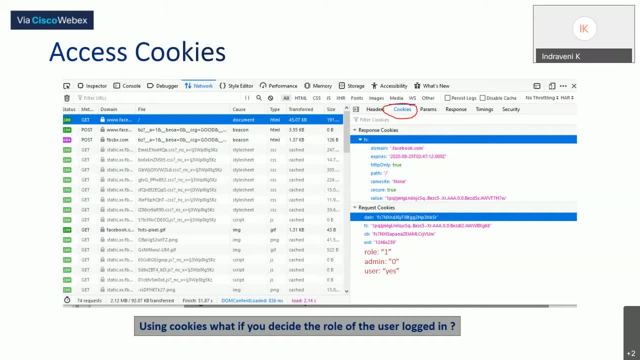 remember one more point: all of this that we are seeing is at the browser level only, so this is how the cookies can be seen, can be edited, and if certain business logic, these kind of critical business logics, are being decided using cookies, then it should be avoided, because 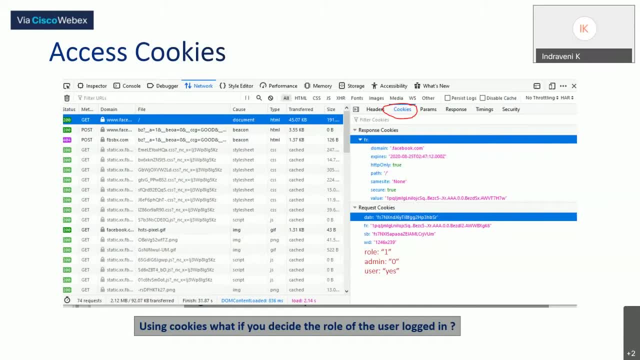 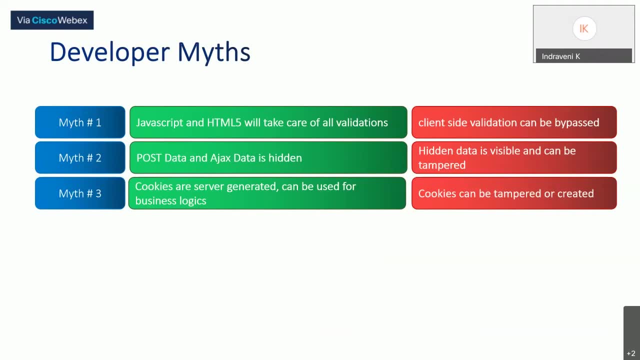 these are also tamperable and one can change these values to what they wanted to, or try it, so cookies can be tampered and even cookies can be created. there are so many vulnerabilities related to cookies or with respect to obsession, so a lot of tampering and relational things are possible. only thing is, we should always have 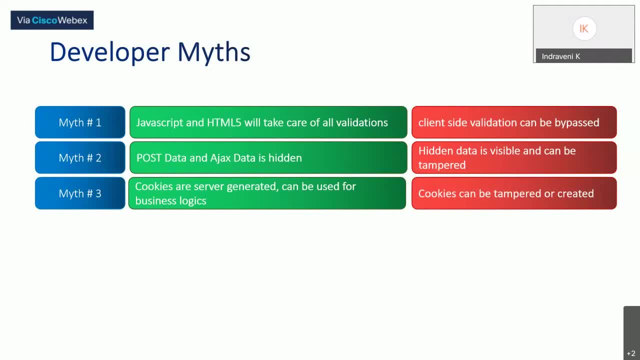 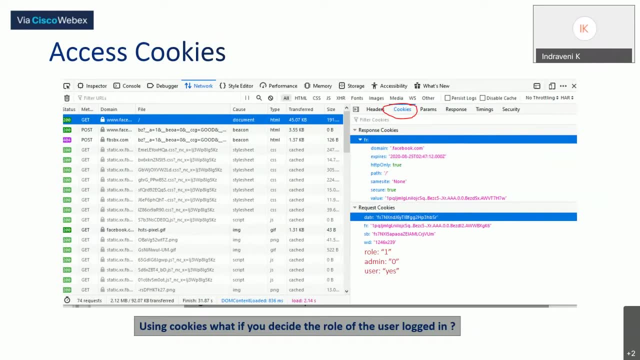 server side validations for everything, any input that is coming. say, for example, you take the same screen if an admin is zero or one cookie value is coming. every time you have to say at the server level: you should see whether this users is an admin or not by verifying it on your database. 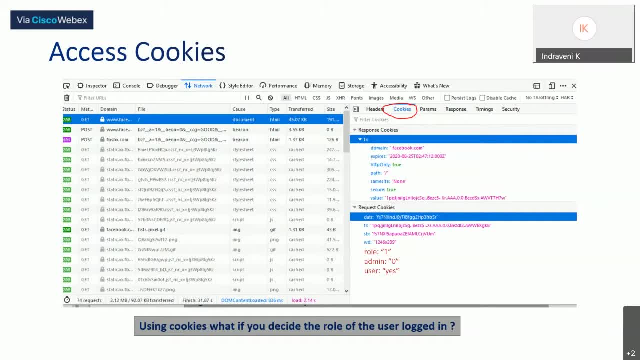 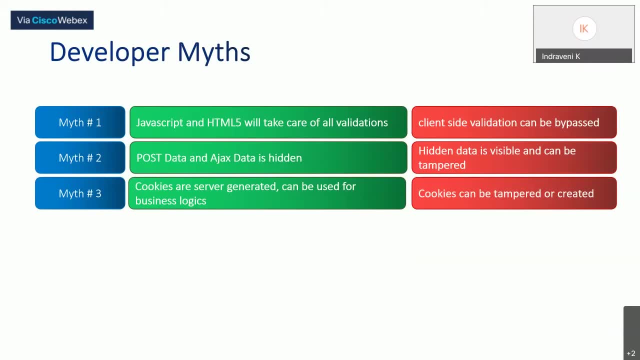 rather than get taking confirmation based on the cookie value that is coming from the client. okay, so what we remember is cookies can be tampered or created, so though they are generated at server in the beginning. further wages the following requests: cookies comes from the request part for part of the request, and thus they can be tampered and sent to the service. so be careful when. 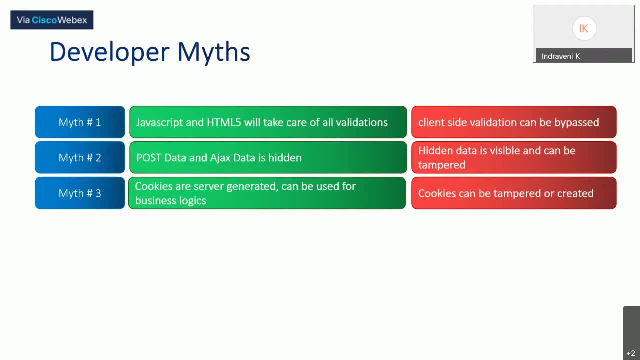 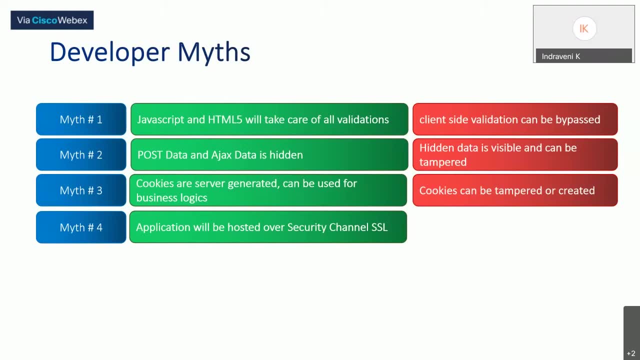 you are putting up business logic in these cookies, and the last myth that most developers think of is that they are not going to be able to handle the security of the application. so most of the times, what's been coming across is any vulnerability. you talk about any attack. 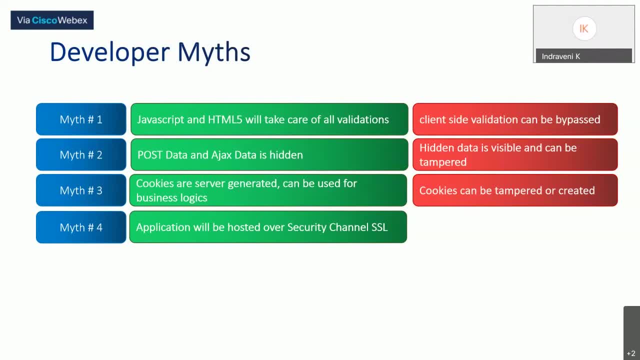 you talk about. the first response that we hear from developers is that no, no, my application will be hosted in ssl, so it will be secured. what is the security that ssl is providing to you? does any of this so far? we have discussed about these three points right. does any of these things? 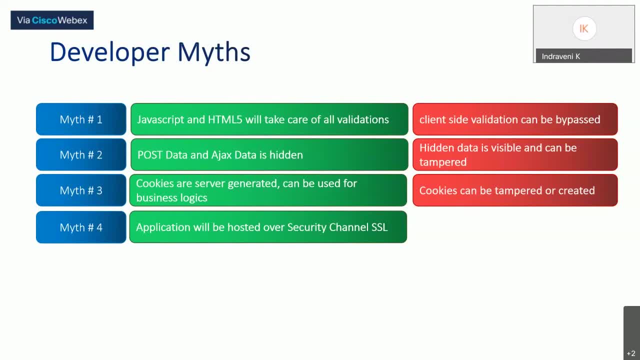 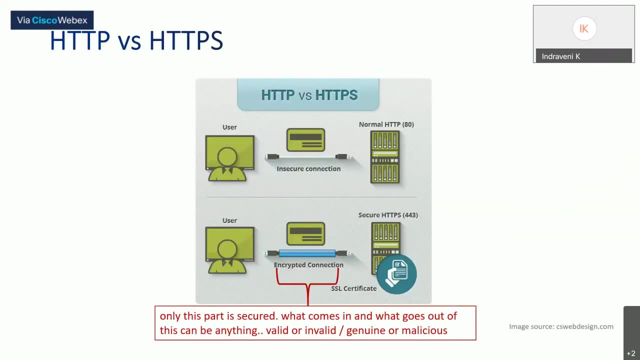 uh, i mean, does ssl stop any of these points? if i have an ssl, is it not possible for somebody to bypass a javascript? let's answer this once we understand the next slide. that is this: let us see what ssl is doing. i don't want to go independent network level what ssl does, but as a developer what you should. 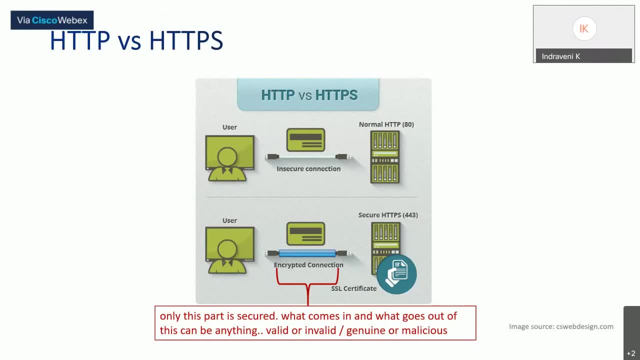 understand is from a user to the server. there is a communication coming. the first block in the top it's a http request. it's a normal tp communication. so where this communication is known to be insecure connection, insecure connection means in between there is no security, so somebody sniffing the data in between doors. 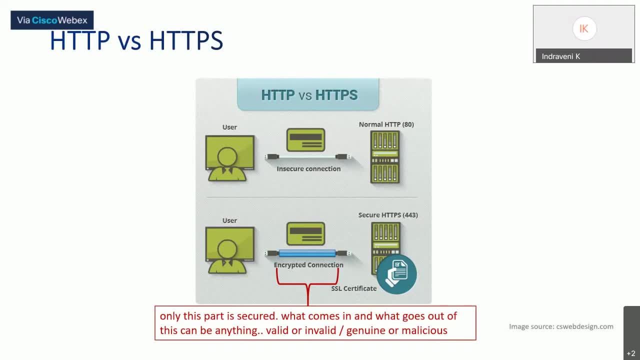 the network or the bandwidth can actually do something in the data, over the data, and thus there is an ssl coming in the bottom over here where the blue secured box. what you see here is an encrypted connection. so whatever is coming from user and reaching the server, it is all encrypted. 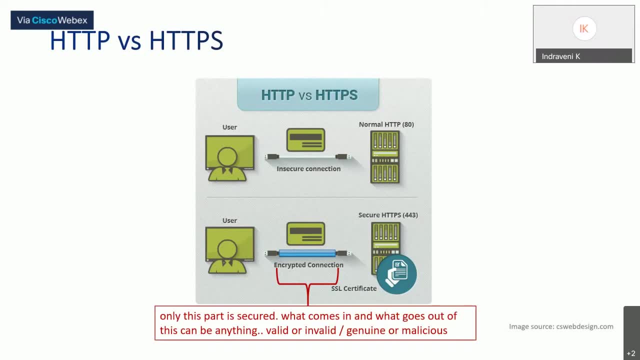 with proper certificates, additional certificates, proper essential keys. the data is encrypted from user to and it is sent to server safely. so this particular part, what comes in and what goes out of this, can be anything. it can be valid data or it can be invalid. it can be genuine or malicious. so whatever is coming, 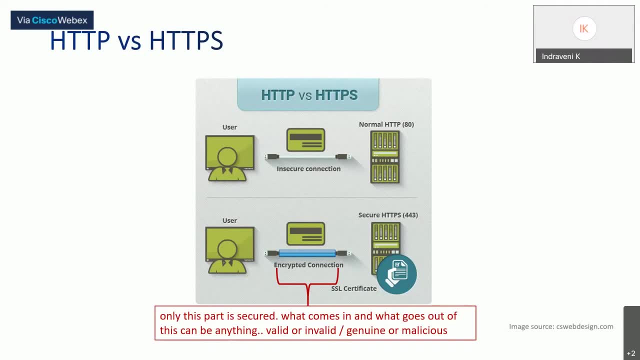 from the user to this encrypted channel is what you see at the browser. so the point which we discussed: if there is a javascript validation is there, i can still bypass javascript and insert something else and send to the system. even that data is sent securely to the servers, so in a way the web attacks also gets encrypted. 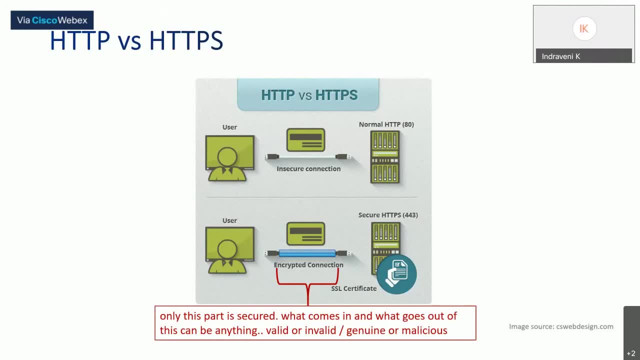 and sent to the server. it's not that web attacks are not possible. web attacks are possible in a similar way. only attacks which are not possible is is a network level attacks. if some body is sniffing the data in between, that data sniffing is not possible because there is an 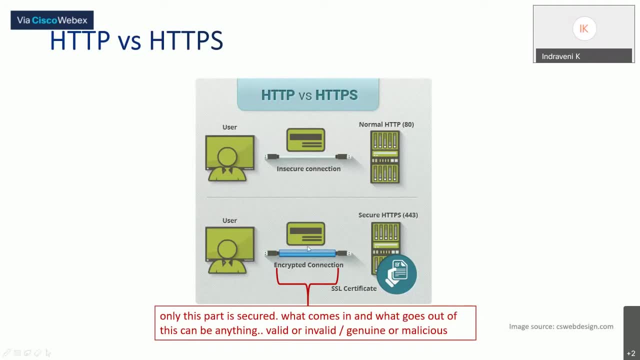 encryption over here so nobody can sift the data in between the traffic. but whatever attacks we are doing at the browser level, at the client level, i am injecting something. i am doing javascript changes. i am changing the post data, i am changing the cookie value. all of them are possible at the 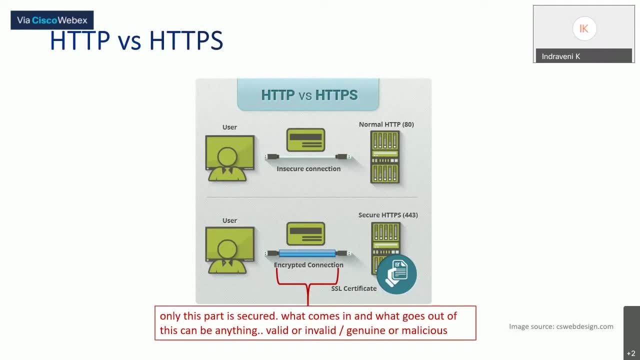 user, even if there is an ssl certificate, even if there is a https communication. so ssl, using ssl. for developer, if the application is having ssl or not having ssl, it's not at all any relevance for you. whatever security practices you have to follow for your application, it has to be followed, irrespective of having ssl and non-ssl. it doesn't have any. 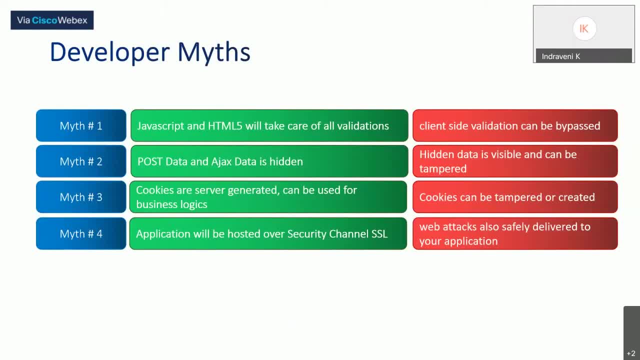 relation with that. web attacks are also safely delivered to your application. if you have ssl, that is the only thing ssl guarantees you. okay, so ssl encrypts the data. the main purpose of ssl communication is to maintain the confidentiality of the user credentials which users enter on your applications browser so that those are encrypted. 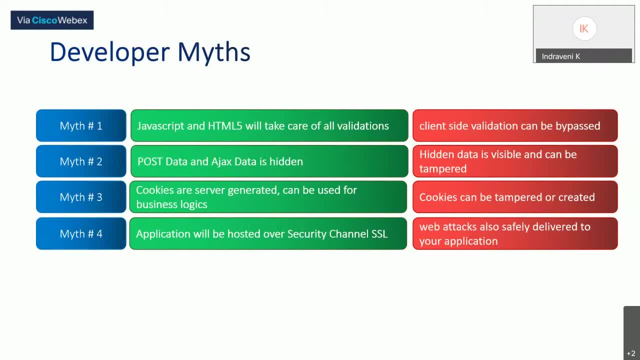 and sent. nobody can slip the data in between and hack the content, okay, but your attacks- whatever we saw in the beginning slides all the infection attacks and the fire attacks. everything is possible, even if the site is having ssl. so these are the four known rules that every developer we have seen that they follow, but unfortunately these do not help us to protect the. 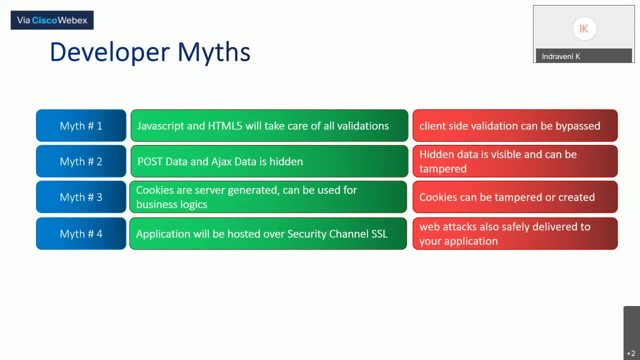 web based attacks. there is much more to do to secure our applications. simple javascript validations post data communications. considering that i'm login page, i would not send username password on the get. i'll say: not post. it doesn't mean that you don't do validation on those fields. it is required because they are still visible. 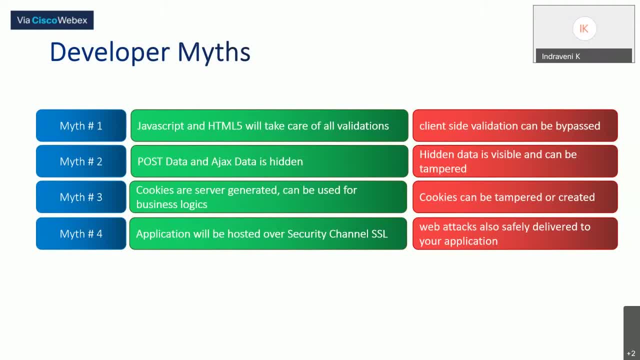 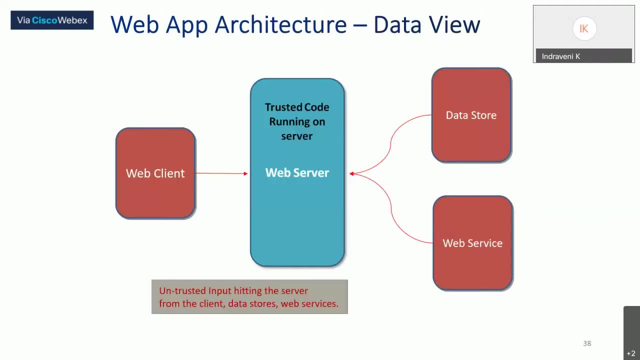 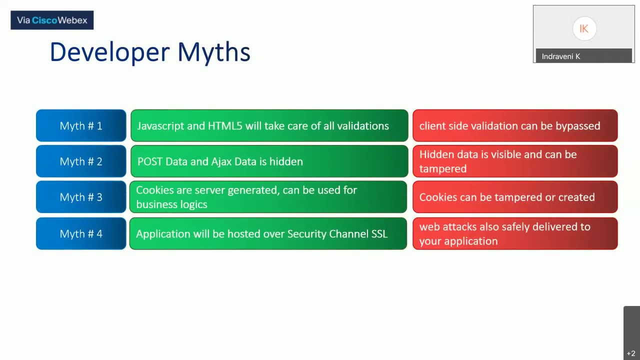 they can still be tampered and do whatever it can. okay, so, moving towards further, now, these are the mites. what we discussed is about the general practices, what every developer follows, but how those practices can be, uh, misused by attackers. that's what we discussed so far. now we'll just try to look into certain few attacks and their related. 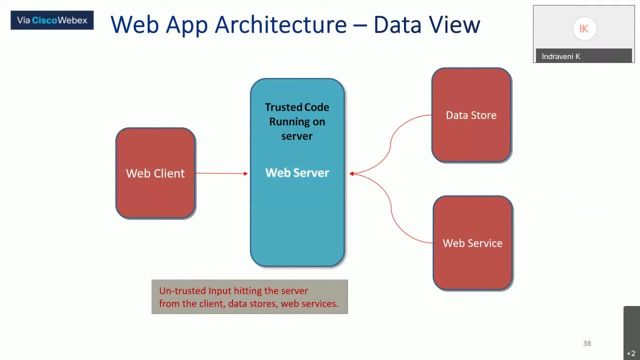 circuit coding practices. so before i go further, i just want to show a data view of the verification applications. you are having a web server. in web server, whatever you are hosting is the trusted. why is it trusted? because that is the only piece of code which is developed by you, which you know. 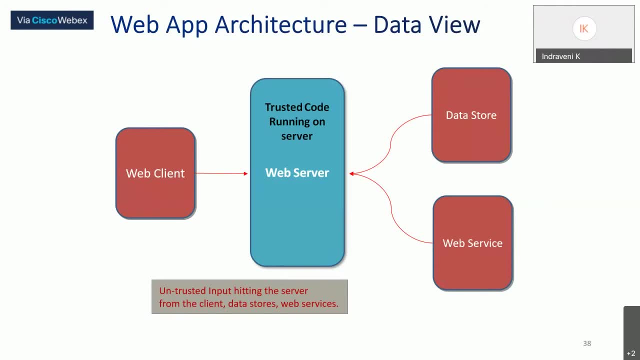 said it, you know how your program will behave if something goes wrong with your program. that is the only piece of trusted code in your system. whatever is coming to you from the client, the client- whatever is coming to you from your data store, nothing but your database. and as well, whatever is coming to you from the web services, web services can be the calls, ap calls. 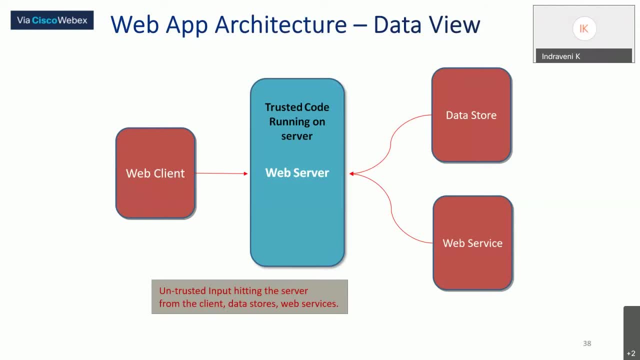 which your server may be accepting from external sources. sometimes there could be certain requirements where your server should actually take inputs from different uh with some kind of statistics or some data processing or something. anything that is coming as inputs to your system, to your application, should be considered as untrusted input. 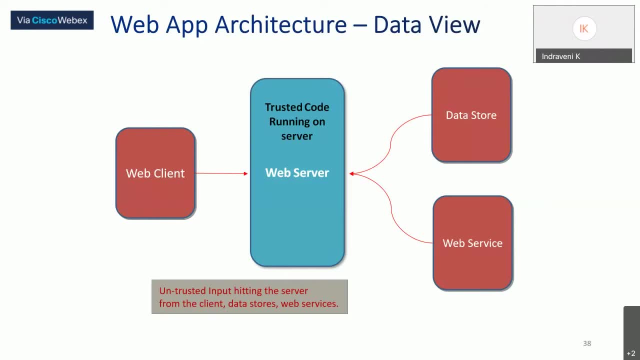 it means you have to validate that input. you cannot trust the data as genuine untrusted means. validation means what we have to see: whether that input is having the content, what is expected by you, what is required by your application, or that's very important. so, whenever you are designing any application, 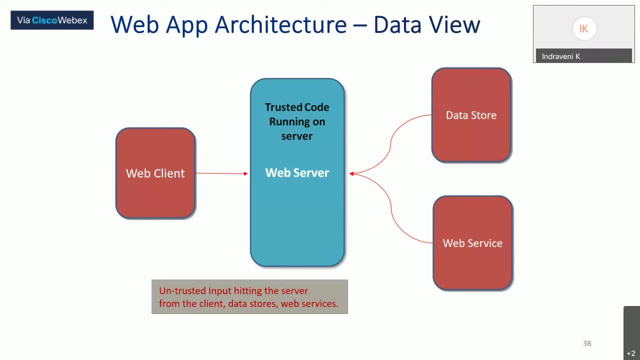 you should think of. what are all the sources of your, of the data from to your systems? i'm referring data store over here. you might be this question: that data store is nothing but the database, and in database the content is getting stored from your application only. so how can you not believe that we can? we cannot believe that as well. we have to validate the. 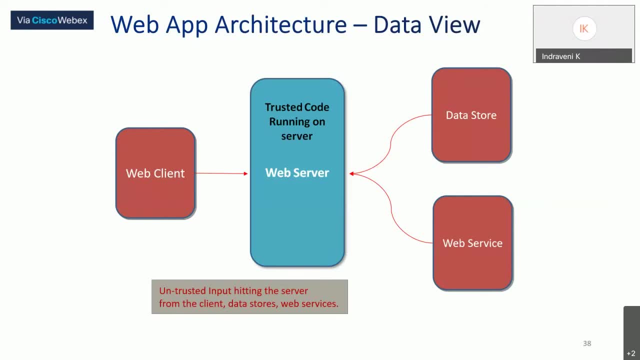 content that is coming from the database, also because there are different types of attacks. by any chance you miss out somewhere. some validation and malicious content is going and sitting in your database through different sources. that should not affect your system again. as an example, there's a crosshair scripting attack- stored crosshair scripting. if you say, 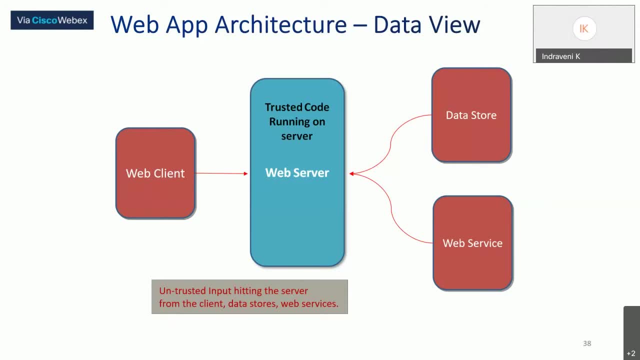 that's an attack where people just try to insert malicious content into your application which can just be taken up and stored into the database. one simple example i can give you is that i'm sorry i didn't give that slide, but no, i have got it. so one simple example i can tell you. 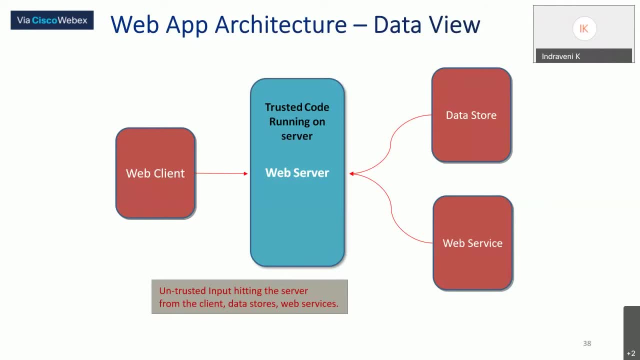 over here is, say, there's a registration form and in that you have a field called address. most of the times, in our indian context, especially our address have every special character that you want. our addresses usually have door numbers, slashes, survey numbers, call and hyphen- all types of special characters that are there in your key codes. most of the time they are stored in a public key like github or google or google plus and so on. 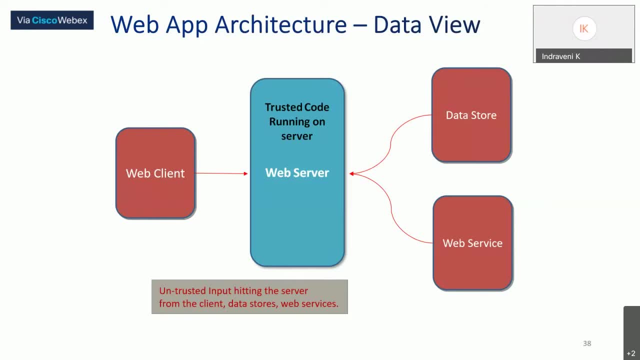 them are used as part of the address. if you start adding validation to not accept them, then you are so many complaints coming to you that your system is not accepting my address and not able to do registrations, so you are forced to accept everything over there. okay, now, if you are doing that, somebody inserts malicious content. somebody inserts a program. 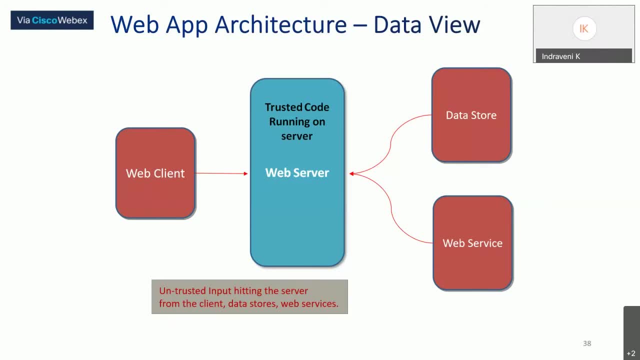 a script, a javascript or something which is harmful to the system into this address field. since you cannot validate and stop the code which is having special characters, you are forced to take the data as it is and store it in database. so there are certain attacks which are actually um, showing impact at a later point. it doesn't impact immediately. data store is done. 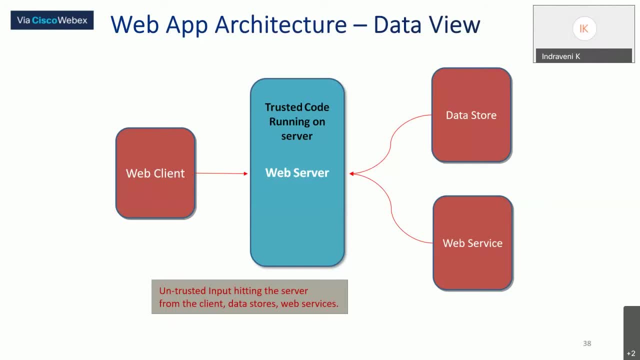 afterwards, when somebody reads the data, maybe an administrator is coming in and seeing all the registrations. at that point, when the registered data is loading in the system, that malicious code which is loaded by user is getting loaded in the admins page. so if you don't do validations, 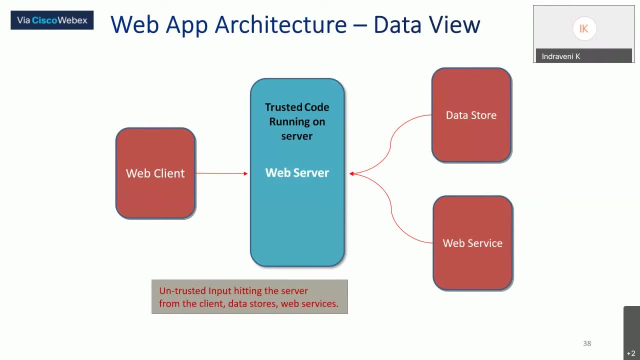 over there, which is coming from the database, the administrator user is getting compromised. okay, so i, in the end, if you have time, i'll try to show a small slide which can help you understand this concept, but all i am trying to show over here is, though, you are the one. 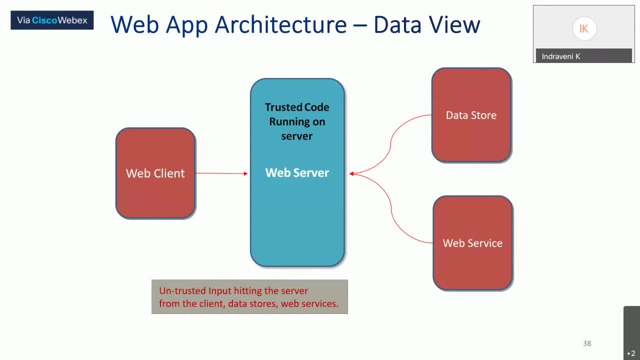 who is writing the content into your database. still, whatever data you are reading from the database, before showing it to the application, before showing it to the user on the browsers, perform validation and then show to avoid unnecessary attacks. as a developer, this is what we should remember: validation of every input that is coming on your system, because 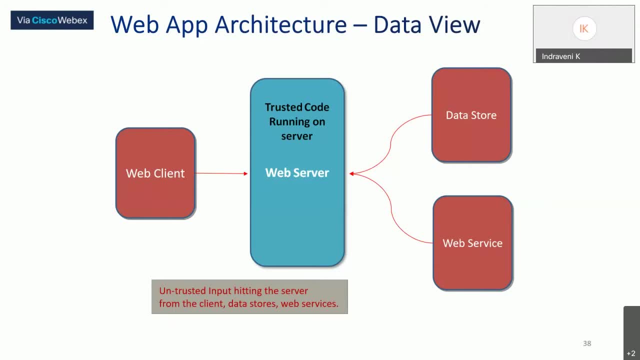 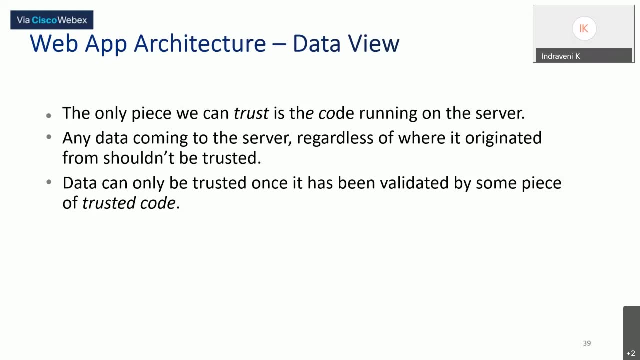 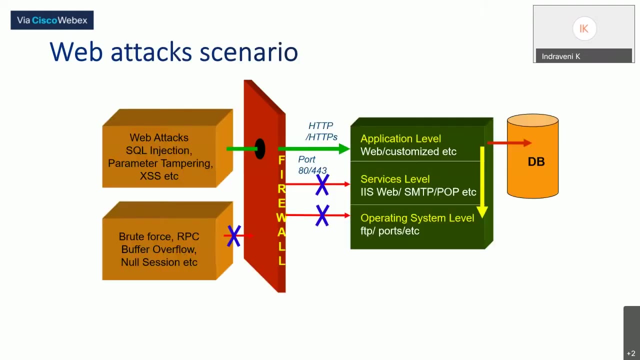 everything that's coming towards the system should be considered as untrusted. so the same has been explained over here. only piece we can trust is the one which is running on the server, and everything that's coming from outside should be validated. so yeah, why all these web attacks are happening? are there no security measures? 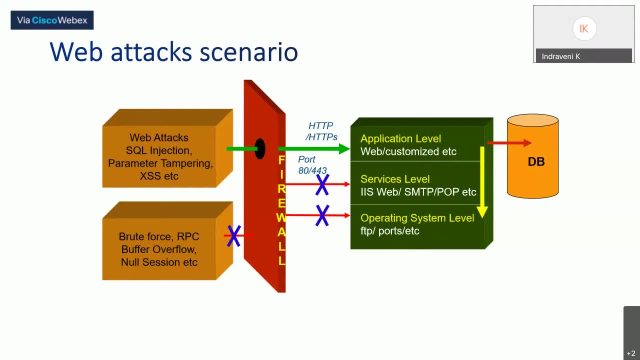 incorporated. you all must be knowing there are so many firewalls available. there are so many ids, ips systems available. still fire attacks are happening. when there is a firewall, what it can stop is it could stop attacks like good force attack, rtc, buffer overflow, null sessions, which are actually targeting your operating system or 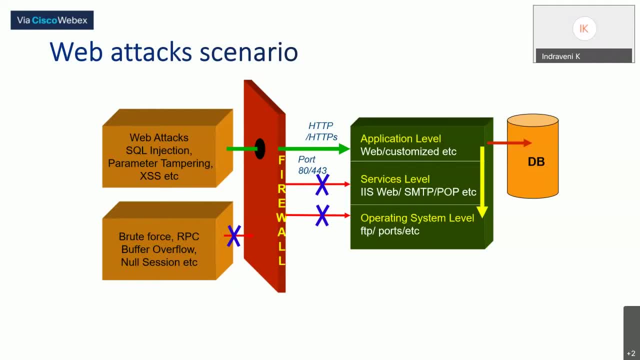 service which is running in your operating system on different ports. usually firewall tries to stop those codes- only 18- so that your application is served with a pump, and so the attacks which are possible on 80 and 443 are passed safely through the firewall and it reaches your application. attacks like injections, parameter tampering, process settings. 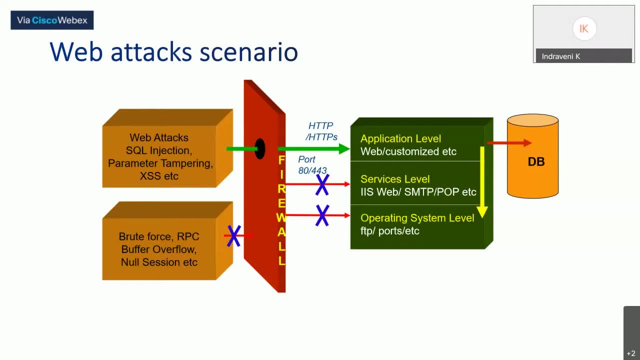 they reach through the firewall to your application. and in the application you can see there are so many layers over here. first layer is your actual code, which is having your application been running, followed by there's the next layer. whereas a web server is there, there can be a main server. 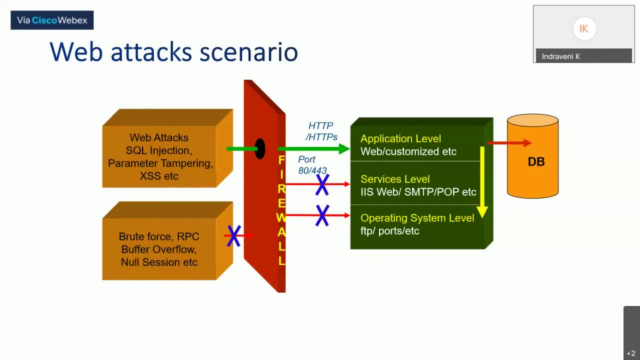 some services are there which are actually processing this input and there's an underlying operating system, the web attacks. the penetration of these web attacks is not only to the application. it can affect your web server. it can even create an effect on operating system and it can also affect 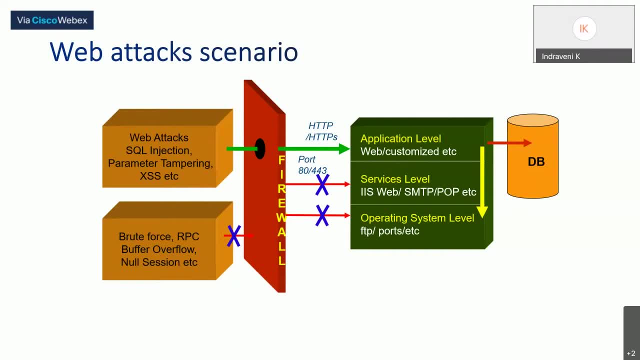 your database through a simple sql injection. you know, can you? through a simple sql injection one can even create a administrator user of the operating system. mostly when we say sql injection we think that okay, it can harm my database. if it is sql injection, it may create database, it may leak database. starting. 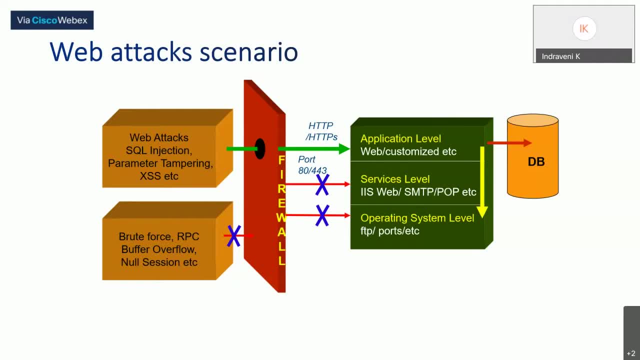 but no, it's not only with that sql injections, if the application is not developed properly. it can allow a user to create admin account in your operating system, windows administrator or a linux administrator. it can allow login into different codes. it can scan your entire network within your dmc docs using escalator. so many impacts are there, so these web attacks are not. 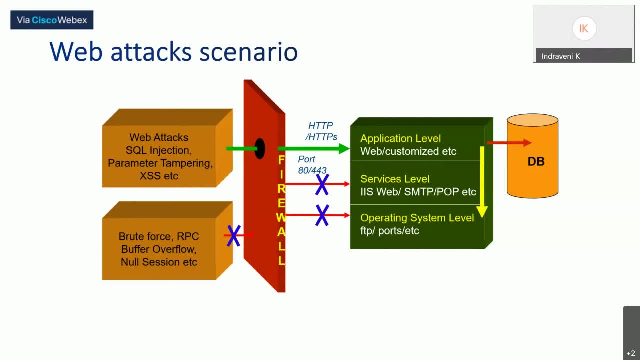 only with your application. if your application is not strong, it can affect the organization's network, it can affect the entire system and today people are hosting so many things on the virtual machines. one web attack affecting one virtual machine can affect the other, vms and other services running on. 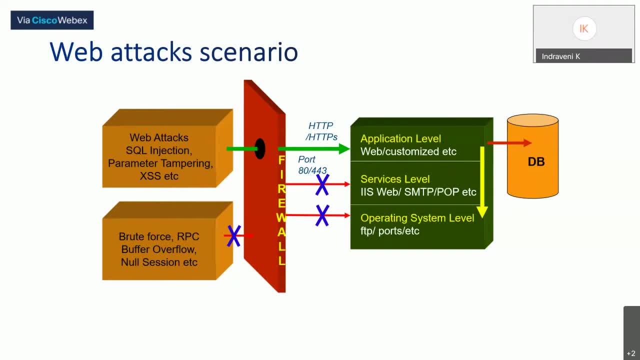 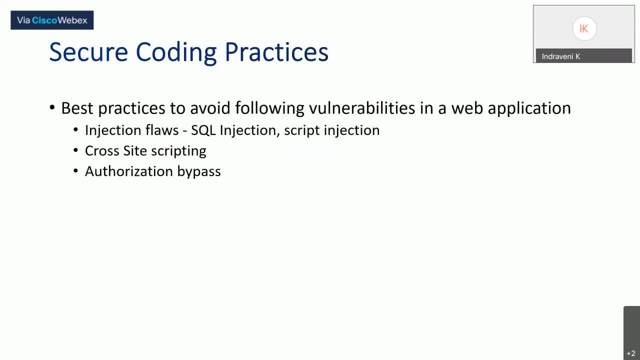 the system also. so implementing security application is very important, and we have seen certain cases earlier. let's start off with certain web-based attacks and their practices. so, first and foremost, we shall discuss about the best practices that we have to follow for this kind of vulnerabilities, like. 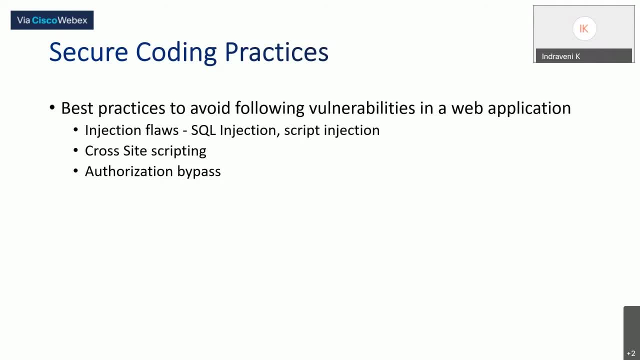 sql injection and sql cross first, which are most famous sql injections, script injections and many more. then we will discuss on how do we stop the cross-site scripting attacks and we shall also discuss on the authorization bypassing. how do we um stop authorization attacks or session based? 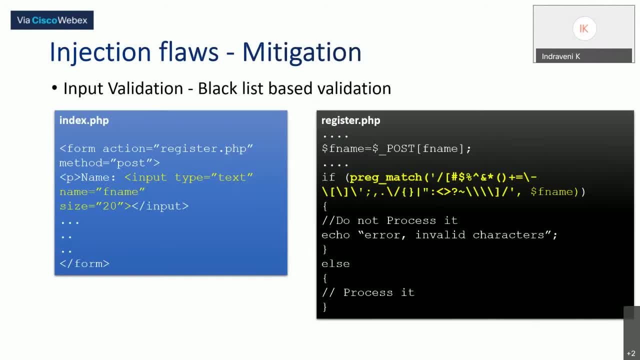 attacks on the systems. actually i'm not putting much of the theoretical, i just tried to put direct because all of your uh students, all these wordings you may be knowing descriptions what it is or not. that's why i'm just trying to show you the code. when we are saying injection flow, injection flaws, 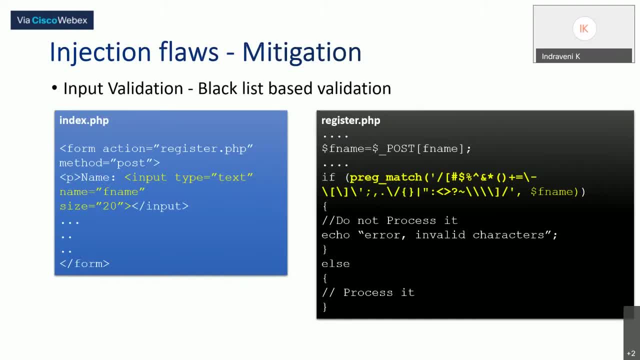 are mostly about the validations and in the session- this session also- from the beginning, i have used the word validations, validation, validation. you must be thinking: validation. you are doing very good and, yeah, we discussed validations. you are doing the javascript and html file. that is also good, but javascript and html file are not sufficient. that's what we understood. 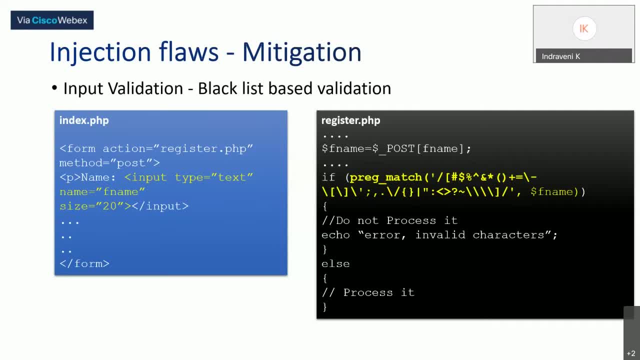 now, by this time. now, if javascript validation is not sufficient, what should we do? we discuss that also. we have to do server side validation. it's not the client server. client set validation only helps us to provide usability to the user who is filling the power of our data. 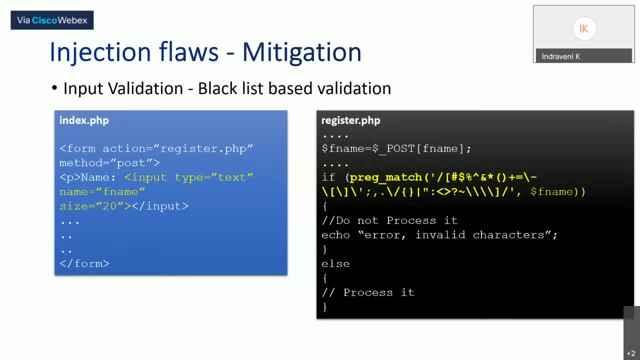 but server-side validation only stops the web-based methods. you do server side validation. what is the best way to do the validation is what we will discuss. i hope you all know what validation means. i'll just in one sentence. i'll tell again if somebody is not able to follow. validation is something that you are trying to look for, what you require. 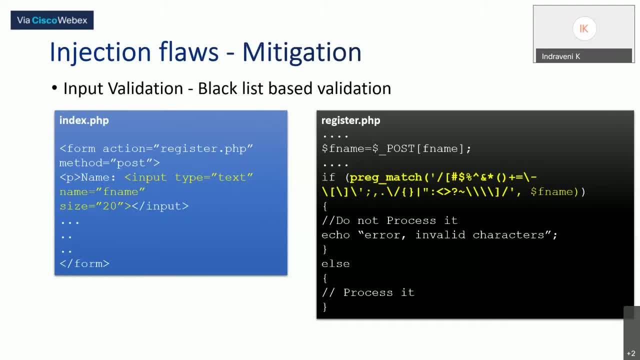 what is required by your application is coming in the field or not. you could fill or not, say, pick up this example itself. in the left side blue box you can see there's a form with action register, dot. bhp, and there are certain form fields over here. one of the field is name and the yellow 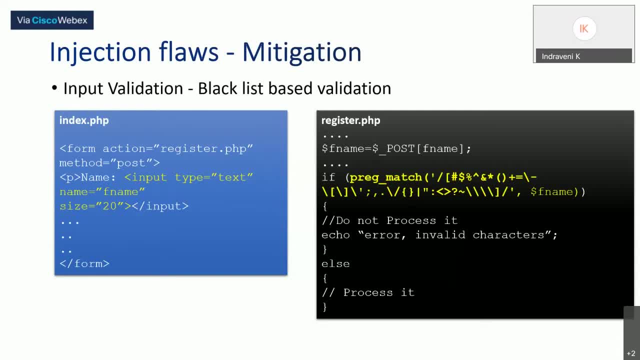 font. you can see this is an input param. input the html tag type text name is f name. so if someone enters any value in this particular input field, that is the field name you are going to see is been sent to registerphp as a post parameter, because the method is post over here Now, when 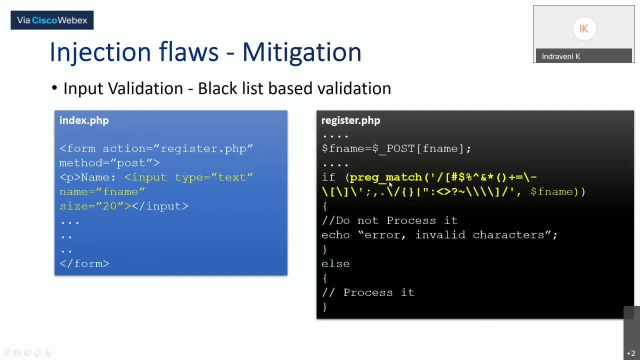 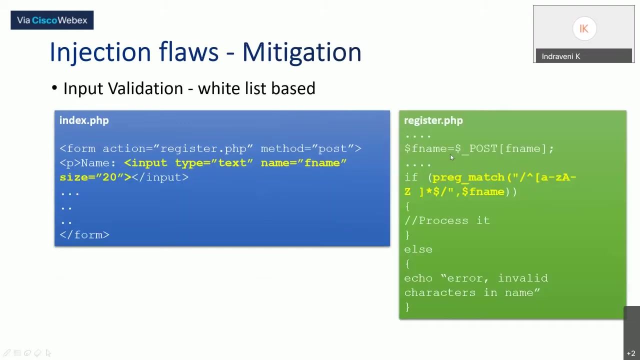 this value is coming to registerphp as a input data. we have to see that this value, fname, is having the content that what we required. Now I have come to registerphp. you can see in the right side black box. fname is equal to post of fname. So I am calling the post. sorry, the post. 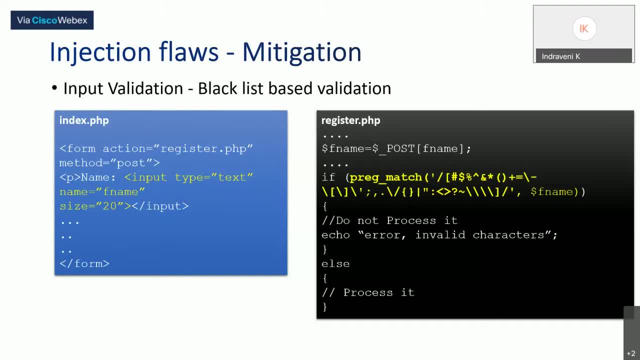 parameter fname data into this variable fname. I am sorry, I have taken an example of php over here. I did not tell about that. So the same logic, see php, you just worry about, don't syntax. you don't worry about the syntax, just think about what logic we are discussing. model This logic you should. 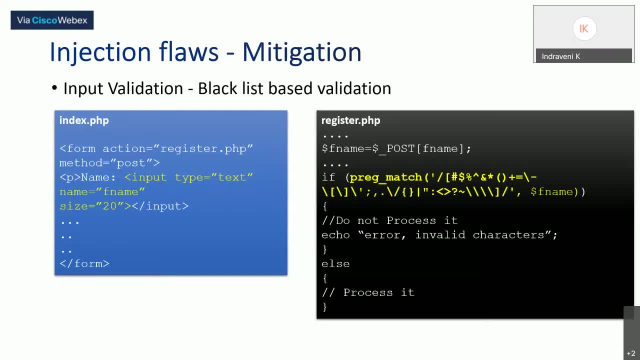 implement with whatever programming language that you are working on in future. It can be java, python or anything. Php example I have just taken for reference because it is an easy language to understand in the plug-in English. Okay, so try to take in the logic as soon as you see php. don't. 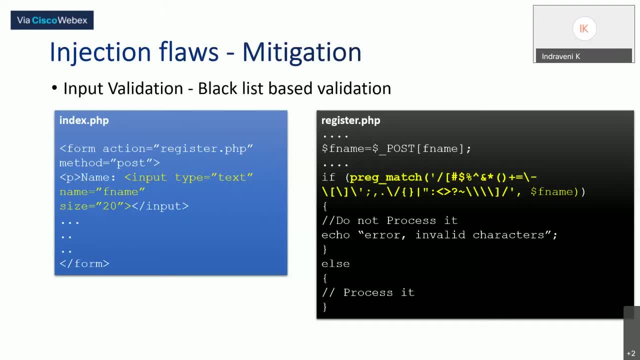 just think that, okay, this is not my cup of tea. It's not like that. it's only an example. take the logic Now. I am taking the post parameter fname, I am taking that into the variable called fname and then we are writing the function if condition. It's a simple if condition. 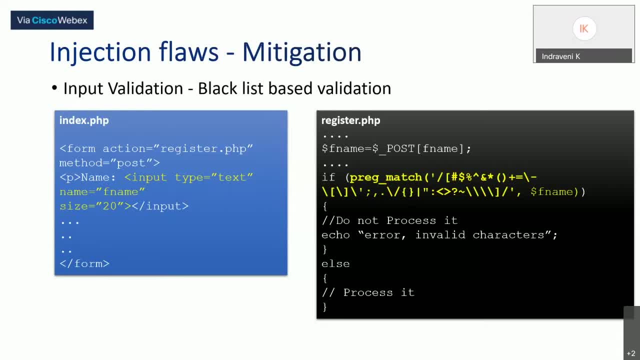 With a regular expression. we wanted to see whether this fname value is having any unnecessary content. So input validation means what, given any field, we should see whether that field is having the content which is required by the application or not. So name is generally. when I want a name. 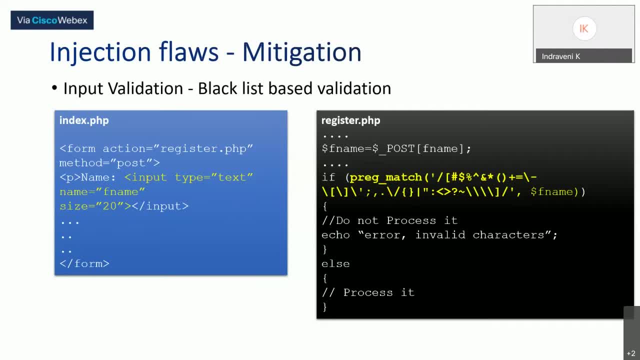 to be taken from a particular form. as a developer, I want somebody to enter their name alone. I don't want somebody to enter numbers over there. I don't want someone to enter some garbage value with exclamatory hyphens, single quotes, all these values, because that will. 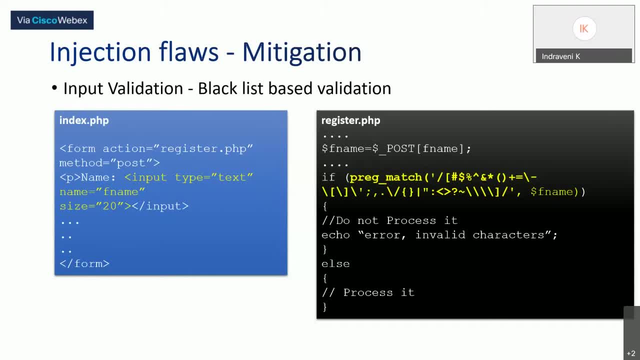 unnecessarily create wrong information in my database and it may also disturb my application flow. So we try to put validations and if your validations is not correct, this special characters can lead into performing attacks like sql injections, crosshairs, scriptings and what not. That's the reason we are saying we should do validations. 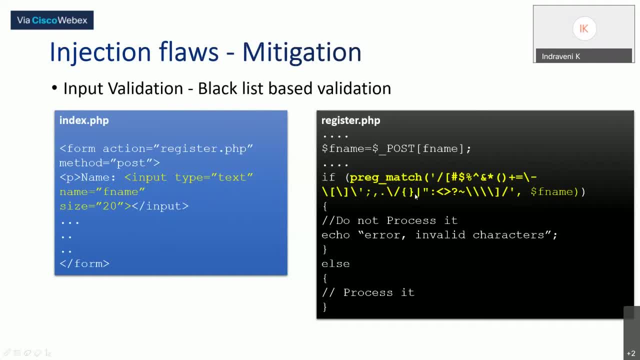 Now, in this case, what we are doing over here, the in the black black box, yellow colored font, you can see. this is a regular saying: that the variable fname if it is containing any of these special characters that are written within these codes, single quotes if it is having any of these. 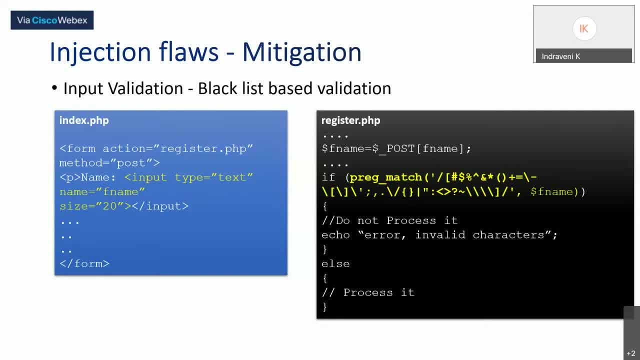 then do not process it. I want to print invalid characters you have entered. If it is not having any of these characters, then I want to process it. Okay, this is one type of validation. This type of validation is called as a blacklist based validation. It means I am trying to put a 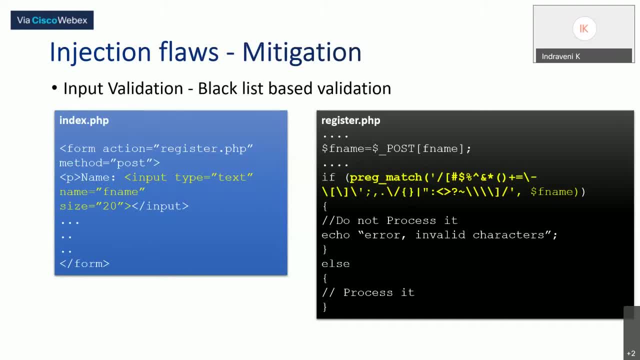 list of blacklisted characters to check whether it is there in any given variable. Okay, so this method is called the blacklisted based validations, wherein I am trying to look for a special character in a field. If any special character is there, then I want to stop that. 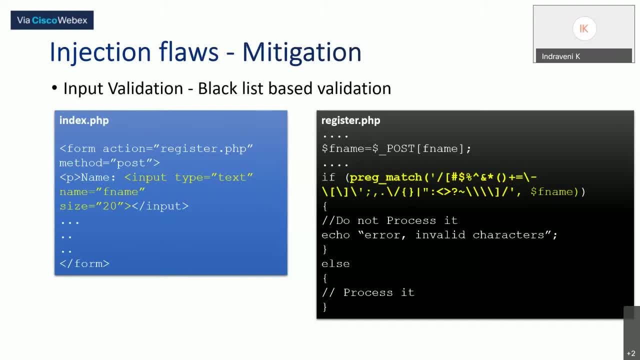 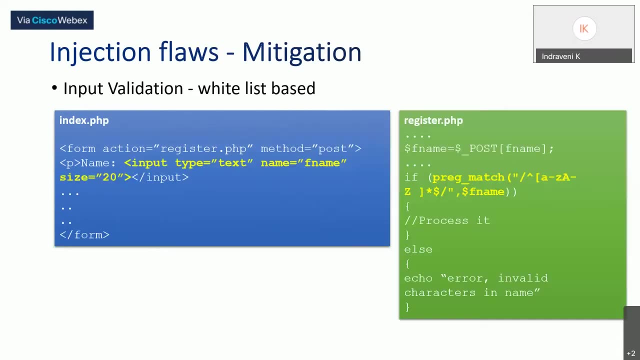 submission or form submission. If there is no such special character in that variable, then I want him to allow him. That is what is the logic that's written over here. This is called as a blacklist based validation. Few developers follow this practice. Another practice of the same code is: 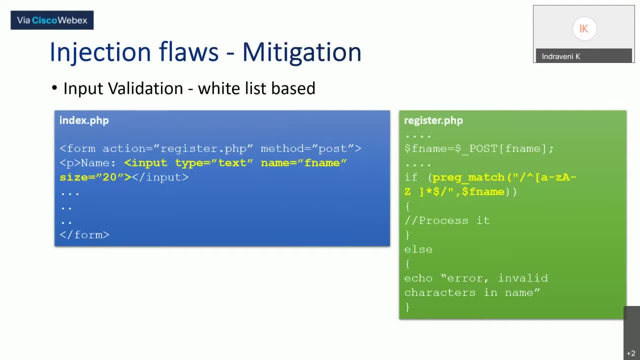 using whitelist based validation. The same form in the left side and in the right side you can see the green box, again a yellow coloured font over here. Here what we are doing: we are trying to see whether my fname variable is having values a to z, so a to z, a to z and a space. 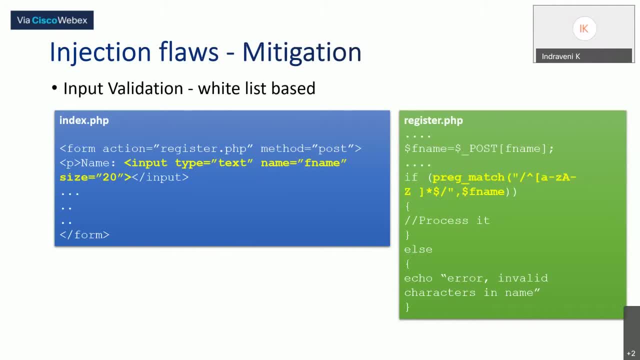 Any of these values are there in my variable, then allow him Else, stop him and say invalid characters are found in the name. This procedure is called as a whitelist based validation, where we are comparing a particular variable or a field value with a set of variables which 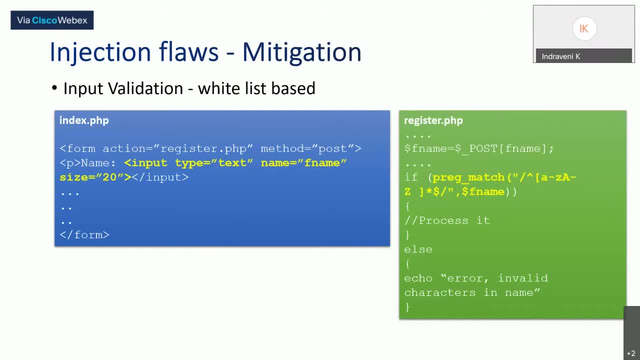 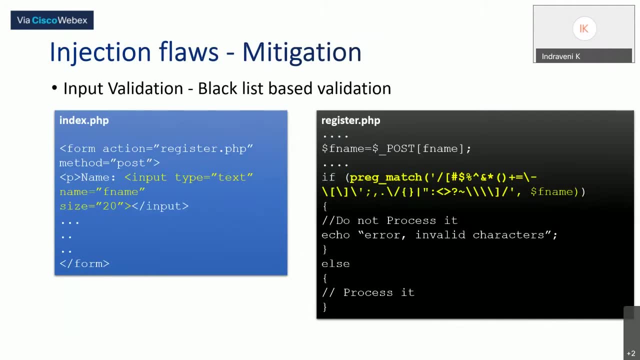 are actually allowed or required by my application. In the previous case, I am comparing with a set of characters which are I don't want in my variable. So these are two types of validations. Few developers use that method. few developers use this method. 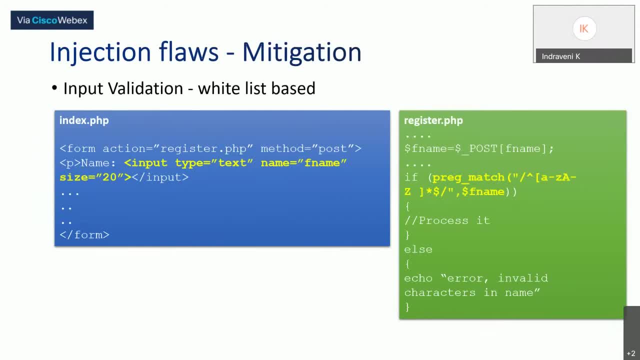 But both are doing the job of validation only. Our intention is to stop a user from entering unnecessary character into a specific variable, So this is what is called as input validation- Any given form- and what we are writing is in PHP, So it is a server-side programming language. 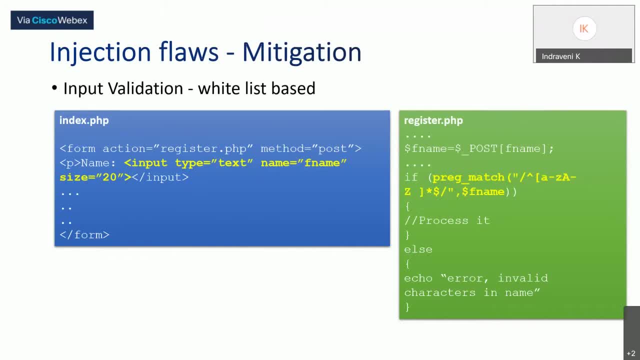 So if somebody does any kind of a tampering and try to inject special character in the form field, then your registerphp wakes up. It tries to show that no, you are entering the wrong value. That is the advantage of having a server-side validation. 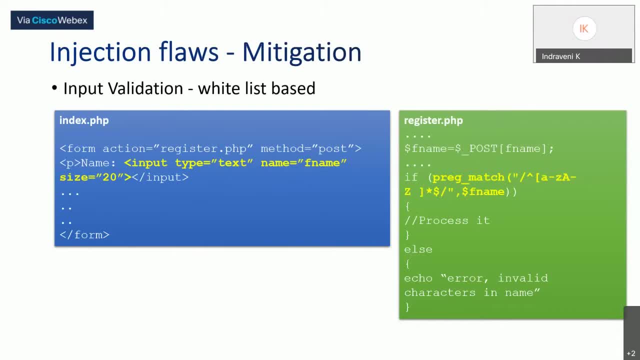 It will stop our unnecessary characters or data coming in, even if somebody bypasses the JavaScript or HTML5-based validations. So I hope you got a picture of what is the difference between these two types of validations and what validation is doing and what are the different types of validations. whitelist-based. 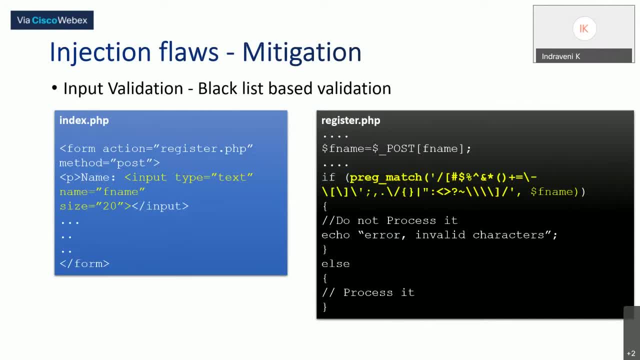 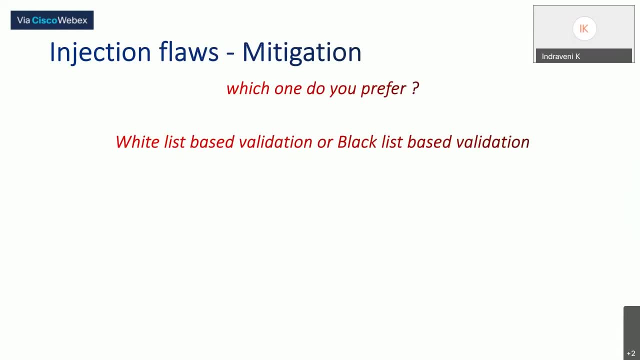 validation and blacklist-based validations. So let's move on. What is the best method? Both are good, Both are doing the validation job. Implementing anything, it would definitely solve your problem. It would definitely stop unnecessary content coming into the system. 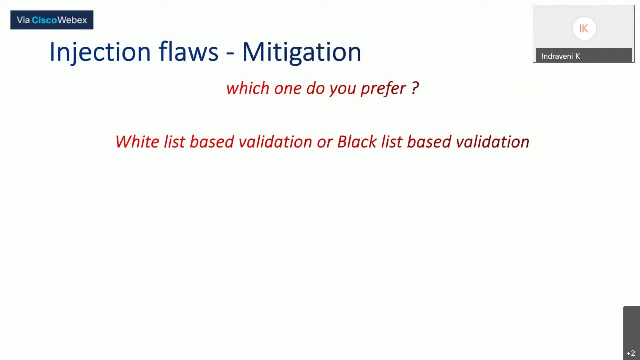 But we want to go with the best practice. Best practice is: what if two options are there? among these two, which one is good is what you should pick up. So, according to you, based on this logic, which one do you prefer, whitelist-based or 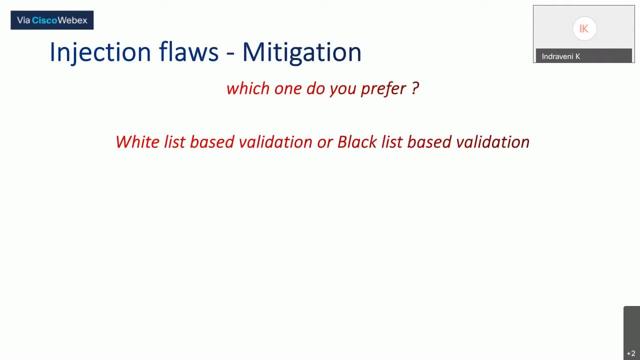 blacklist-based. Maybe you can type in the chat box your answers. However, I did not stop with the answer. Somebody said: blacklist Is my voice breaking. still I could see a lot of messages: Voice is breaking. Those are old messages. 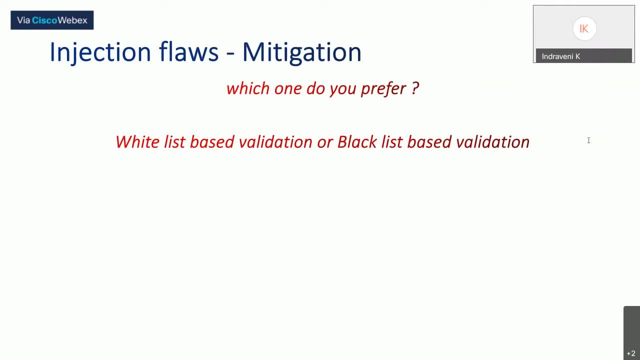 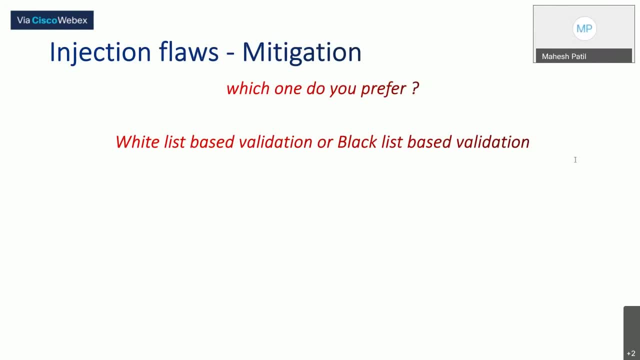 Okay, fine. So yeah, many people are saying whitelist-based, blacklist-based. For me I think blacklist is nice, Blacklist is nice Good, Good to see Many people are choosing. So I could see among the chat answers are 50-50 and both. 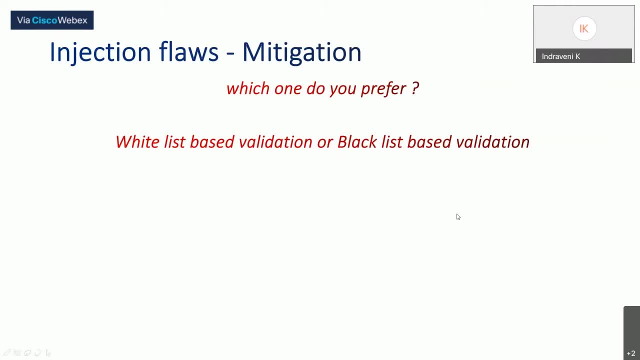 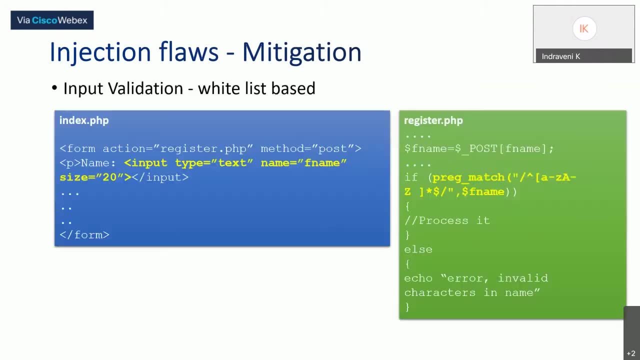 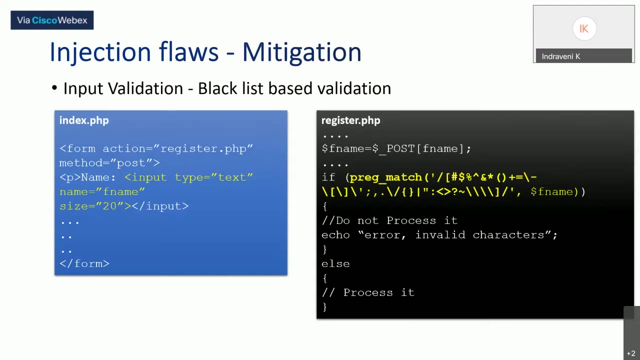 But a general security practice is to use whitelist. Why whitelisting? Now let's just go back to the previous slide, Why we are saying whitelist, Why I am saying whitelist. saying why I am saying whitelisting is say: by any chance, you forgot to add a character. 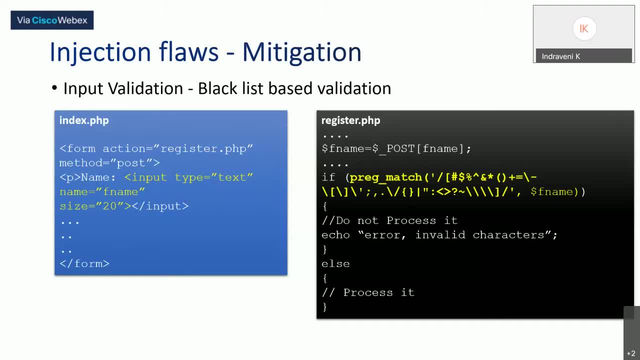 like a single code in this particular box. We are just typing, right. you may do copy paste also many a times, but most of the time, even in the first type, when you fill up a set of blacklisted set of characters, when you type, if you forget any specific character, what? 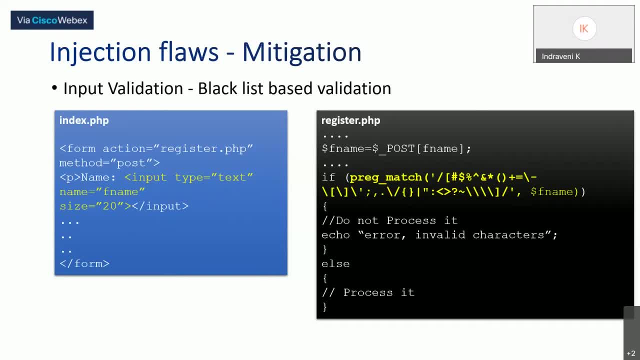 happens, those character based data can come into the system. Second thing is, whenever there is a new attack coming into picture with the combination of characters or data, particular, unfortunately if a new character itself is coming to the keyboard, like I say, there is a new rupee symbol come out now, today, these days, a new Indian rupee symbol came. 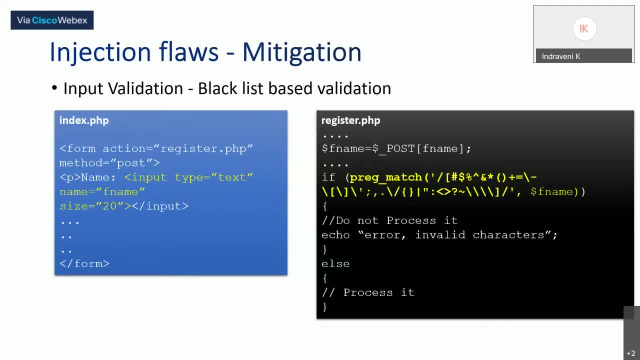 in our keyboards. similarly, what if some other new character comes into the English language itself? some other character comes into the keyboard itself? we need to come back and change our code everywhere where you are writing a blacklisted characters. I want to blacklist a new character. I should come back to my code and keep changing my code everywhere, wherever. 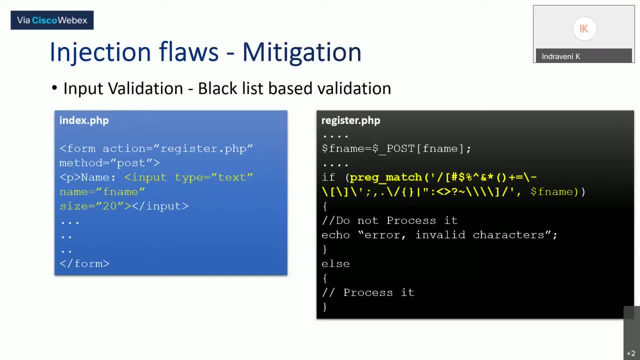 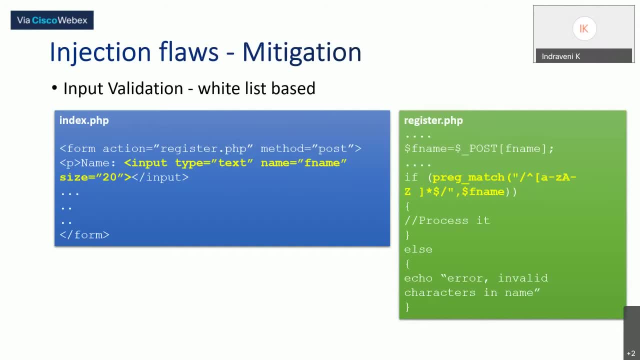 I want to stop that particular character, but if you are known that what you want and you are accepting only that whatever is there in the world is blacklisted, for me, what I want is A to Z and a space. Why should I worry whether it is having numbers 1 to 9,, 0, special. 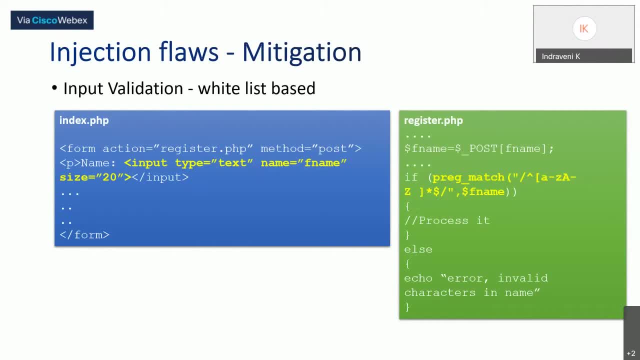 characters, Arithmetical numbers. so many things are there in our keyboards, right. why should I worry about which all things I have to incorporate into my list? If I just worry about what I need, I will take rest. all is not my cup of tea. then it is very easy for the programmer. 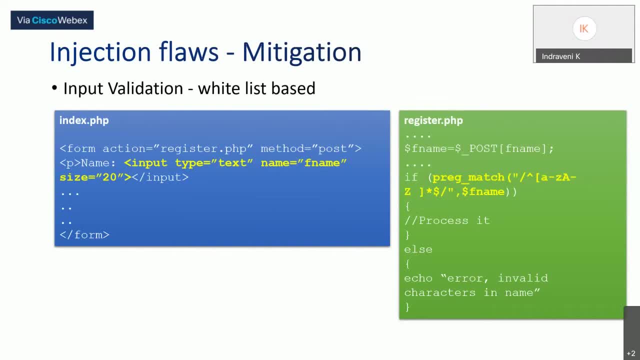 as well. you do not need to go back and keep changing your code every time there is a new vulnerability coming into picture or something coming into the case. So it is always a good practice to go with white listed where there is a blacklisted character. 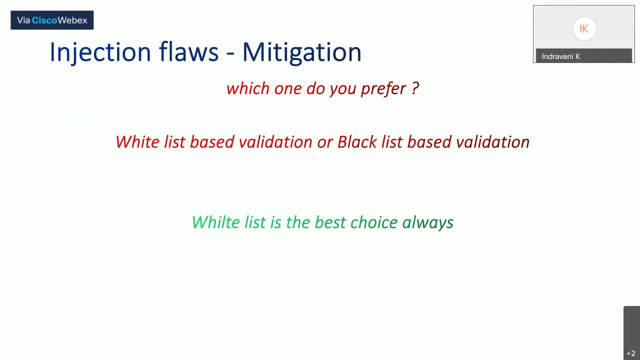 You know what you actually want for your application For a name. you know you need alphabets for a phone number. you know you need digits. Many a times you can just put apart from 0 to 9. if you find anything else, you just drop it. It is easier, right, rather than you putting. 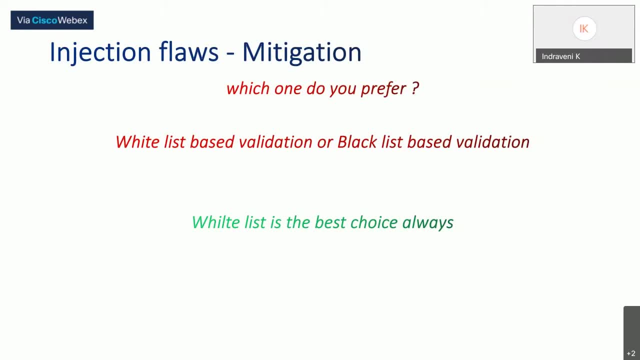 alphabets A to Z. I want to avoid. I want to avoid so many numbers, special characters, braces, single quotes. it is a long list, So that would be easier for us. it is best to have a white listing. So this is the best thing. only validations, only for stopping any kind of these attacks. 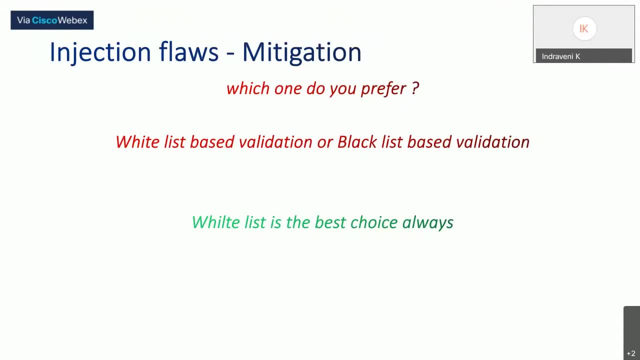 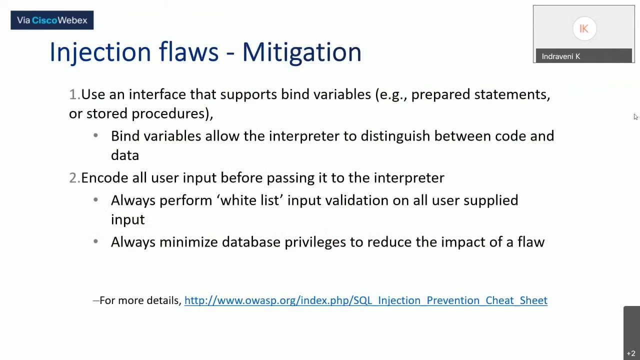 I hope you understood why we are saying white listing is only the best, because that would reduce our headaches at a later point and it will not ask us to go back and keep changing the code every time there is a new vulnerability seen or something. So this is just an overview. 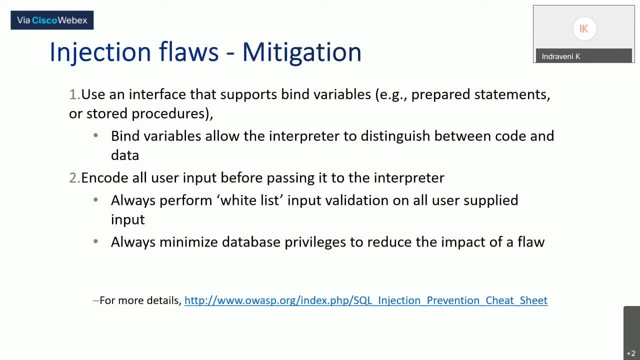 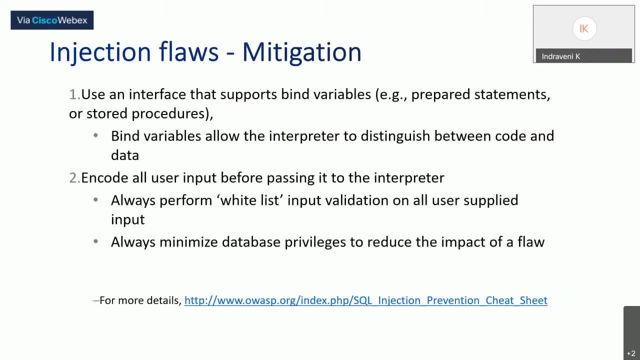 So this is just an overview of what mitigations we have to do for injection clause And to stop SQL injection- I think previous to stop SQL injection based attacks. apart from all of these validations, when you are interacting with your database from your application, you should use prepared statements or stored procedures, kind of things as something that. 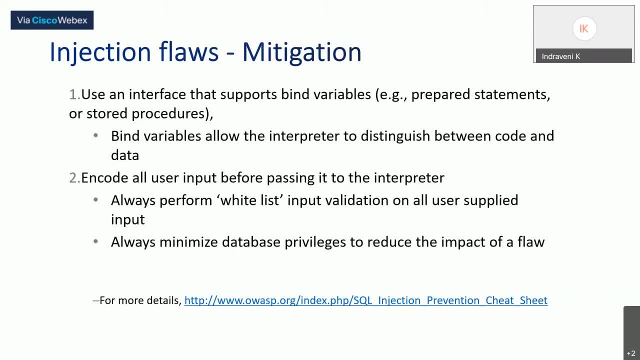 pre-compiles the query. it should actually separate your code from data. that is how you have to choose to interact with your database from the application. So that is the first thing. So this is just the first thing. So after that we are done. 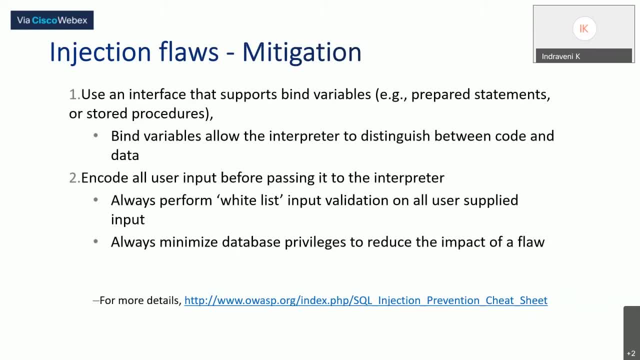 Thank you. this- the SQL injection attacks, can be stopped to an extent, though you do. validations using prepared statement is an extra layer of validations security you're adding to your application. bind your variables to your application such a way that there's a distribution between the code and 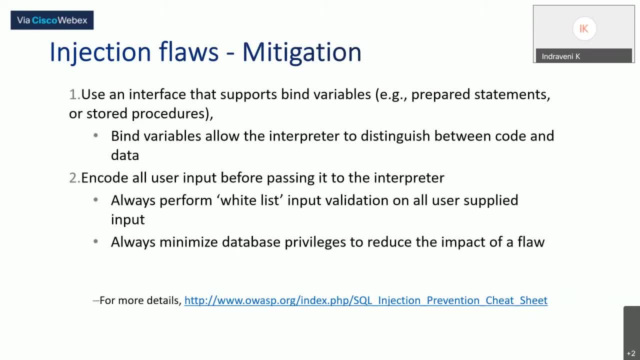 your data. second point is what we have just discussed: encode all your user inputs before passing it to your interpreters. always perform whitelisting based input validations and always give minimal database privilege to user access to your applications. you will have an connectivity line in your programs, in your applications- database connectivity where you say your. 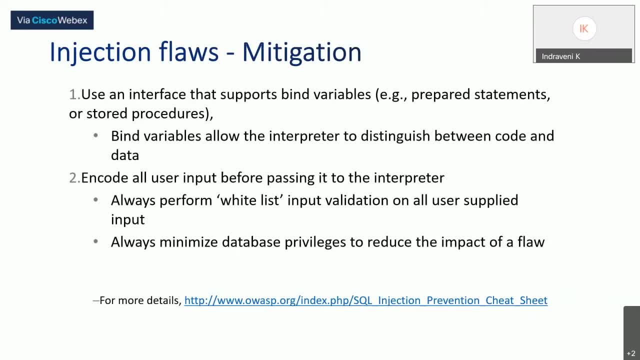 application should connect to which database, using which username, using which password. remember in that point, try to remember: do not ever use the root privilege database user if it is a MySQL root, if it is a Postgres SQL, if it oracle tiger score. this kind of default and the super privileged users we should not use for our 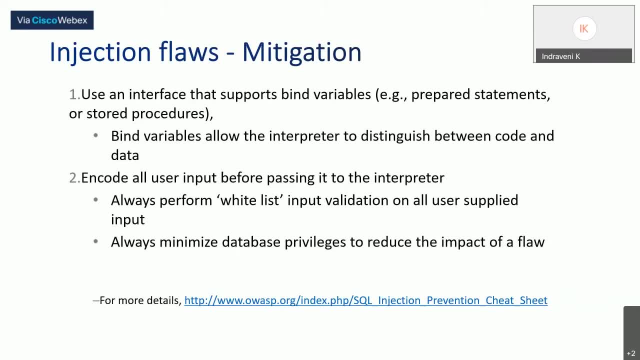 applications to connect to this database because any attack that comes to the system will create lot of impact, high impact on the database. if you are giving lesser privileged user with minimum roles like select, insert, delete, allowed only user, you should create a separate user and that user should be used to connect. that will reduce the impact of affecting the actual core system. 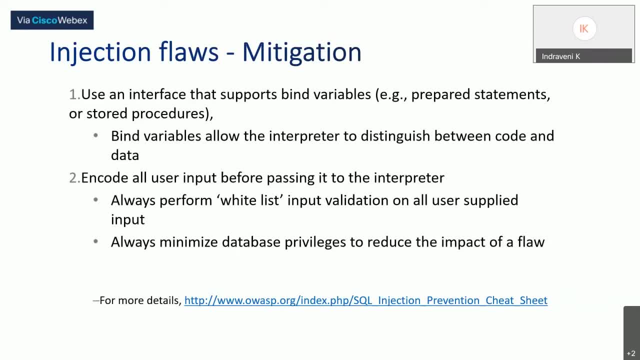 as we were discussing, injection attacks can create os level users and all also. so you should be careful enough to give least privileged users only access to the systems. and here i have given a link for sql injection changes. so the same page is having a bigger, same reference. you can. 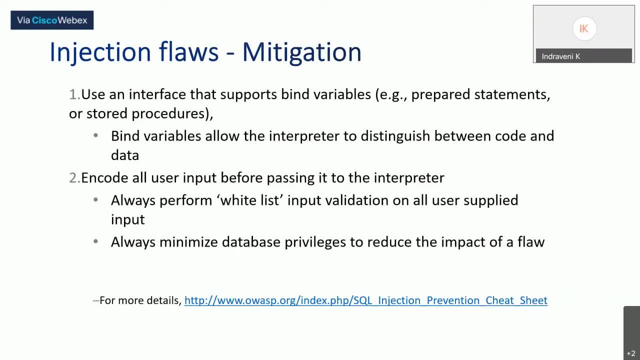 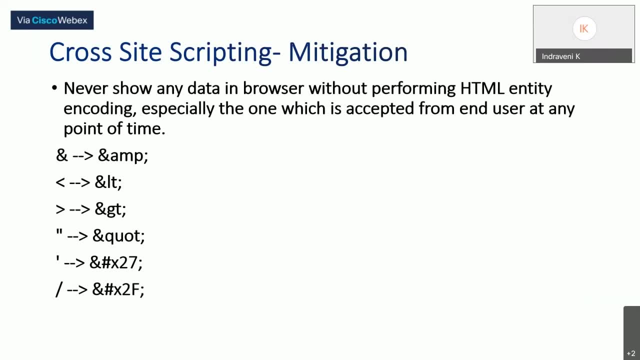 see complete cheat sheet for mitigating all types of attacks related to injections or so on. moving towards the next vulnerability: cross-site scripting mitigation. cross-site scripting: basically we are not. i'm not detailing here, but it's something that through which someone tries to introduce a javascript code in your application which can create attacks like 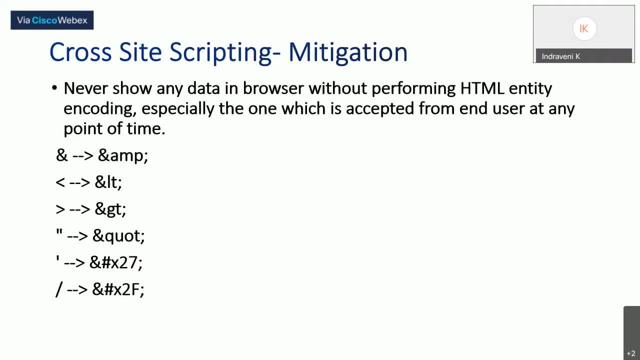 either hacking cookies, redirecting your users- your genuine users- to phishing websites, making them victim to various cyber frauds, something like that. if you want your application to not have cross-site scripting kind of attacks happening on your system, then what you should do is never show any data with the browser without performing html entity. 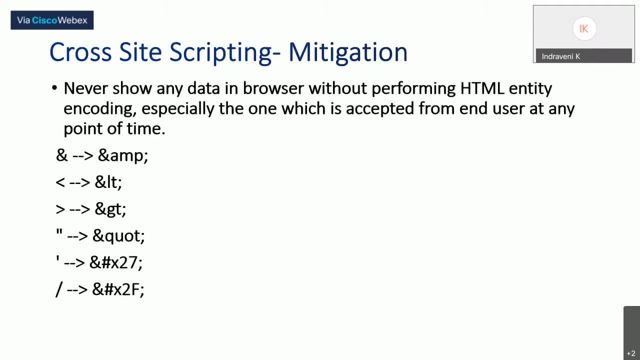 encoding, especially if you are accepting that data from an end user at any given point, maybe today, maybe before or during registration or sometime. okay, so how do? how do? what do we do? is it's called a html entity encoding. you can see in the bottom over here listing 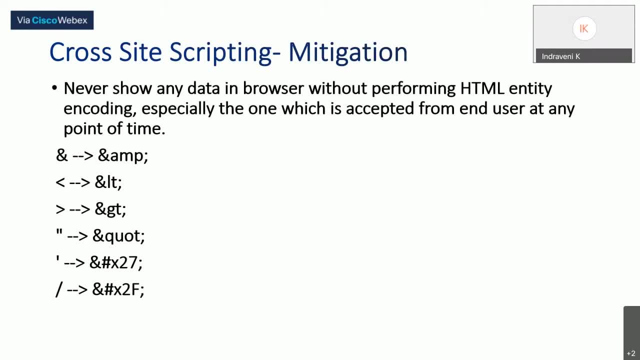 if there is an ampersand, you should write a logic to convert ampersand to dark ampersand: amt semifinal. if there is a less than symbol, you should convert into ampersand: empty semifinal. this conversion should be done before you show the data to the browsers. then what happens? the this: 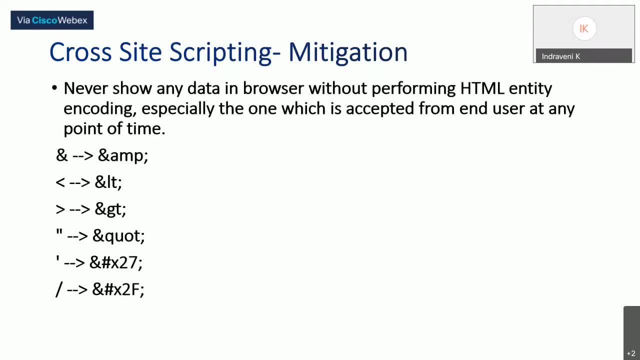 these characters would be considered as a text rather than making it part of the code because, as i said initially, browser has the capability to execute a javascript code. as soon as it sees the javascript, it will execute automatically. it doesn't know who sent it, where it has been said, whether it is genuine or not genuine- nothing it knows. it sees a javascript. 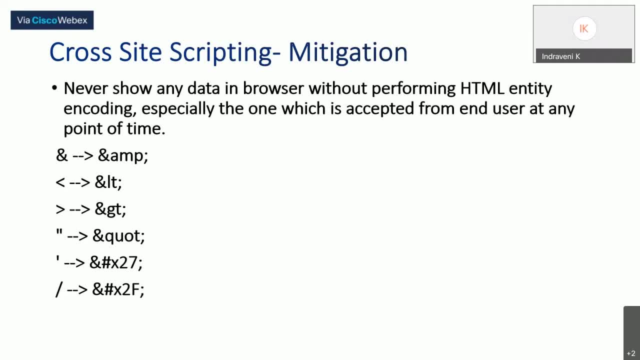 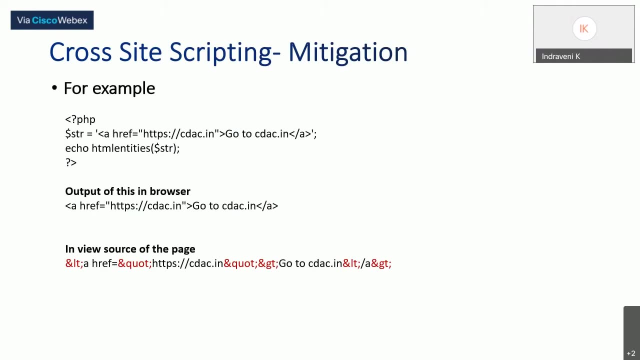 code it executes okay. so that is the reason to stop. cross-site scripting is related to javascript, especially any kind of client-side coding injection into the applications. a simple example is available over here: the mitigation technique. this is again a php example. i'm just having a variable string. 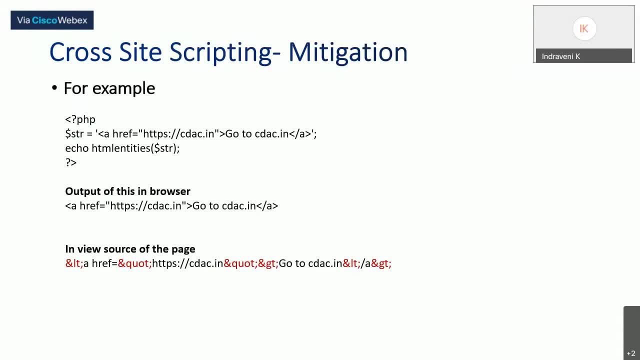 with a href sedagin go to sedacin. i just wanted to show this content in the browser, so in the echo statement i am adding a function called html entities for the variable string. when you, when we do this html entity string output is filled with a string. 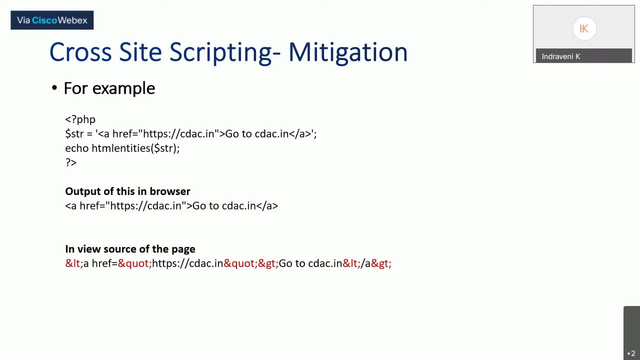 and we'll call it. i'll call it a varistring. when we do this, html entities string output is a string. types output is the string and input is the string. the browser would be something like this: ah, so it's. if you go to the page source and see this, 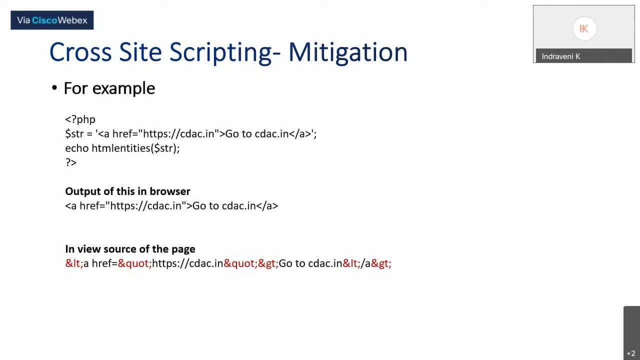 is how you see the pages. whatever i have marked in red are nothing but the conversion that has happened on the input of the string data. whatever is there, wherever less than symbol, greater than symbol, are all there. they have been converted in this form. that is the reason this is shown. 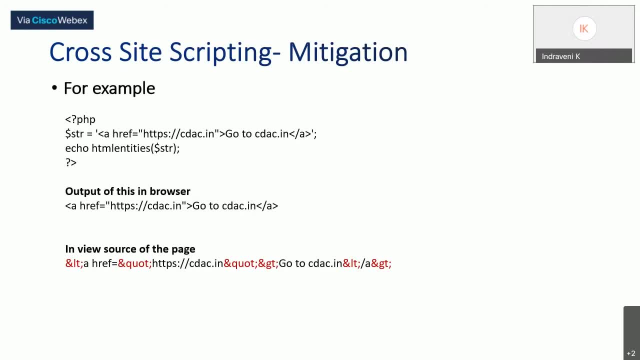 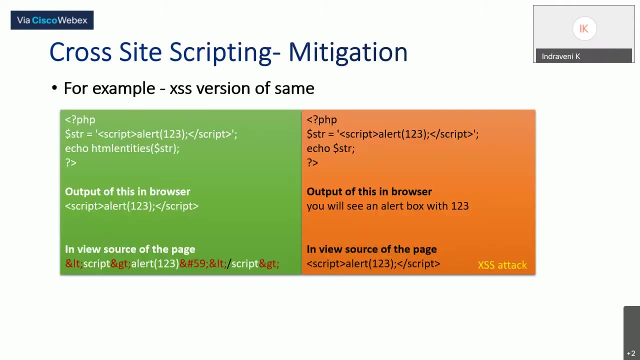 as text in the browser. you may be thinking this is a simple html. what is wrong with this? on the browser it isck att artwork layout that is presented with the짢x, the latest new features that have been implemented in text. they are trying to understand how the 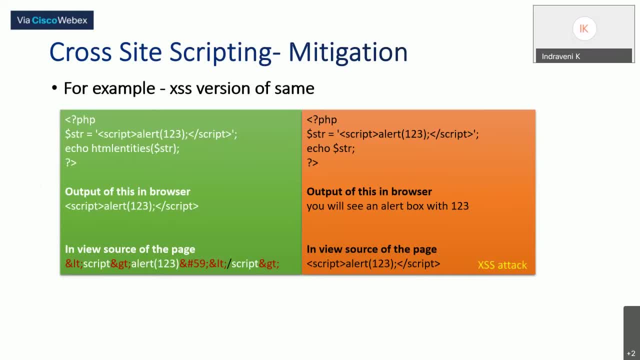 special characters are getting converted. before showing the browser, now let us take an example of- is how it shows. whatever is shown in the green box, you can see the in browser, you will see script alert one, two, three and if you see the page source, you will see ampersand, ld, semicolon and all will. 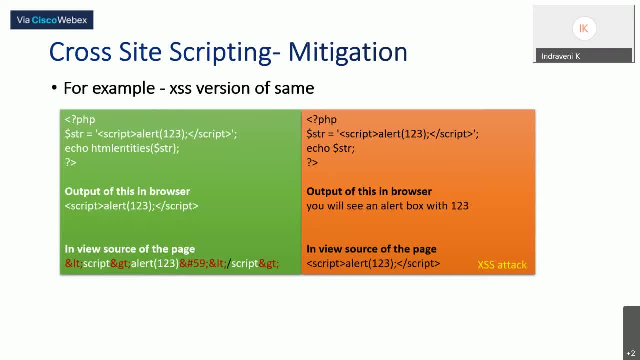 replace, but with the same code, without calling this html: entities function. if i'm going what happens in browser, you will see an alert box. you won't see this code because for browser it is a code it executes. if you see the page source of this browser where you see alert, alert message. 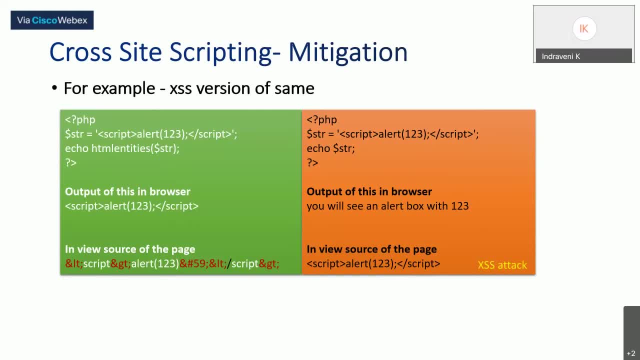 you can see in the pages, the code is as it is: script. since there is a script attack browser knows that it should execute, so it executes. so the mitigation for crosshead scripting is: you should always perform html entities encoding technique so that any special character, if at all, 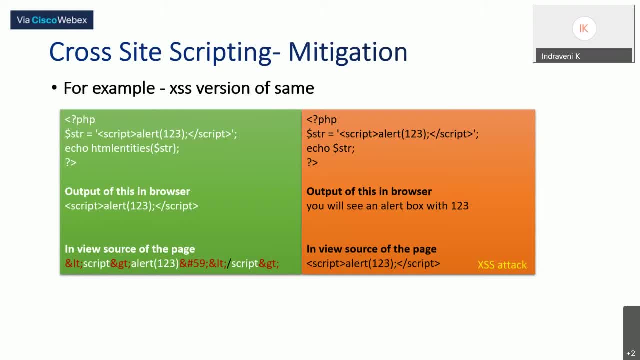 by mistake, though you do a lot of validations by any chance, if somewhere of the other it is coming in also by doing this kind of html: entity detection, entity encoding the special characters get replaced with this html encoding encoded characters, and thus the browser would not execute it. the browser considers that to be text. 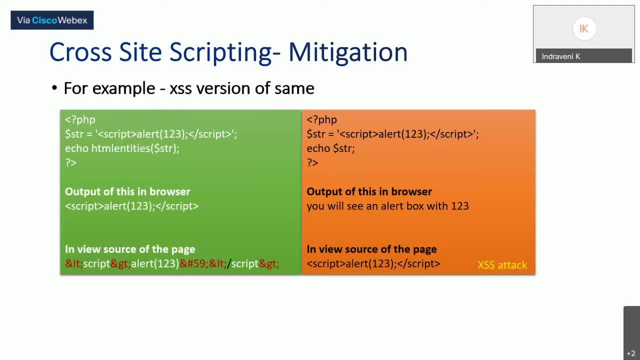 it won't consider that to be a code, and so the attacks like crosshead scriptings reflective, or it can be stored or it can be dom based. also any kind of things wouldn't get executed. that is how the crosshead scripting attack can be mitigated. 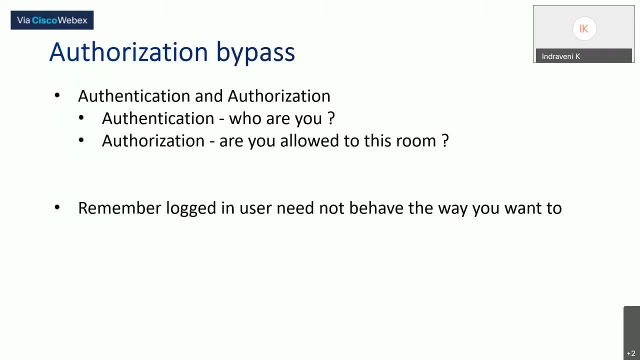 is it clear. now, moving towards the last topic, authorization bypass. so authorization bypass is something which is related to the sessions. basically authentication and authorization. these are the two things that you should know, always being a developer. so authentication does not have to repeated signageruktur for those teams. so, as we discussed also, 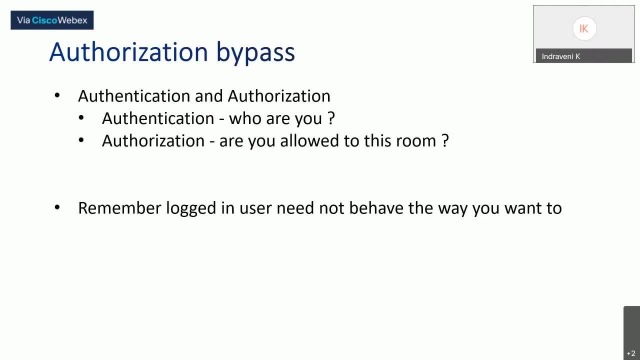 key business στο you are civiliyor is the user's identity. that generally asks the users who you are. so who you are is answered by entering a username password. so we know that this is the users identity. user username and password is received. after that, what happens? are you allowed to this particular rule? are you allowed to access this page? is what is the authorization means? so first is: 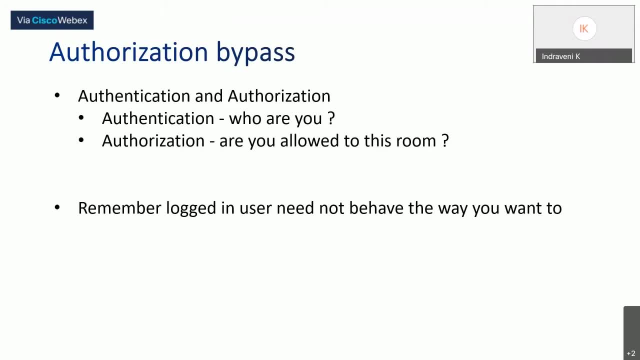 space of this application or not. that's all. now there are so many attacks related to authentication bypasses also, authorization bypass also, but authentication bypass attacks- most of them can be addressed by doing proper validations and all these things. authorization bypass is something related to the logic that people implement in their programs. that's why i've thought of putting 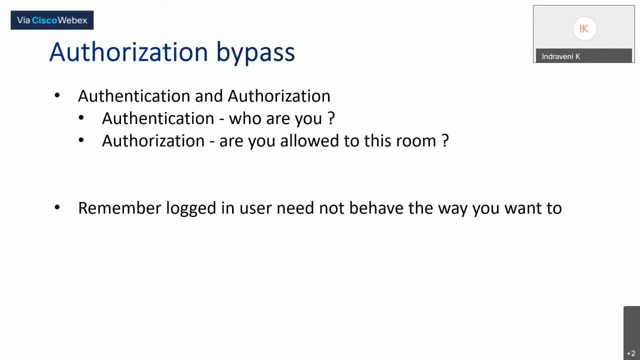 authorization bypass as one of the key points why we are stressing this is the reason- is logged in, users need not behave the way we want every time. once the user logs into the system, he can click anything, he can tamper anything, he can change anything in the url, whatever he can. 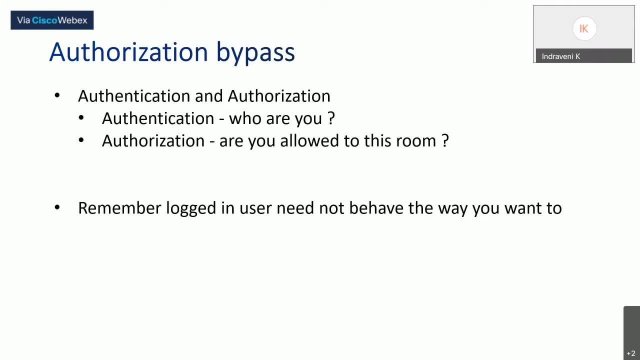 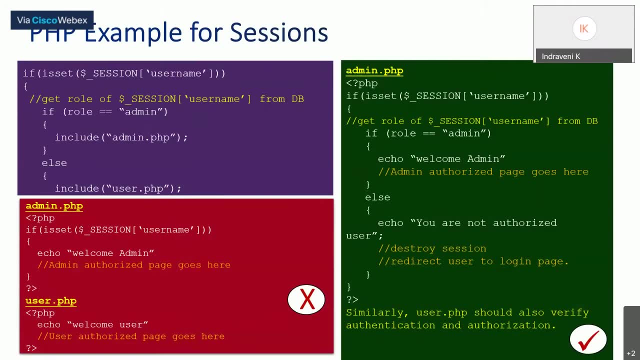 do this, so logged in users can behave differently. for this, here i'm showing you a simple php example and a scenario of how authorization bypass happens if a code is wrongly written. so let's go block by block. you see the first block, the purple color block. what you see here is about- uh, this is the first page- where, if a session 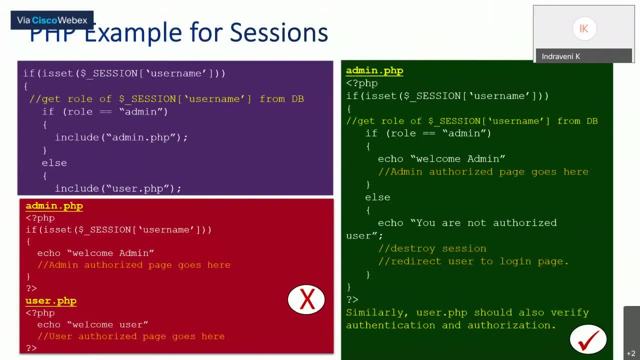 is of user us. if a username session is available, that means a username session is there, means what user have logged in. a session id has been assigned to him. after his credentials are being verified with application, then this variable session of username is set as soon as this variable. 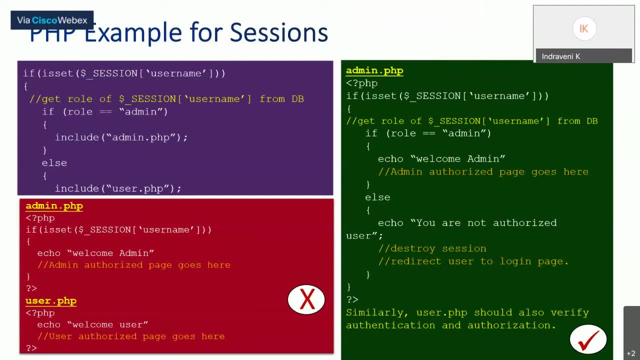 is set for an application, it means that okay, authentication process has completed successfully. he has come to the next page. now, after coming to the next page from the database, we do a check whether this user is role, is administrator or not. we do that entire. whatever i wrote in comment or 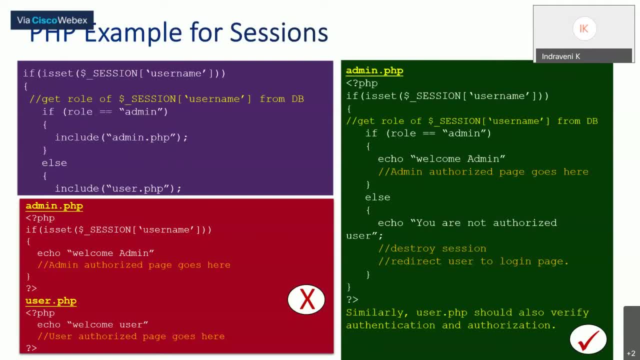 over here is about a logic that we should write regarding the database character. you call a database query and see whether this user's role is admin or not in the database. as soon as you get the role you verify over here hardcoded role is admin or not, i mean fine, if it is administrator, i am. 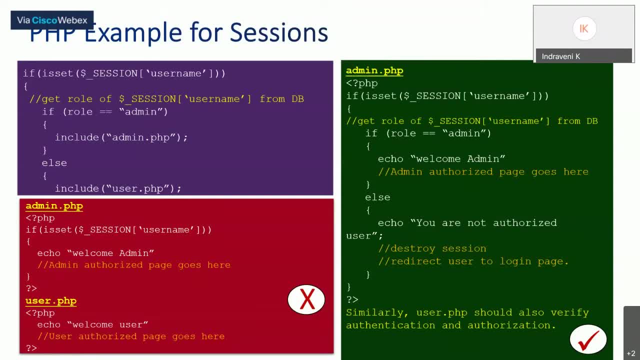 trying to call a page. if it is not administrator. we are calling a page of userph. this is the logic that is there in the first page. so after session is valid. i see the role. if the role is admin, then i'm taking into respective pages. and now in the blocks, red red box in the left side. 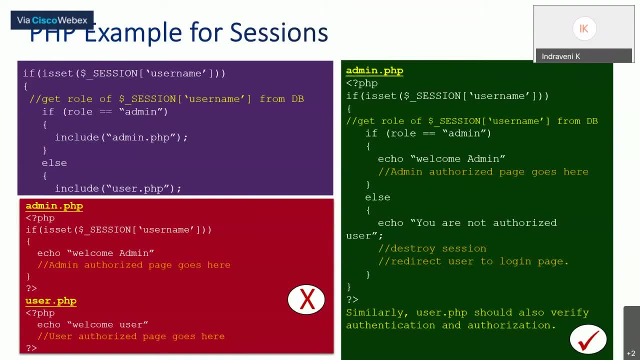 the admin page is there? what am i doing in admin page? again, i'm checking whether the session is there or not. okay, so i want to see whether an authenticated user has come on. then, as soon as he is authenticated, i'm immediately saying welcome administrator. and i'm giving the. 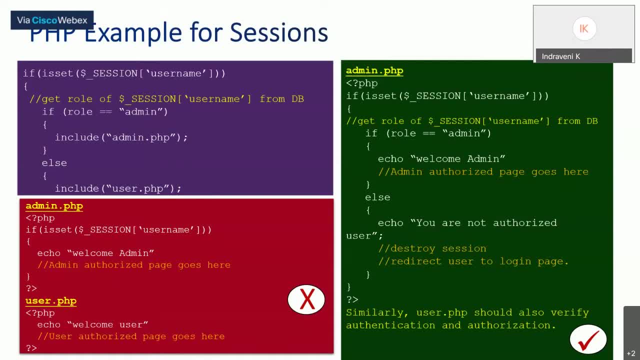 actual content related to admin. now in the user page again, he is just echoing welcoming user. if not you can. there may be also conditions for checking user session of user over now. in this scenario, when this purple and red color blocks code is available, what can happen? can you imagine if a user logged in, what happens? session is checked- his? 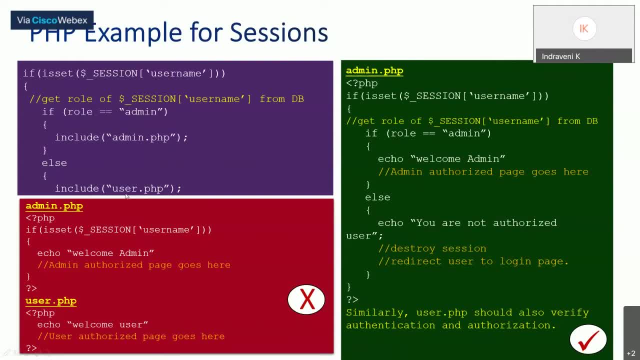 rule is not admin, then definitely the userphp page is called in userphp. he will see this code good enough. if he is a little tricky what he would do in the url there is a word userphp. he may play by changing user to adminphp or some other products. it's just a try and trial and error. 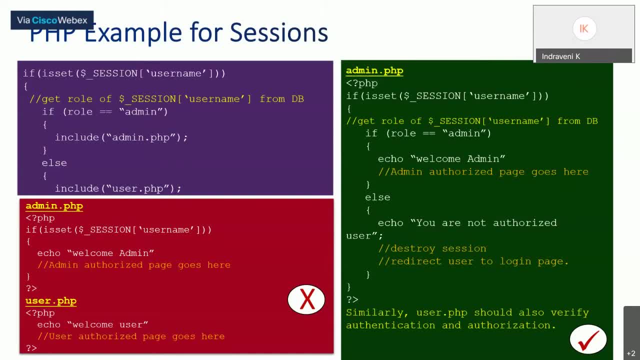 case and with the name adminphp. he will land up into this page and since he is a valid user with the valid session, in adminphp also valid session is being verified. he can see the administrator page over here. this is what is called authorization bypass: a user is logging in with the valid session and he is trying to change the url. 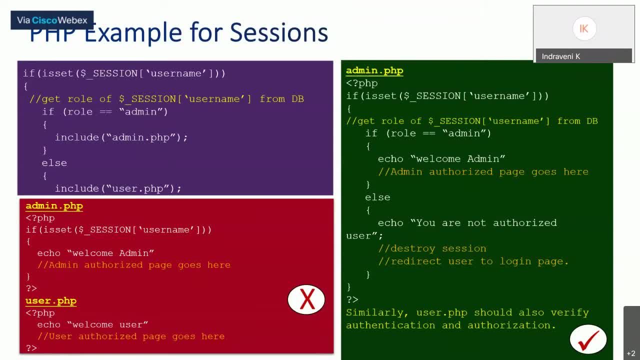 by changing the file names or something and he is able to get an access to the higher privileged user page without providing username password of higher privilege user. and this is what we have seen in most of the codes that are available in most of the applications. so what's missing over here? you can anyway see in the right side over here. 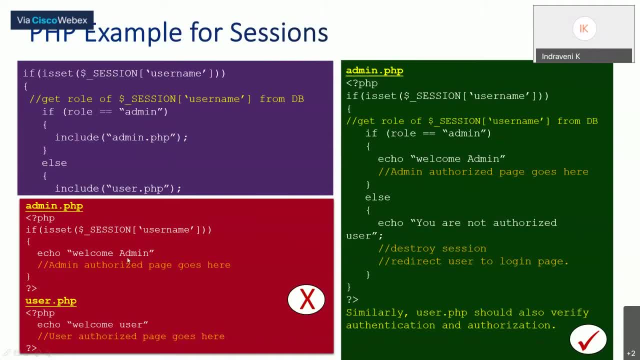 what is happening over here in the admin and user pages. they are checking the session is existing on, but again, they are not checking whether he is helping on. assuming the the reason behind this is they may be thinking: okay, someone can reach adminphp only through this main page because i'm including it over here only. but what we are forgetting is 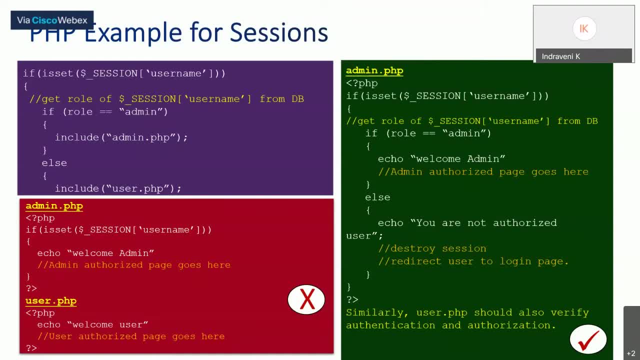 i may know the file name from the url, from the page source or somewhere. i can tamper it right. so what is the best? my admin should be something like this: what is there in right green color php? i'm? firstly, i'm checking whether my session is user or not. 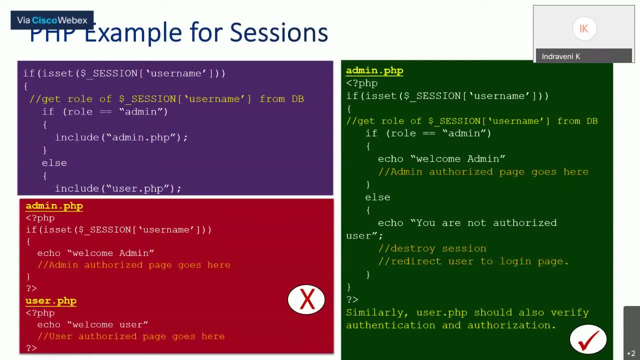 again, i'm seeing whether my role is admin or not by the database and then only give him the access. else you should say that you are not an authorized user to access this particular page because, as i'm saying repeatedly, a logged in user. we should not expect a logged in user to behave. 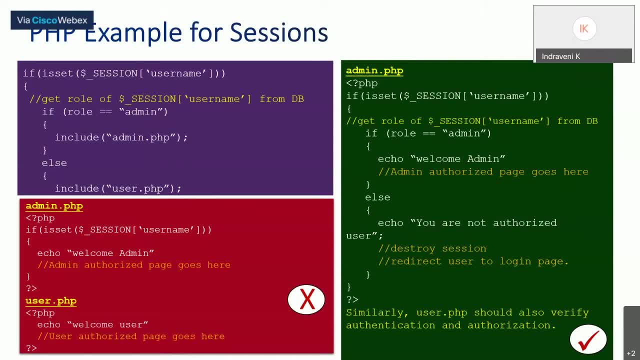 the way we want. he will behave the way he wants. so he can change the url, he can change the tamper, the parameters, whatever he wanted to change, basically. so authorization, check, verification of the role should happen in each and every page, it's not about only on the first page. he would. 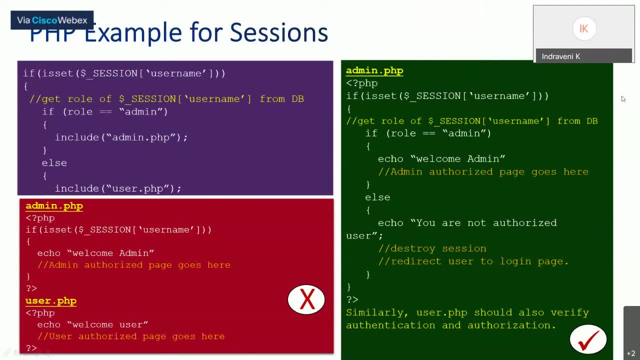 check or or on the landing pages. he will verify. every page that he is coming in has to clarify. it is something like if you go to a place where strict securities are there and all your id has been shown, say, organization itself, your id has been shown, otherwise you take your college example. 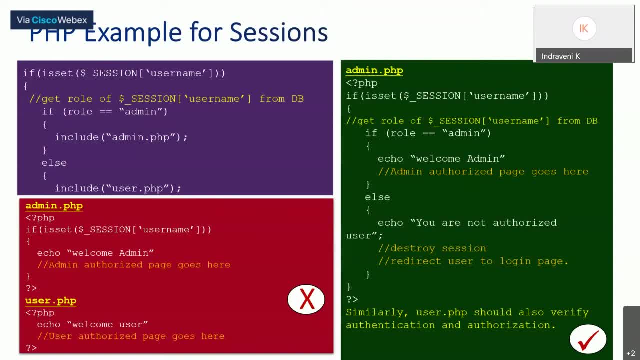 to enter into the college, you should have your id. you are a student of that college. but then, after entering, which classroom you should enter, it depends on your belonging to which year, branch and all these things right. it's not that by taking that id you go and sit in any class. 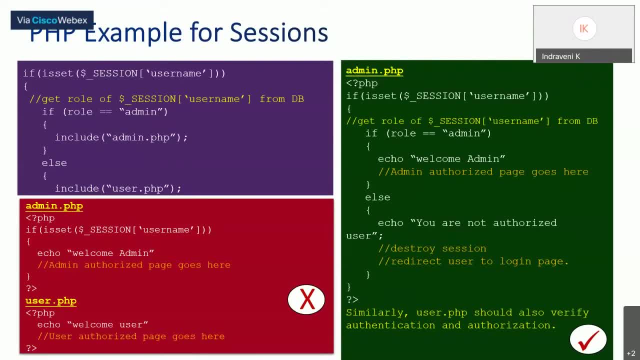 that's nothing but your authorization, so that we have to see at every class. it's not about only checking, only in at the entrance and then i'm leaving- at every entrance of the class we have to check. similarly, authorization, role based, role verification- has to be done at. 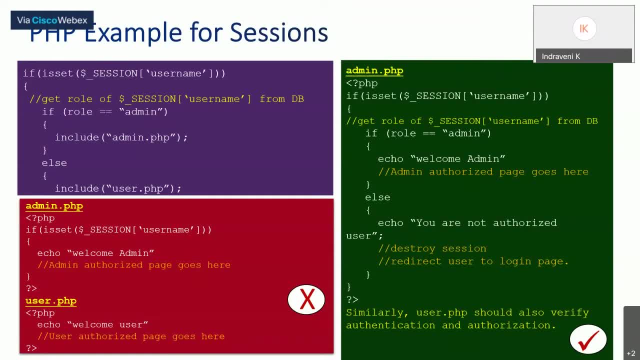 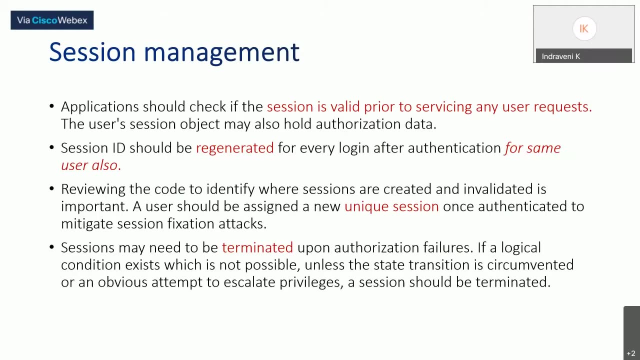 each and every page of a particular application. it's not only a one-time check over there, so i hope this has given you a picture now. so with respect to the sessions, that is, the session authorization check is most important. apart from that, how the session ids are generated. 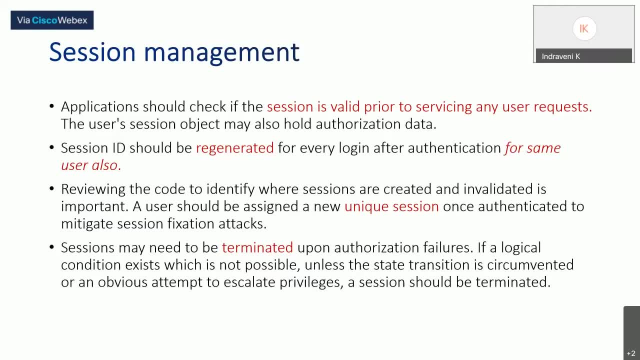 is also you should think of. you should take care about that as well. so application should check if the session is valid prior to servicing any request. this is what we saw just now in the previous example. the user's session object may also hold authorization data. so this is what we 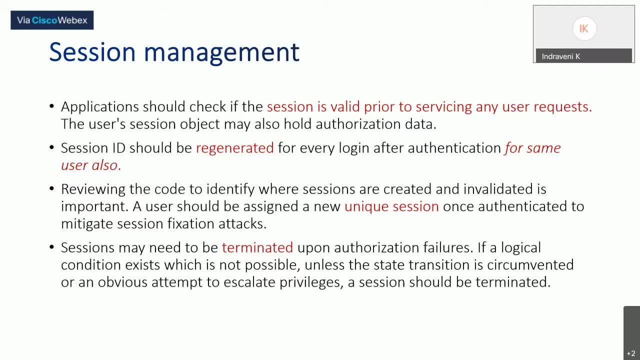 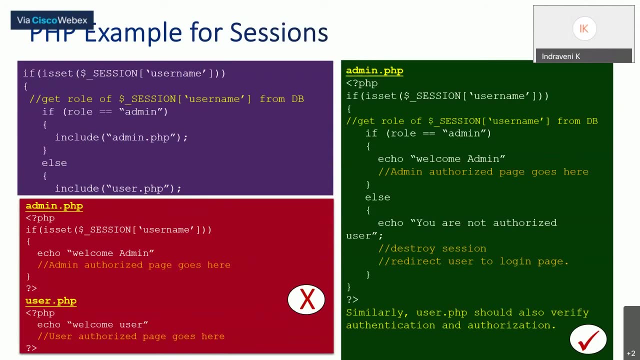 saw just now in the previous example, the user's session object may also hold authorization data sometimes, so we should consider verifying that data inside the session id itself. what does this mean? this role, what we are checking over here? we are doing a check with database. sometimes what people do is their role also. they try to assign to the session. 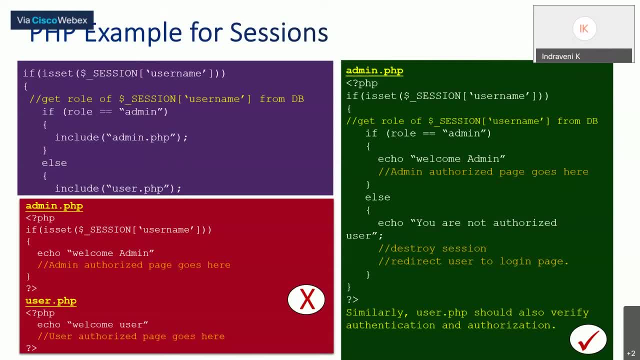 variable so that wherever the page session of username is verified, similarly session of role also can be checked in and taken a decision. so role value is also being stored in the session. that is also fine, you can do that way. or the database. if you want to reduce the database queries and all you can do it. 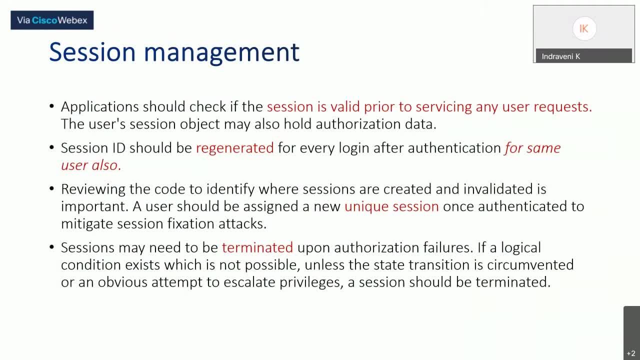 that way also. the second practice for session management is: session id should be regenerated for every login for authentication, for same user also. i know you will regenerate session id for every login, but are you regenerating for same user? please check if a particular user is logging in. 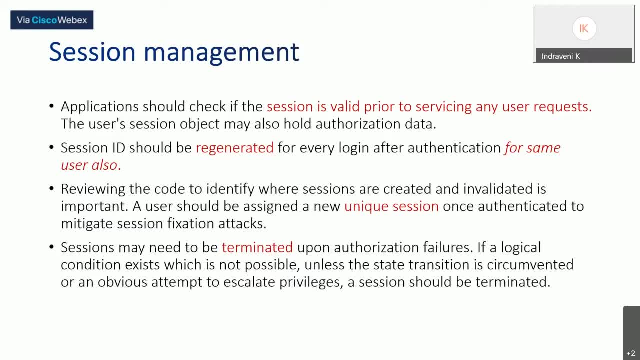 every time. you should not get the same session every time. you should get a different session. i think every time i'll click a logout re-login, i should get a different one. even i should also get the session id different before and after login as well. this also will be different, and a user should review the code to identify where sessions. 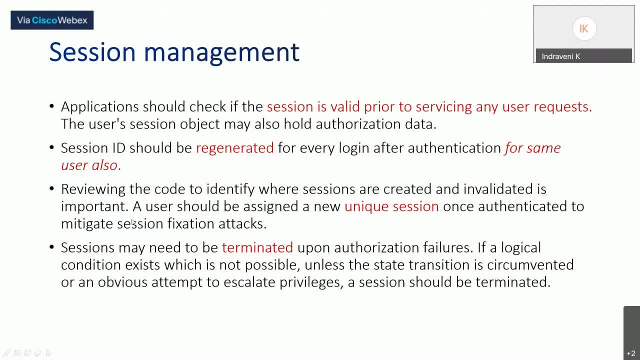 are created and inherited is also important. have you anytime seen where your session ids are stored in your web server? no, no, no, no, no, no. if not, please, you can go and check. your session id data is stored in your server in a specific folder which is actually configured on your web server: calculations, and that is a simple text. 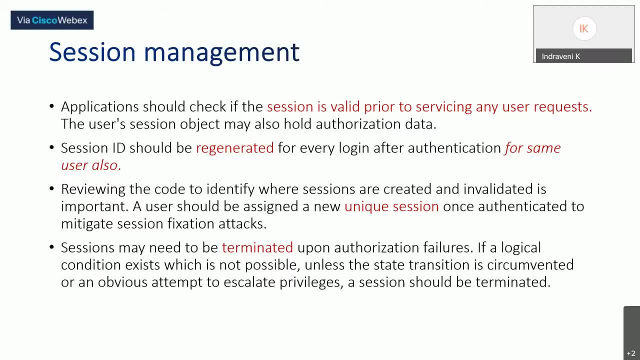 file. in case of php, it is a simple text file with that particular value. if you open the text file there, you can see the content in play. what is the session value? what is the rule value? whatever the session is storing, everything is stored in plain text in that data. so it's equally important to 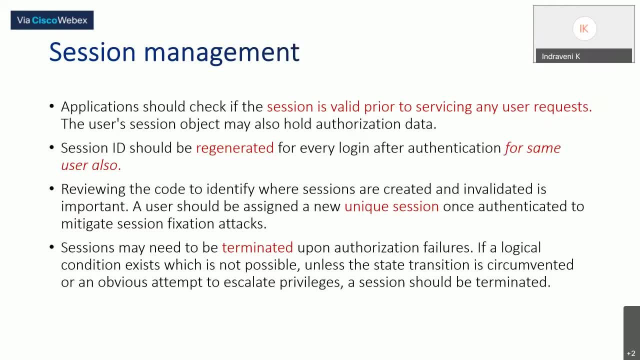 safeguard such folders, which is maintaining the session id source anyway. so a user should be assigned with a new session id once authenticated to mitigate session fixation attacks. this is what i'm saying. session fixation is something related to having the session id prior and after login as same. you should have both of them different always. so before i log in, when we first open, 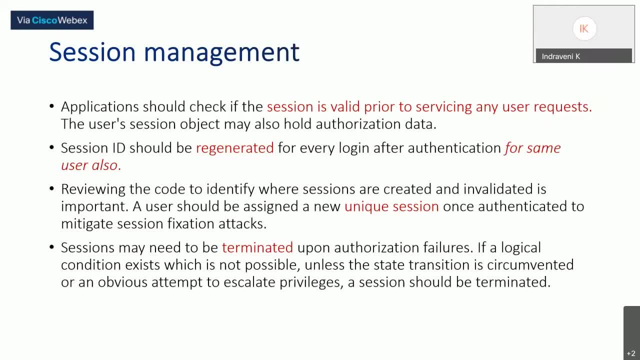 our webpage. open a program js. you defaulted. you get one session id in your browser. also you can go to cookies web developer plugin and check the cookie. you can get one. see the cookie after you log in. also you see what cookie is and what value. both are same you. 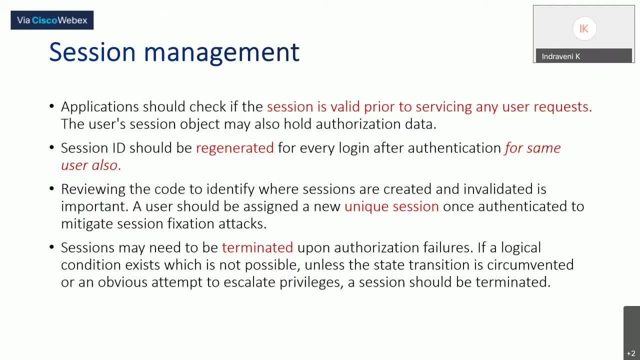 have to look into it so that you regenerate the id. it should not be same both of all the places before and after. then session should be terminated properly. session termination is also equally important. it's also equally important. many a times on logout they just close the browser, but they don't delete the session. get the server side. server side deletion. 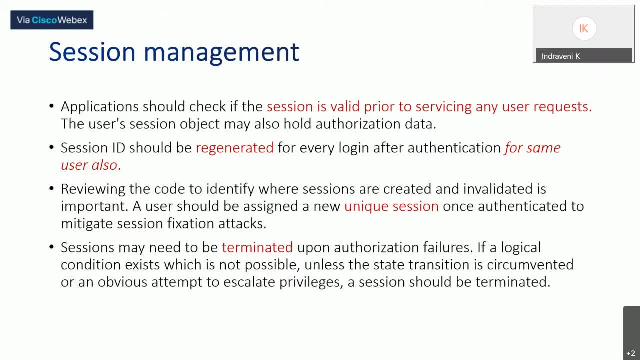 of session is important for us. it should be terminated every time that we close the system, that we log out the system and so on. so session may need to be terminated upon authorization failures if a logical condition exists, which is not possible unless the state transition is circumvented. 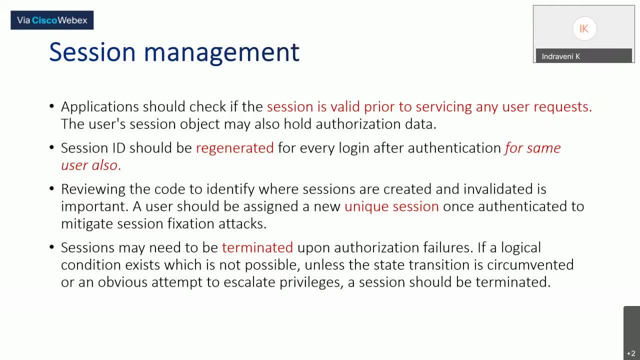 or an obvious attempt to test this session should be terminated. so it means that if someone is trying to change some values, somebody is trying to tamper a behavior on the systems, you should try to terminate that, even a valid session that is being generated on that particular browser. 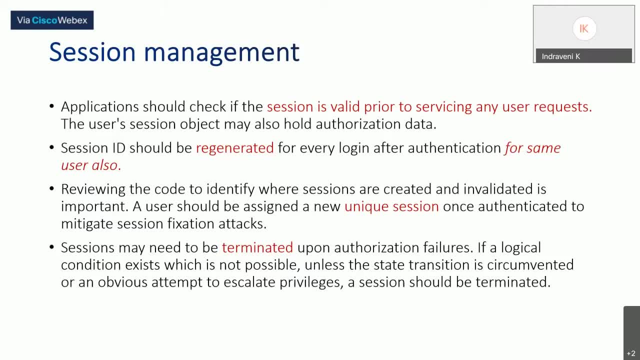 there should be some logic being written on the systems to identify the behavior of the user after the logs. it means tampering sessions and then you have to terminate them. so these are some best practices that you can have to follow for session management. so that is all about the various web attacks. 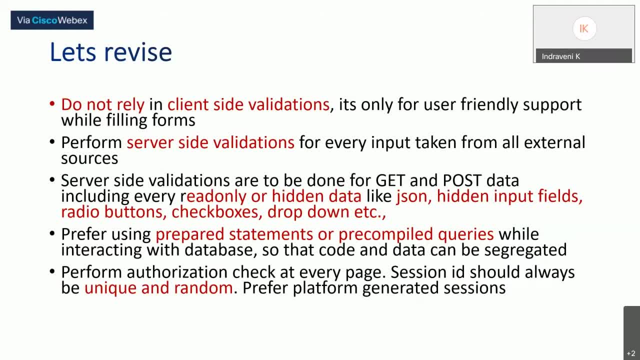 so any questions we can take up. what the points we have discussed so far is what i have just dropped it down over here. so what all points we discussed so far is something like: do not rely in clients and validations, it's only for user-friendly support while filling forms. this is what we discussed in. 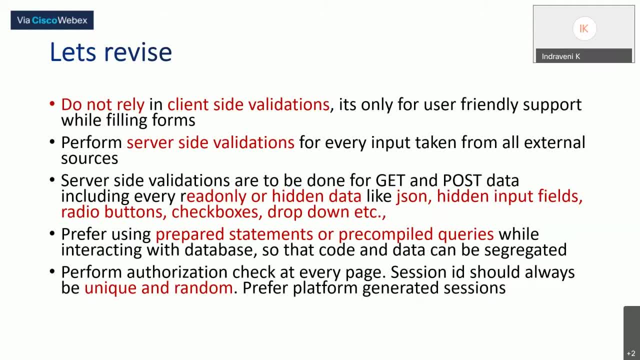 the beginning. we should not perform any kind of client-side validations. perform server-side validations for every input. perform server-side relations for every input taken from all external sources. so, whatever you take from users, every data should be validated properly, as we have seen in the data view. 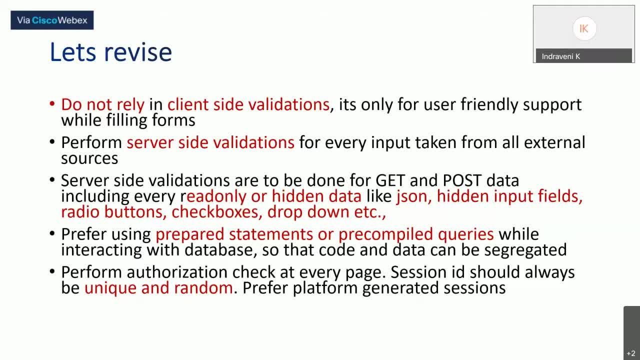 picture. we have to validate every word. then server-side validations are to be done for get and post data, including the read-only data or hidden data. also, read-only is the one which i was referring to- the drop down check boxes, radio buttons and so on- and prefer using prepared 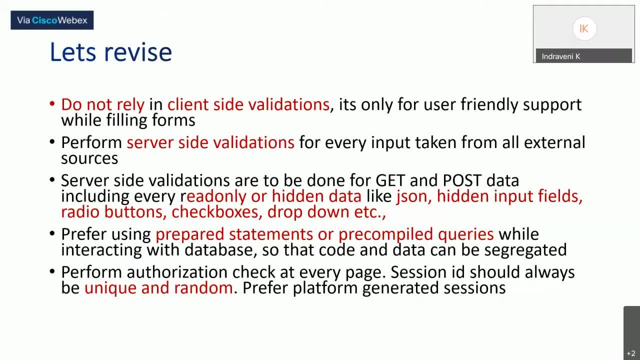 statements or pre-compiled queries while interacting with the database. this is most important and also using the least privileged user is what we should think of and perform. authorize check at every page. session id should always be unique and random. please prefer platform generated sessions always. that is php means php generated sessions we should use. we should. 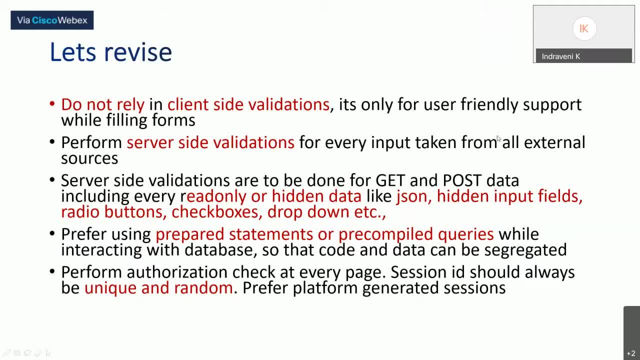 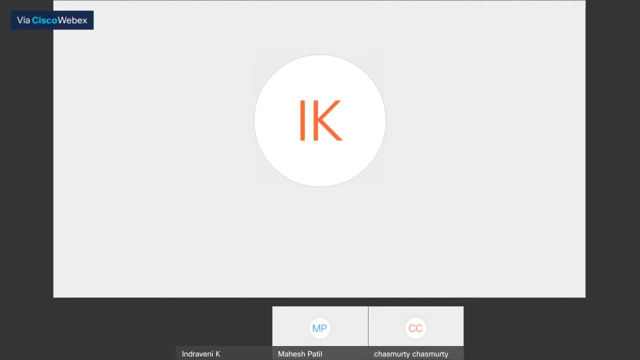 not manually or using our code. we should not try to generate the session ids. so i have some questions. in the browser, where can we find sessions? yeah, in the browser you can definitely find sessions. okay, let me show in browser. i'm just stopping screen share. i'll show my screen character. 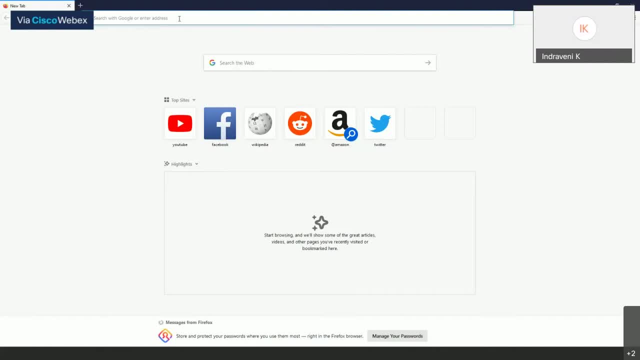 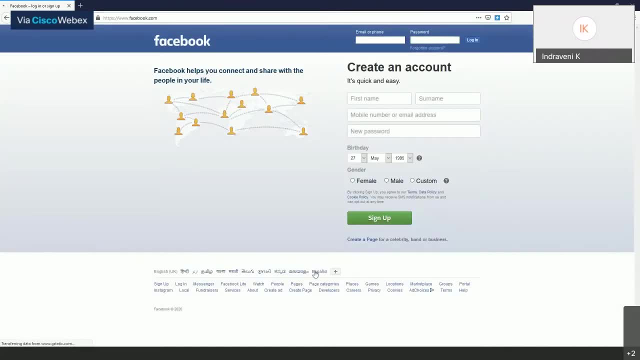 can you see my screen? this is my browser over here. i would just show you facebook only for your reference, so i'm just answering a question that has come. where can we see the sessions in a browser? as i said, any application you access, you just press f12 key, you can see. 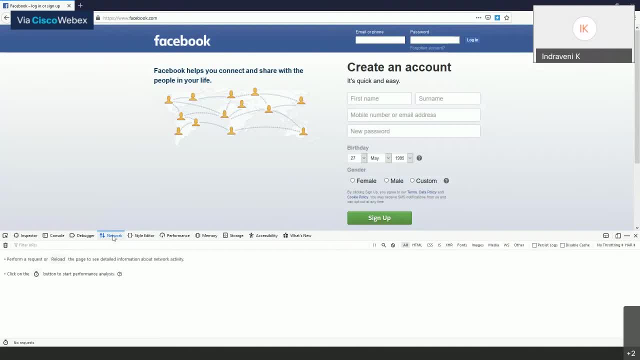 a window coming up like this. so over here you will see there is a network tab. after this window is opened up, then if you try to refresh a page you will see the link will be displayed so you can see it. you can see the link has been opened up after this window. 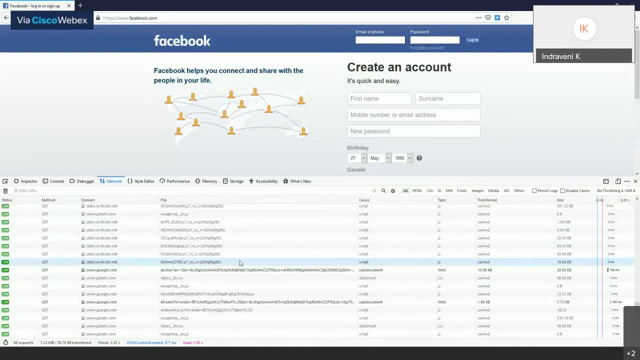 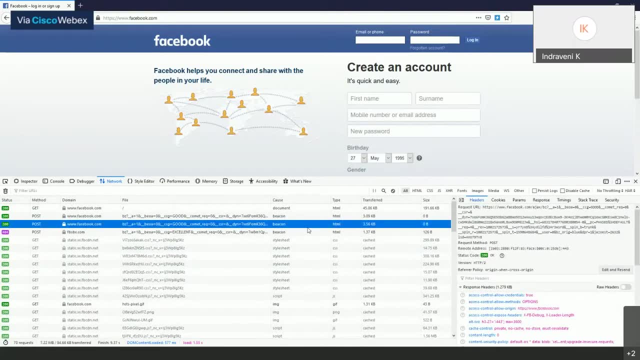 been coming up over here like this so you can see your sessions, cookies and all over here for every page by default. i just clicked on one of the link over here and in the right side you see there is a cookies headers, cookies params, response and all just go to the cookies. 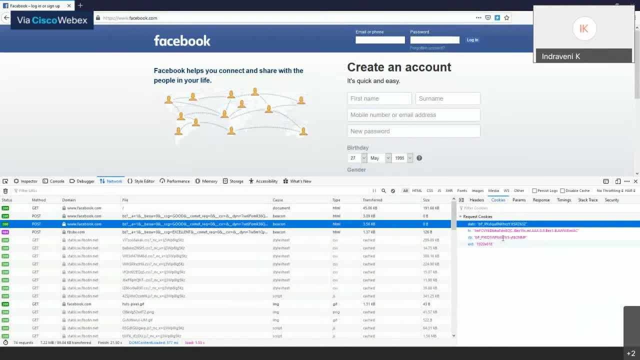 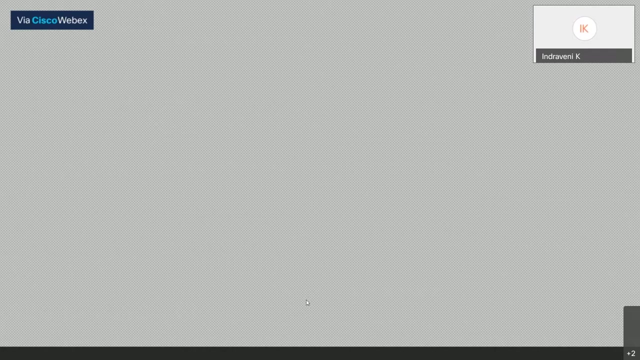 header. these are the cookies and these are nothing but the sessions, like fr session id. since i did not log in, these are the sessions that are there prior to login. this is where you can see your sessions and cookie values. so this mitigation what we have seen um. 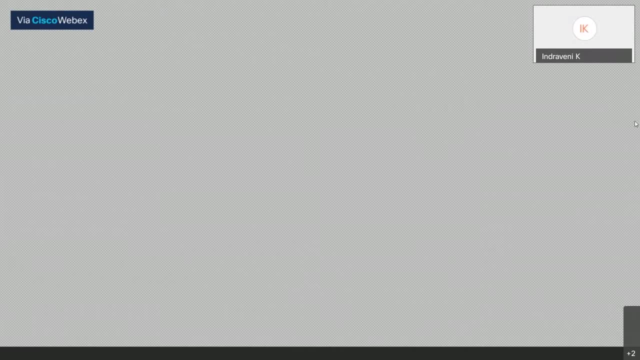 mr jonas maranga, the mitigation is applied for php. the html entities function which i have shown is for php, but you can search for your programming language. if it is java or whatever it is for that specific language. you just look for html entity encoding functions or libraries. they would be an equivalent one. what i have shown is an example of php, but 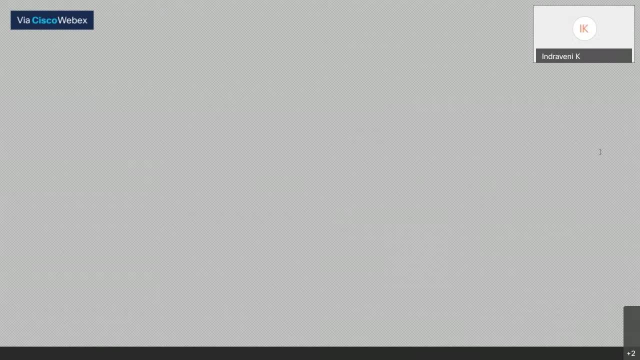 the equivalent would be there in your respective language. it could be java or jsp or so, but in its example they have been applied to all the other languages. so to start here, at point one, the data loader is working fine. you can see, here is the data loader. indeed, it is not. 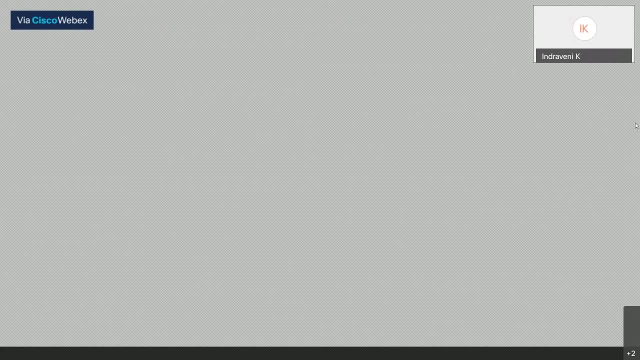 a page, one that is on therosoft website. so, to start here, it is a php data loader. it is the first one to be saved from the php package, then after that it is a new document, and one of the important things here is that it is a function called php, but you can see when 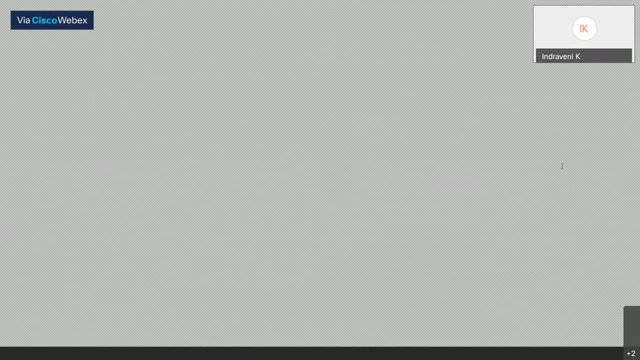 it is used here. it is used in the browser. it is not necessarily in the browser, but it is asking: blacklist or white list based validations can be written in one php code. no, i think you should use. you should use any one type either. you have to use blacklisting. 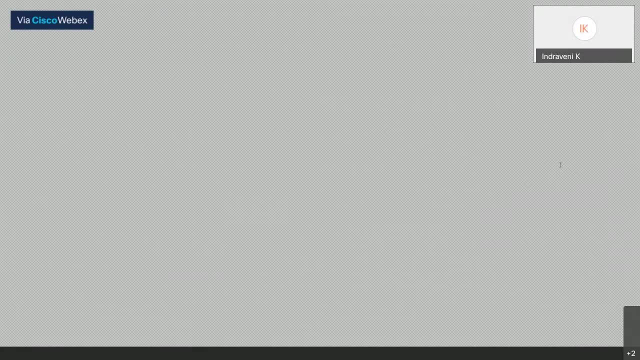 or white listing. you don't have to use both. you wanted to miss madhuri maeswaram. basically, you should try to decide upon whether your application you want to use white listing technique or backlisting to validate a particular input. you don't need to use both. but 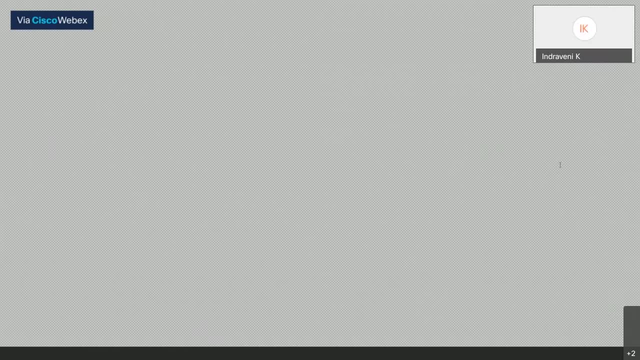 the best practice is to always prefer for a white listing technique because you can have a list- uh defined list- of parameters or characters which you know what is required for your application. so you just put a regular expression with what you require for your application and then access it right in your application. don't put both. 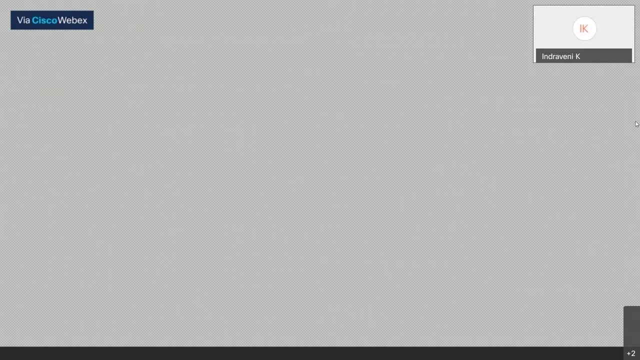 of them in one php file. so that's the best practice for your application. so that's the best practice for your application. how do we develop software for cyber security? bishop sovani um says developing software for cyber security is a very generic question. yes, can you be a little specific on what you are looking for exactly? 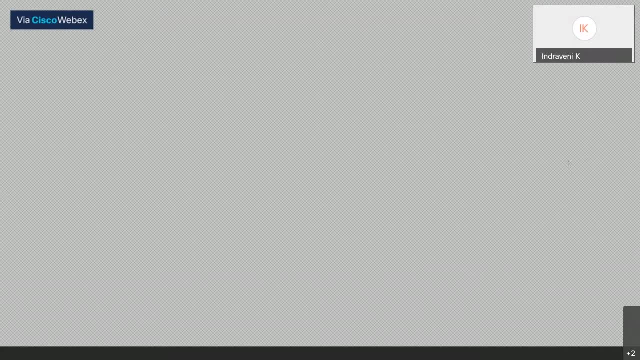 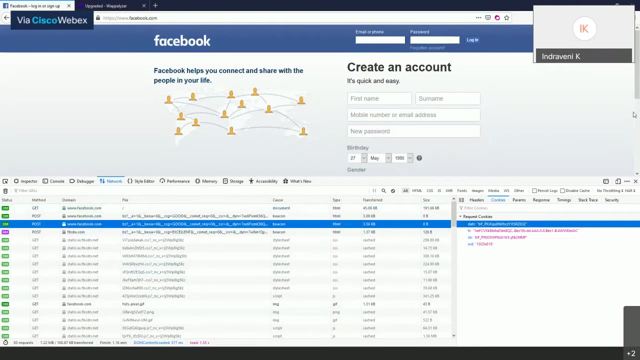 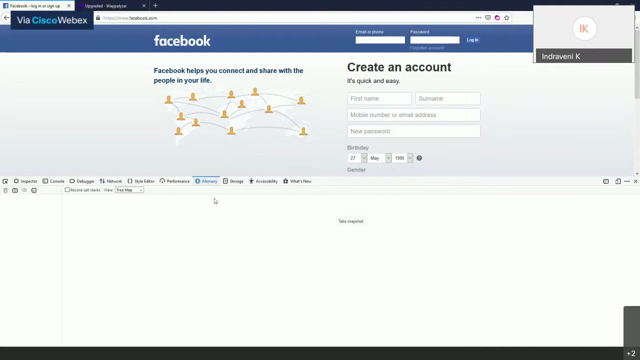 mr rishabh sovani. um, so meanwhile, i would like to show you one more point. i was referring about the local storage related content also, so in this same web developer plugin, you will have an option of memory over here. okay, so this would actually show you information about. 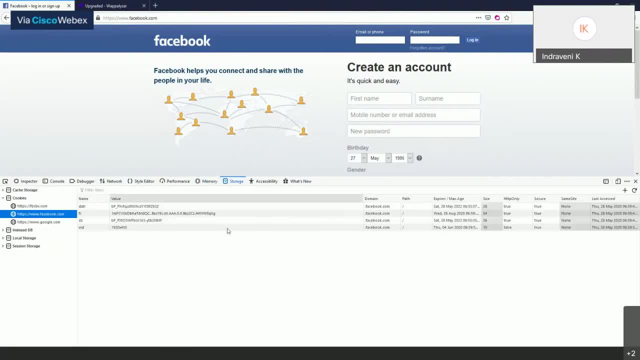 about your system browsers memory. then you also have a storage tab wherein you can see local storage and on. nowadays, all these html5 based applications are trying to store their informations on this sessions. their local storage and on some local data can be visible over here. okay, so whatever you store in local storage is also accessible to the users. so 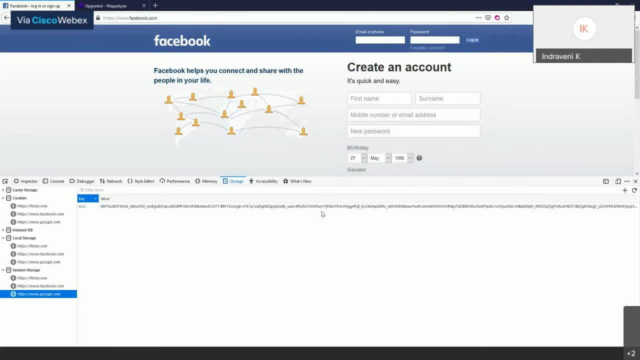 sensitive information should not be stored on the local storage as well. see, security is not python, php. every programming language is having its own security practices, security libraries. what we should know is the right way of implementing those are using those libraries. dmz in web application architecture is nothing but the demilitarized zone. it's basically a network. 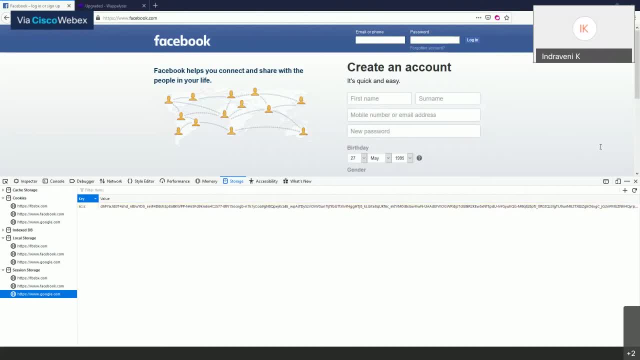 in a data center, wherever we host a website. generally, when we develop an application, we host it on a server. no, so that server is usually placed in a dmz environment. it means that that server is protected with a firewall, with a router, with an ids- ids- and it would have a different network than the organization's network. 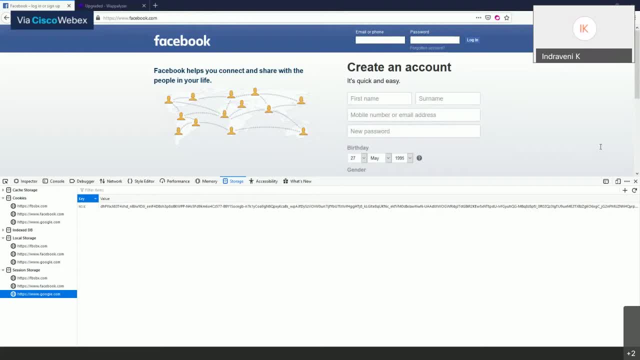 so that it is not. it is a secured separate zone. that is what is the dmz name, miss madhuri. once again, yeah sure, white listing and blacklisting means what risha wanted to understand: white listing and blacklisting. so i just go back to the same slide. 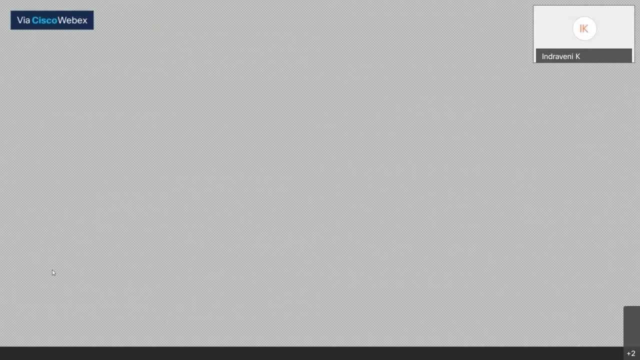 see white listing and blacklisting is something that on what logic you are trying to accept your applications isau's�. so white listing, black listing is something related to on on what um thought of characters again is what set of characters you will be validating your variable. so over here. 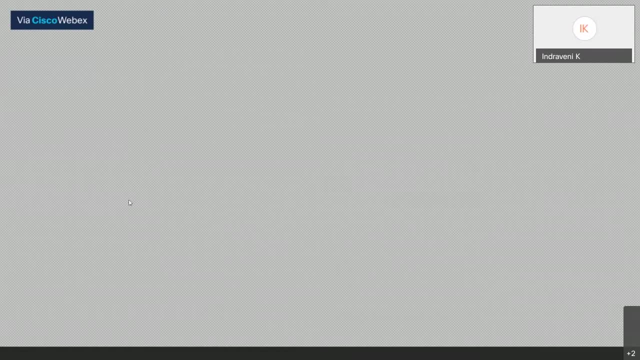 you have a variable called fname which i am taking from a form input field. okay, this fname, when i am taking from my browser, i mean i means when the application is reading from the browser, it's an input that is coming from browser to the server. so when an input is coming from browser to server, 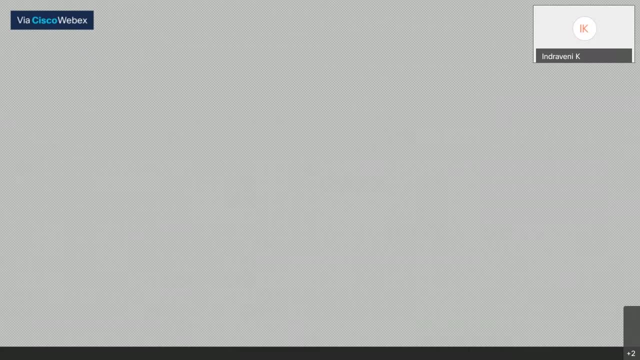 it is important for us to see that it is the right, correct input. so we have to do validation. so what we are doing in registerphp: we are trying to read this post, variable fname, into a variable called fname. i am storing here, and then we are trying to put a very regular 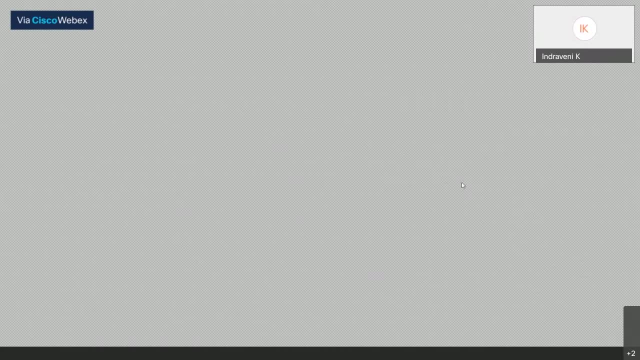 expression. this is a php regular expression with certain special characters being added over here. the condition over here, what we are seeing here, is if the dollar fname variable is having any of these, then this: if condition: do not process it, else process it. this is called whitelisting. i am saying: if any of these, why i am saying blacklisting is these are the blacklisted. 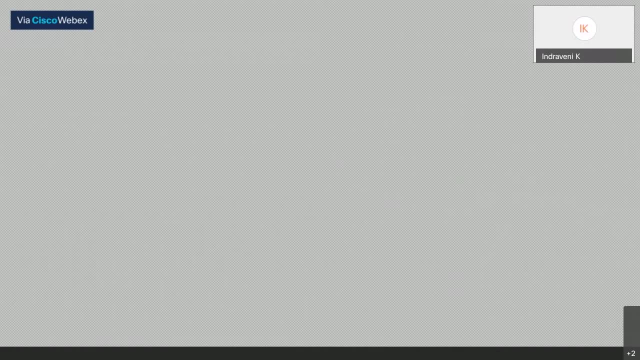 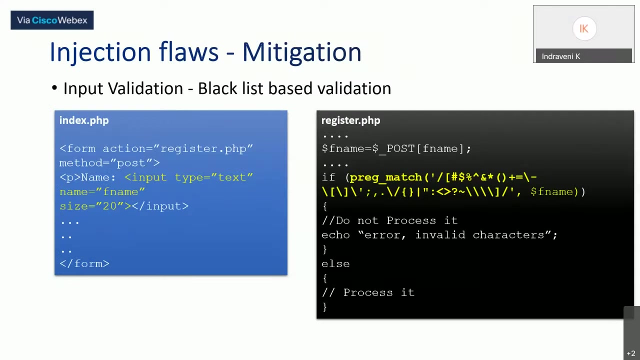 characters. these characters should not be there as part of my variable. that is why it is a blacklisting if i want to say that these characters are needed in my my uh screen. can you see now? yeah, okay, so if regular the post variable fname. i am trying to verify. 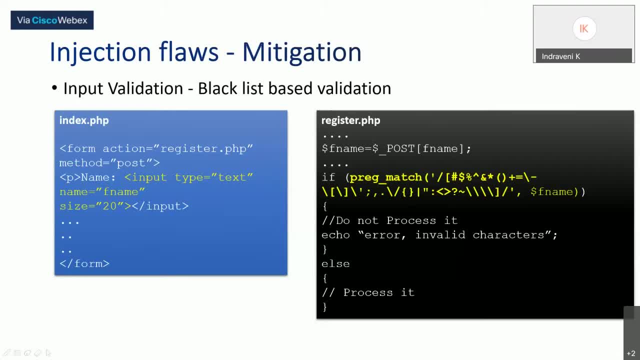 with the set of characters, whatever you are seeing over here, uh. so here you can see that these are the characters, these are the special characters. single quote: uh, square bracket, hash dollar semicolon. all of these are the special characters which i am saying, that i don't want these characters to be part of my dollar fname variable. 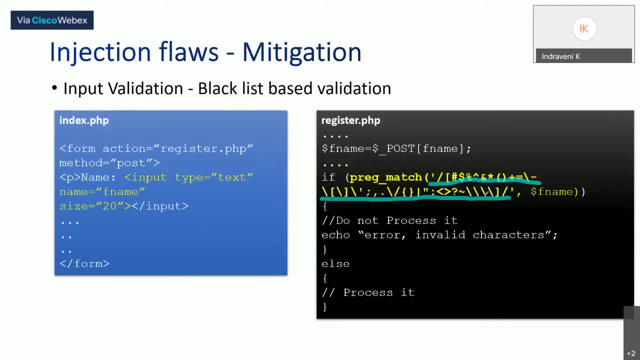 when i'm saying i don't want these characters, these are all blacklisted. i don't want them, so they are blacklisted. so if you're writing your code to put to compare your variable with a blacklisted set of characters, that is called as a blacklist based validation. 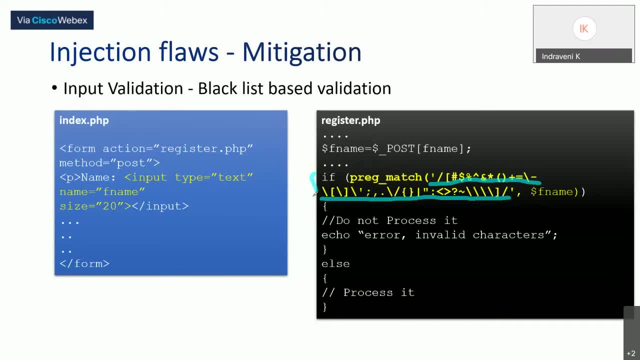 you're trying to choose a validation technique, this one, which this entire validation technique, whateverнали validation- is there. you're trying to utilize this entire technique, uh, in a way of by creating a list of blacklisted variables and then seeing whether any of these things are there in that variable or not. this is gone. 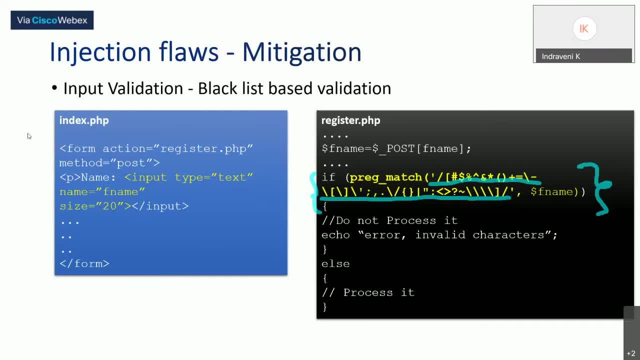 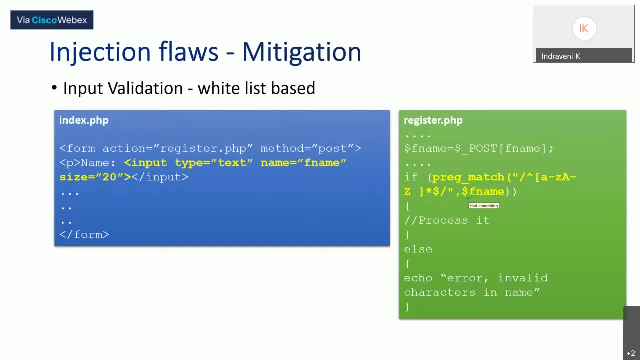 is a blacklisting whereas the white listing technique. in this, what is happening? we are trying to create a set of variable. these are the a to z, capital x and small a to z and a space. i am i know that in my name field i will have only alphabets, and we also put 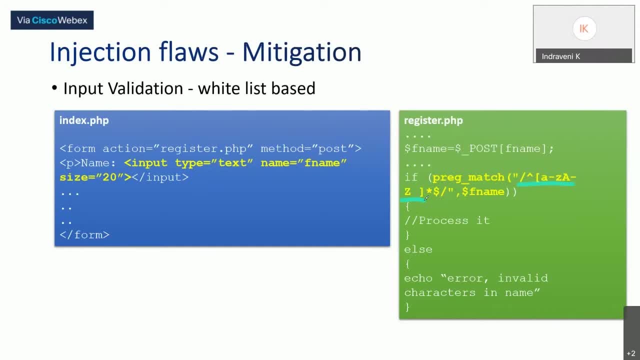 space. say, if i want to type my name, i will type k space, indra, space painting. so it's a combination of alphabets and spaces. i don't expect a name to have some special characters. in a worst case we also use a dot, so you can also put dot in this, because if you want to, 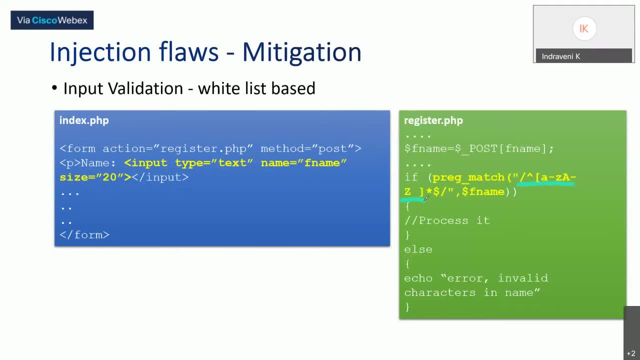 accept. in your application you wanted to accept a dot also in the name field. you can also put dot over here. so you can also put dot over here. so you can also put dot over here. so we are clear what we want in our variable. so you will use a regular expression with: 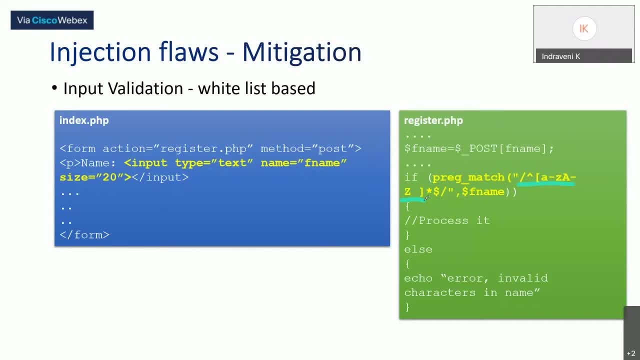 what you need. only, instead of saying what you don't need, what you need you are putting over here in the set of. in the regular expression this is called as a white list. what all characters i want is an array of white listed characters. so i am checking my variable with what i want. 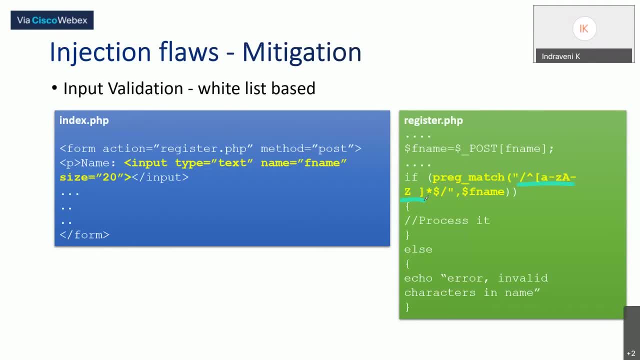 only that is called as a white list based validation. in the previous case i am checking for what i do not want. that is followed by a white list based validation, and then i am checking my variable with what i am checking my other character. this is also a regular. 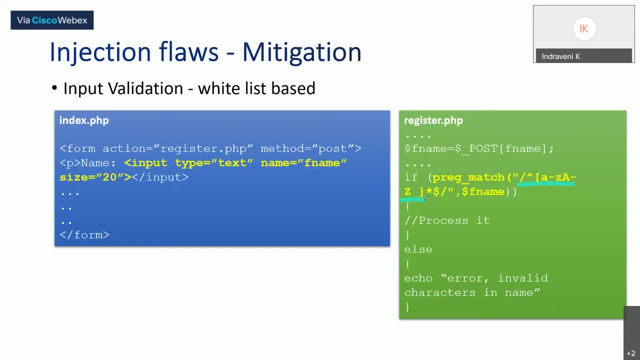 expression. so i am checking my variable with what i want. basically, i am checking my variable by saying what you want. anything else is in the same direction here. this is also a regular expression. now, what we are going to convey over here is a blacklisted variable. that is called as a blacklisted variations. now, when we are comparing this, we are trying to choose that white listing approach is best because what we want we know very clearly and that is usually a smaller list when compared to what we don't want. that is the reason we. 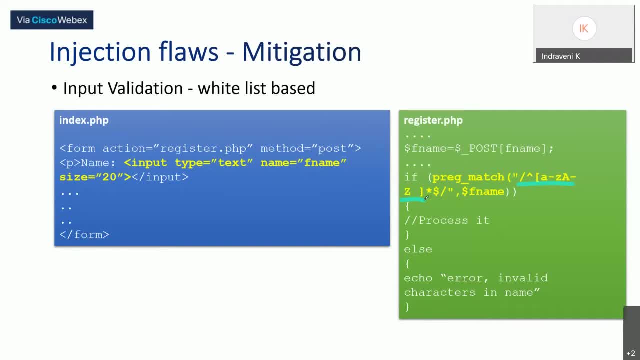 Post method is more secure than Smadri, secure than gate method, and the data within the post method is tampered. Yes, Smadri, the data within the post method is also tamperable. That is what we are trying to show over here in my previous slides. 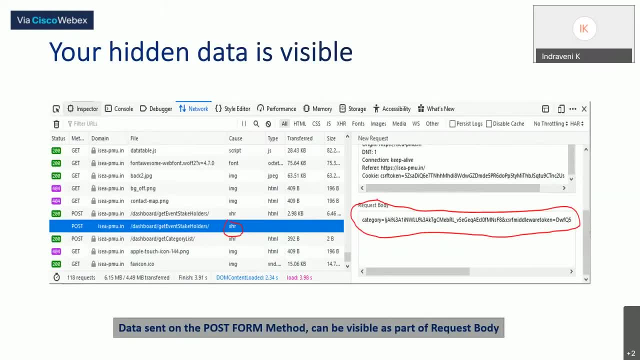 See, if you see this screen, this is how this is a post method in the left side. This what you are seeing over here. this is a post method request In this particular page to this particular get even stakeholders- page. this data is going: 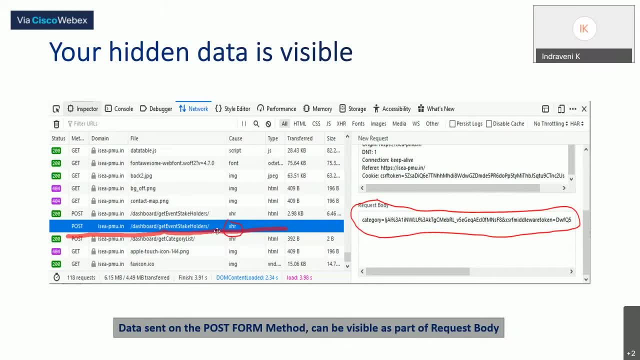 in a post method. It's not part of the URL. See: these values are not there after this stakeholder part. If it is a get parameter, then what you will see. you will see it at the, something like this: See, this is what you see in a get value. 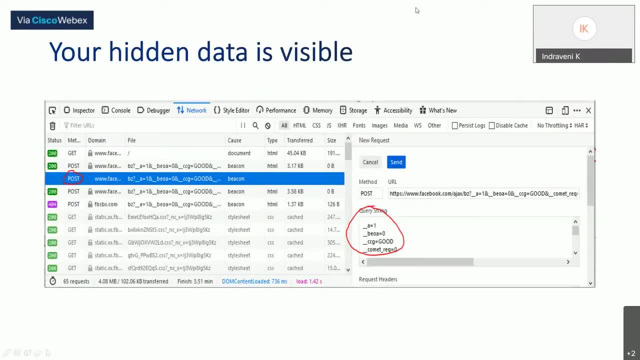 Whatever you are seeing over here- question mark, all these values are get parameters, isn't it? These are very visible in a URL. So what you see in the question mark, all these values are get parameters, isn't it? And then the next thing in the query string over here is also get only. 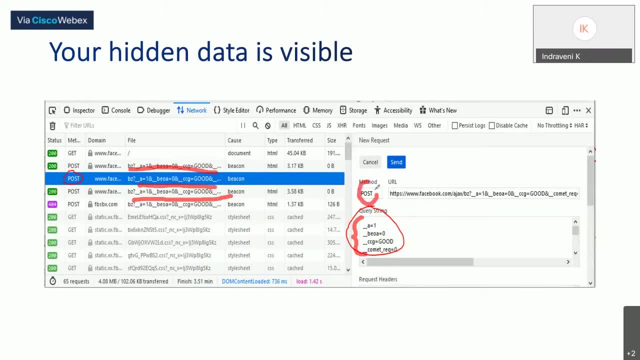 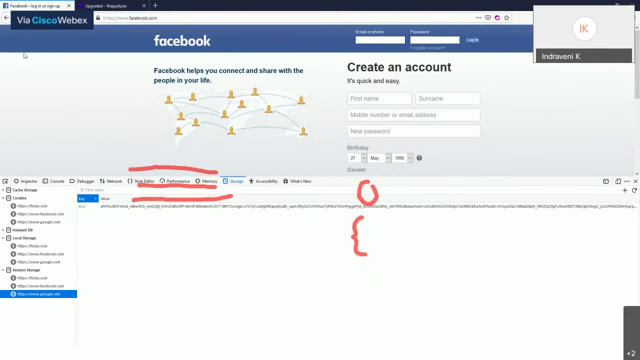 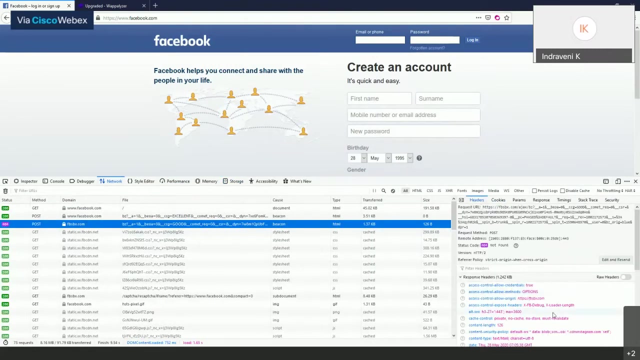 But the same method since it is post over here. if you just scroll this page down, usually you will see someone post method over here. I'm just refreshing my this one Facebook page network tab. can you see my web developer page here? 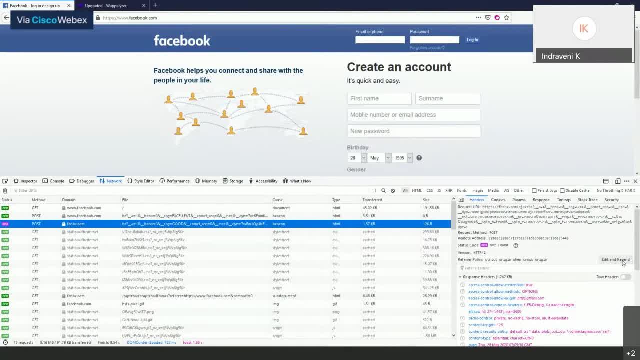 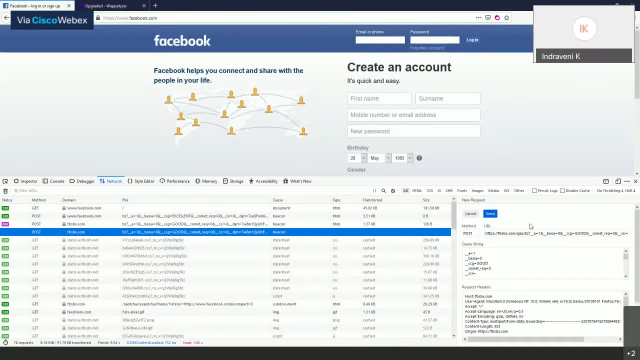 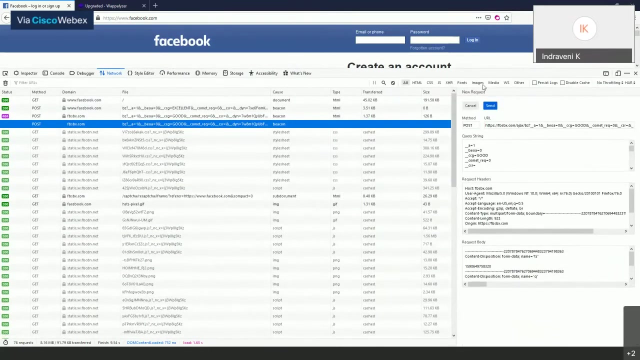 So you can see the same here. So PHP validation is server-side validation, basically. So this is the post method data that you are seeing here. See, this is the query string. this is the request header. If I scroll down, this is the. I will just move this screen up, This body, whatever you. 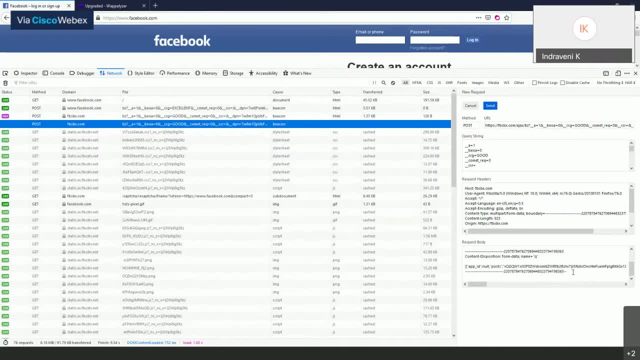 are seeing over here. this is all the part of the post data. So all this data- this Madhuri was asking a question post is secured than get In what sense it is secured? It is secured only in the sense that it is not part of the URL, like this General URL will. 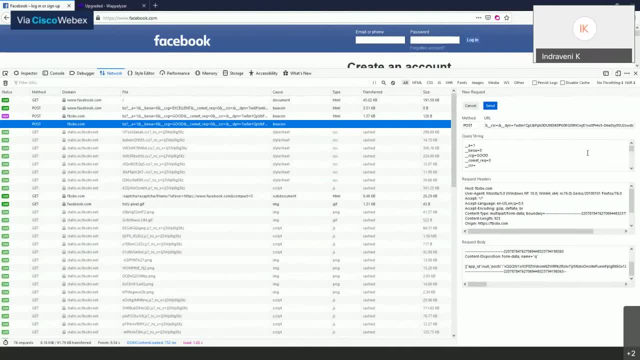 have all of this content, But in post all of this would not be part of URL. There is some more content which is going without part of the URL, So post method data is visible over here and we can also tamper this, As you can see here. this is where this is where. 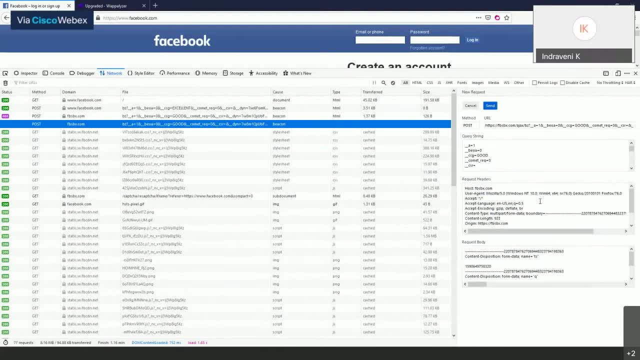 I am using this plugin. I just click on edit and send And now over here I can come here, enter any value, name value, any of these values. I can enter some garbage value, anything I want, and then say send. This data will be sent to the server, with whatever I have tampered. 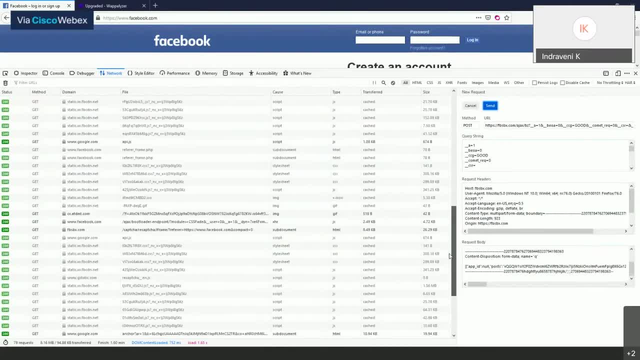 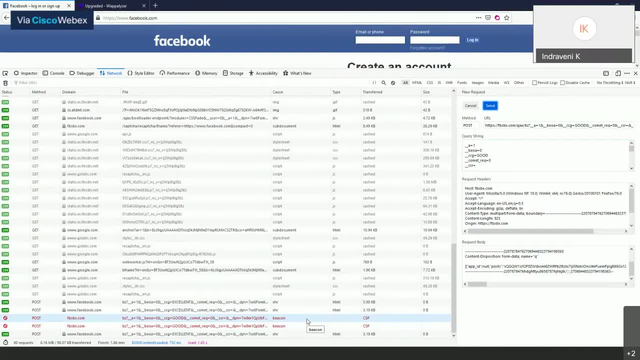 That may show me an error. It depends on that. That sent data. you can see in the last- And you see there is an error coming up here. Content security policy is stopping me, So I am going to delete this. But post data can also be edited. It is not like post data. 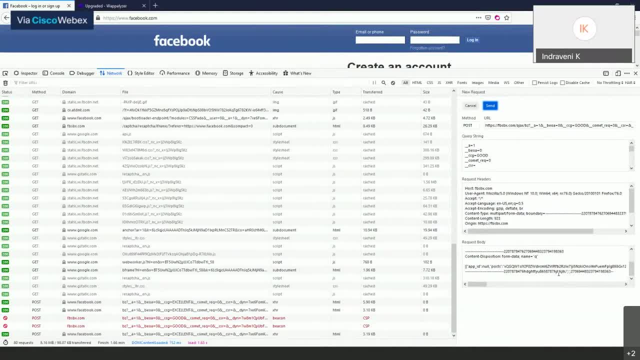 is secured Post data also, you have to do complete validation, So you should not put sensitive information on the post data and all these things. Okay, is it, Madhuri? is it clear to you? Yes, the best method is to validate every input at the server side only. 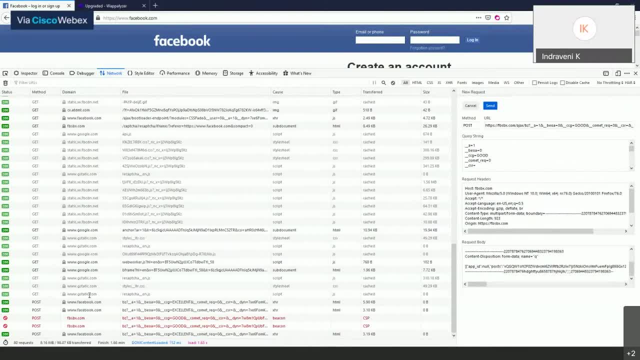 PHP validation. what we are doing is a server side validation. So what we are doing is a server side validation. As I said, PHP, Python, Java, Ruby, all these programming languages, all the frameworks that people use- all of them are server side programmers. So whatever. 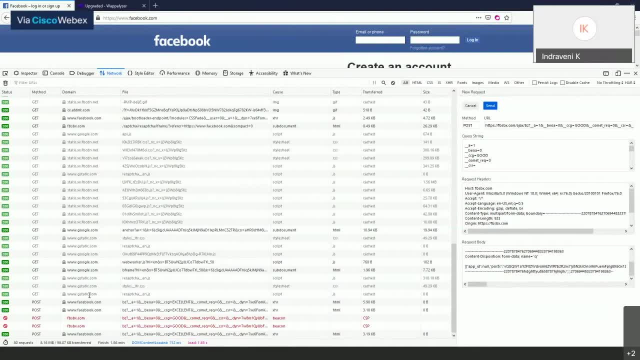 validations you write as part of that particular code, it is a server side validation. If you are writing any logic, any validation using JavaScript or using HTML5, that is a client side validation. So those can easily be tampered or bypassed. It won't stop from entering special. 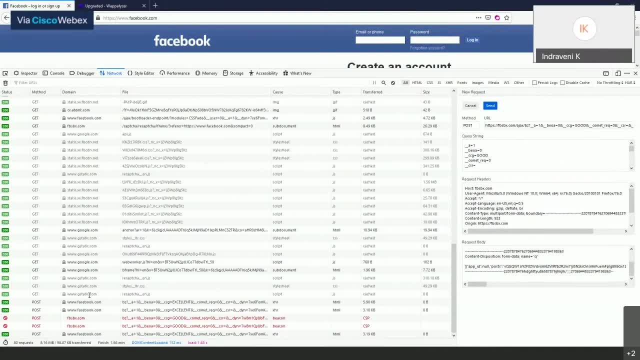 code. Is there a way to do MP5 or other encryption at the client end before it is set? Yeah, MP5 hashing you can do. encryption also you can do at the client side. There is a JavaScript plugin library called as jcryptor. You can use that to do encryption of the content in. 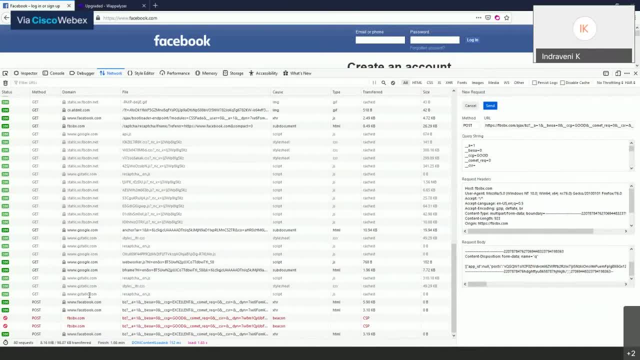 the client side and send it. But the only thing is that the key for the jcryptor decryption key you should maintain at the server. So that is the key for the jcryptor. So that is the key for the jcryptor. So that is the key for the jcryptor. So that is the key. 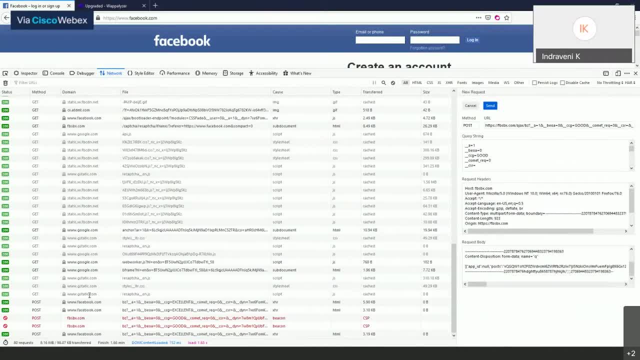 for the ccpt. So that is the key for the ccpt. So that is how you can decrypt the content In server. only you can decrypt the content. I mean encryption happens at the browser. but even an encryption key should not be used for decryption. That is how you. 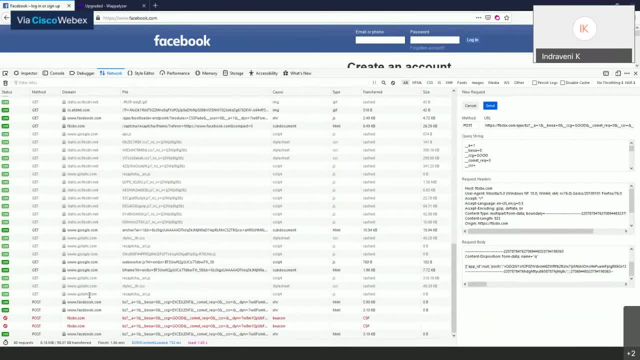 should plan the application and use the jcryptor plugin. That you can do. Mr Nihal Nihal has asked a question about this: How to de-hash password. De-hash password- See, hashing is a technique where you can decrypt a password in a jcryptor. So let's try that. Let's. 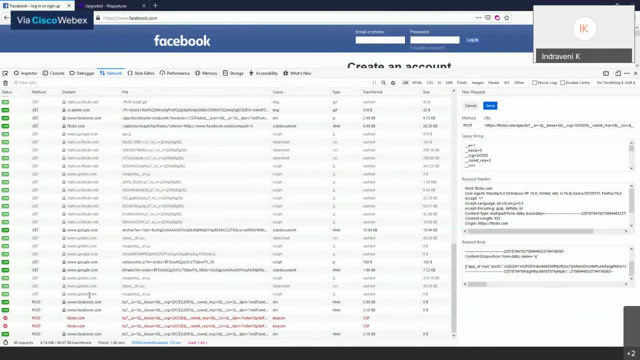 technique where you can do one time, one way. only thing is you can get same hash value for a given code, but hash cannot be dehashed. hash can be generated and compared to ensure this is the correct one. Mr Manikant, what I am saying is say, for example, you have a 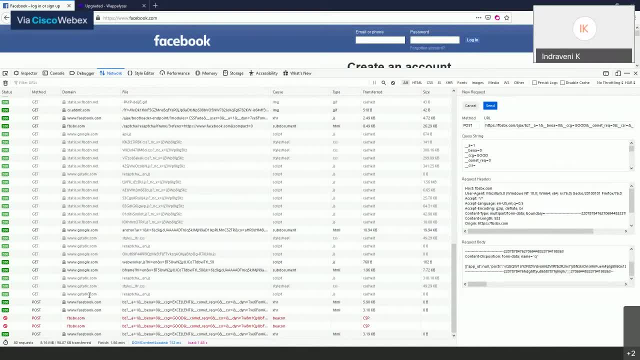 string called as cdac. the hash for cdac is: may be one, two, three, four. if you want to decode or dehash or unhash this one, two, three, four, you cannot do. but you can use the same hash algorithm and create a set of values and generate hashes. then you should see which among these. 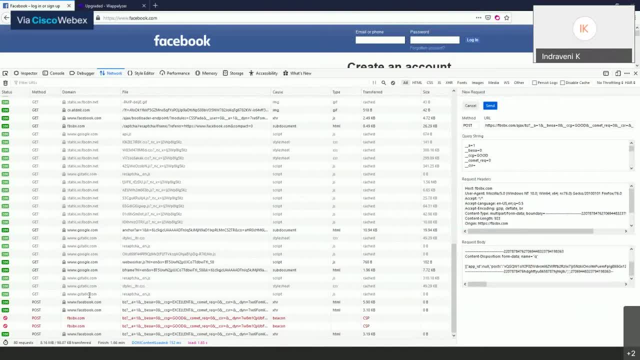 values is having the hash result at one, two, three, four. if it is matching, then that is the original value of this hash. so you have to, but you cannot dehash the or unhash the value. hash is a one cannot. first of all, it is not possible. you can generate the hash. 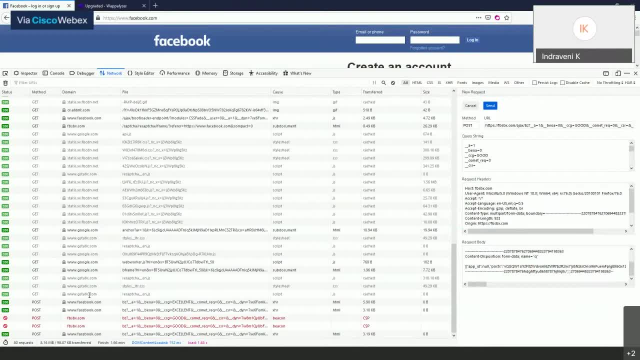 value and then you can generate the hash value and then you can generate the hash value. So if you create multiple hashes, for plaintext compare with whatever hash you have. if both are hashes are same, then you can confirm that. okay, this is the original value, provided you. 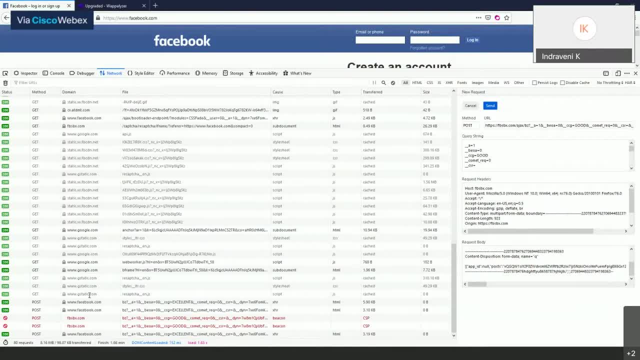 use the same hashing algorithm every time. got it Manikant? okay, if you keep encryption at the server? no, I didn't get your question, Jonas. see, whatever you are keeping encryption at the server, said attackers can't touch that through the regular means, if there are some. 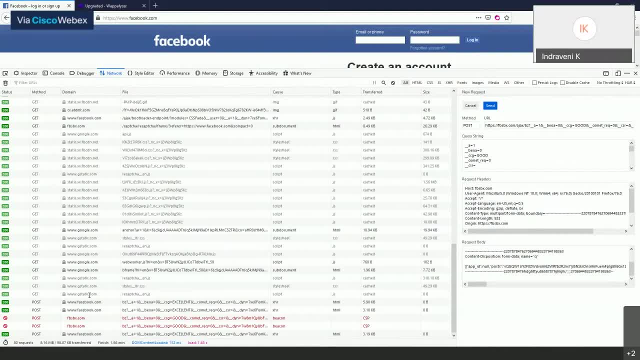 other attacks if they are accessing server that they can access. but through your web application it depends on what, which key you are using, what encryption you are using. all this depends on your logics. Okay, so this is an assignment. I think that's for assignment. also, is a procedure been already. 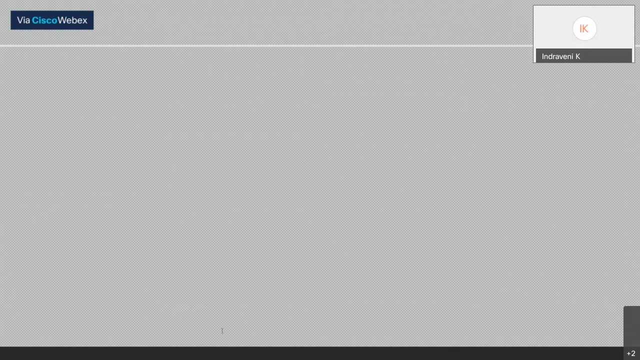 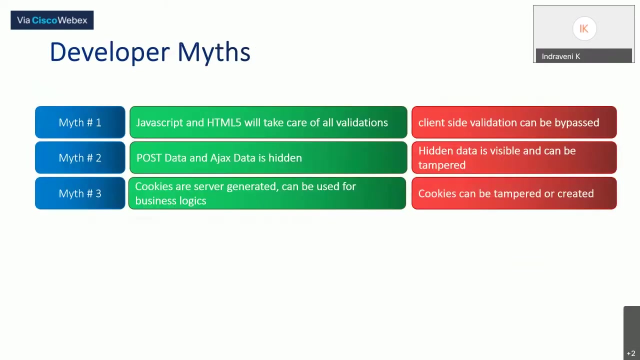 informed. I have given a very simple assignment But only challenge for you will be that you implement a secure, you develop a secure application. that is the challenge for you. So your assignment you may submit to us so that we do reverse testing on the system, whether 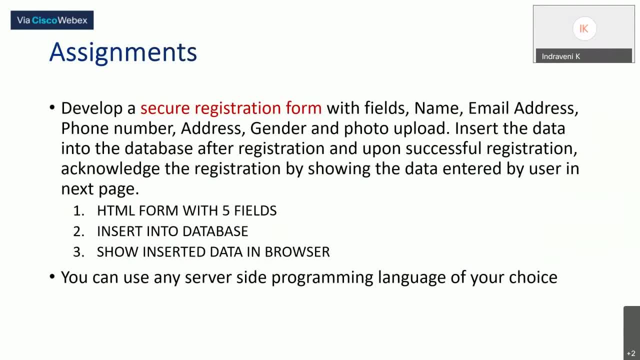 we can break the coding whatever you have. This is the assignment. you need to develop a secure registration form with the following fields, In which case you need to create a secure registration form. Whichever language you want- you can do PHP, Java, whatever is your choice. 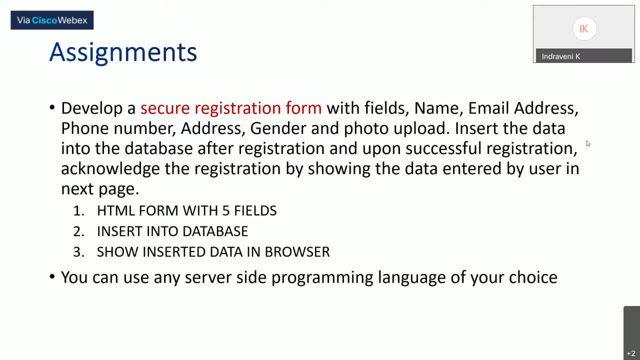 I'm not giving a language choice. I think the instructions on how to submit assignments will be given to you. will be myself will tell you after some time. Yeah, those details will be sent to me, So you'll have to develop a simple registration form with these fields. 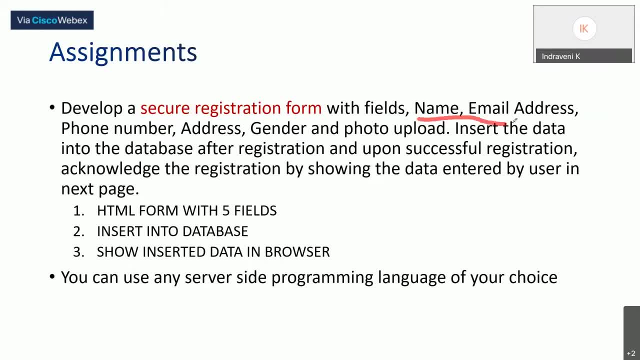 I have given you the field names also Name email address password. You will have to develop a simple registration form with these fields. I have given you the field names also: Name email phone number. Name email phone number. 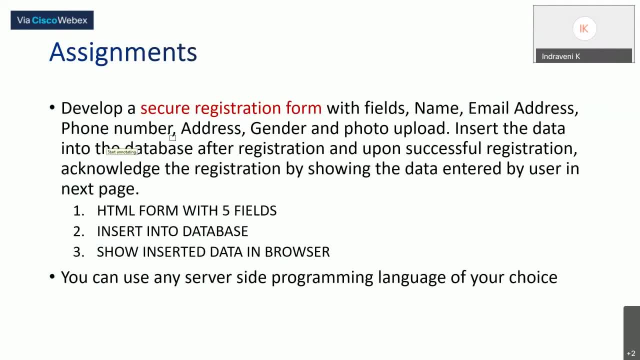 Address, gender and code. top look. These are the fields which you have to prepare for form. Once you prepare a form with these fields, you should insert the content into the databases, These values. After that you should show on the second page. 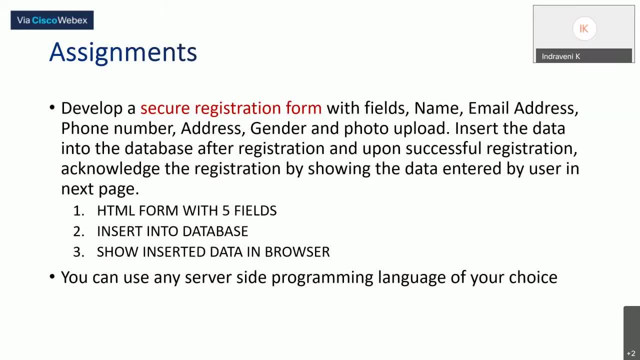 Say thank you for writing this work, thank you for your registration. you have entered the following details and whatever fields they have entered over here, six fields. they have entered all those six fields. you have to show me on the second page this two pages application. you should develop and send it so when you're